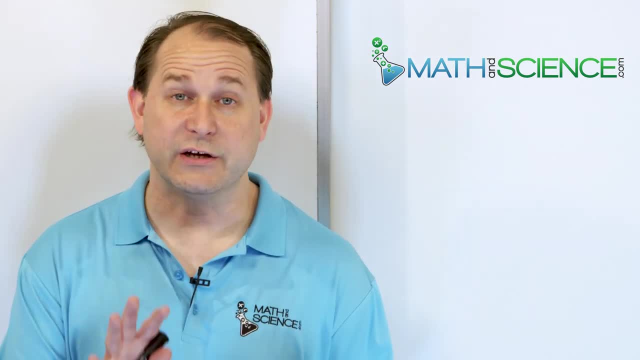 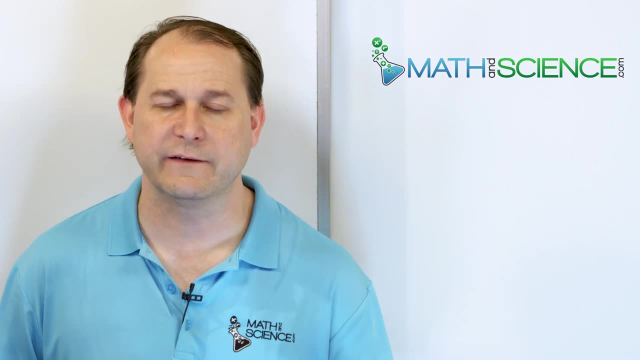 functions, because really there are six trig functions in all. But the good news is you don't have to memorize too many things, because really the fundamental trig functions are the sine and the cosine functions. Everything else, all of these other trig functions, come from sine and 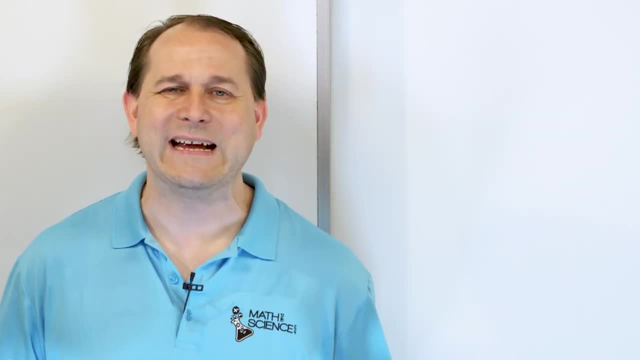 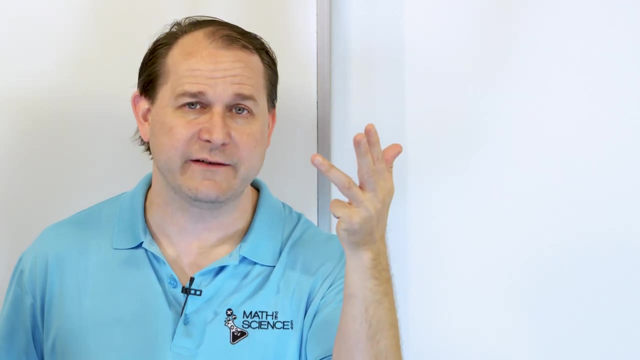 cosine. So verbally I'll just go through it with you here before we write anything down: We have sine, we have cosine, we also have tangent. Then we have to define something called cotangent, then secant and then cosecant. So sine cosine. 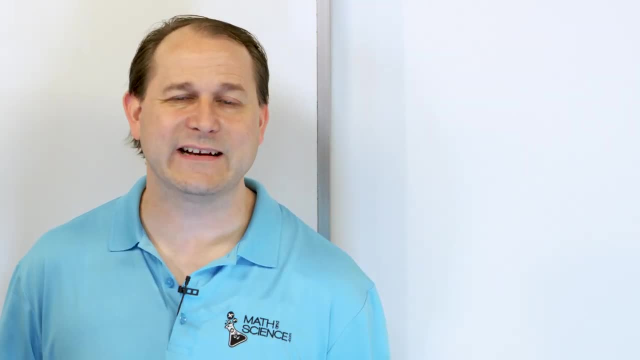 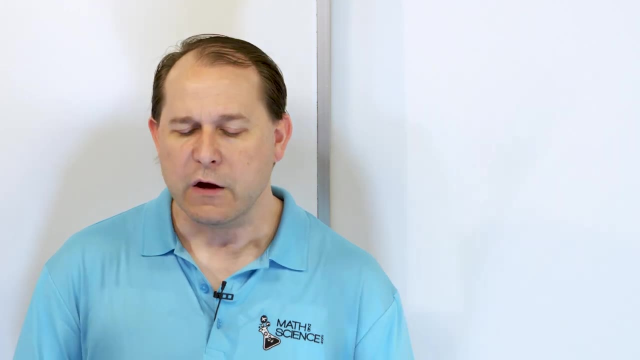 tangent, cotangent, secant and cosecant. So that's six all together. But, as I said, the fundamental ones really are just sine and cosine. All of the other ones come from sine and cosine. So I'm going to write a ton of stuff down and it's going to look intimidating, But in 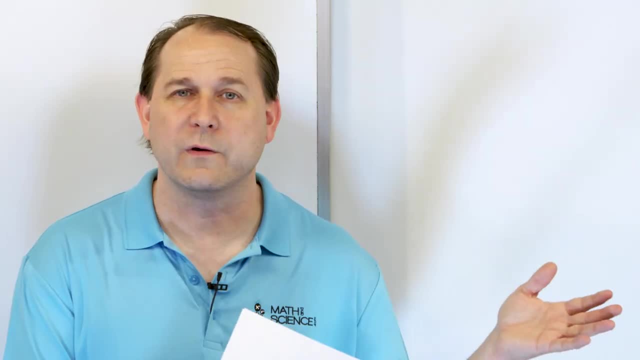 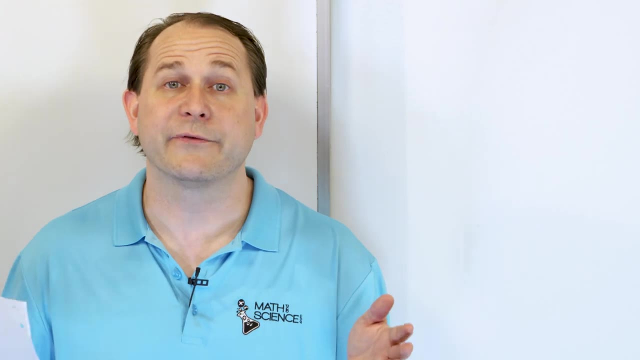 the back of your mind. I really need you to understand that really all that's important, or the most important, is sine and cosine. That's why I spent entire lessons on them just a minute ago. Everything else comes from that, okay. So these are trigonometric functions of acute angles. 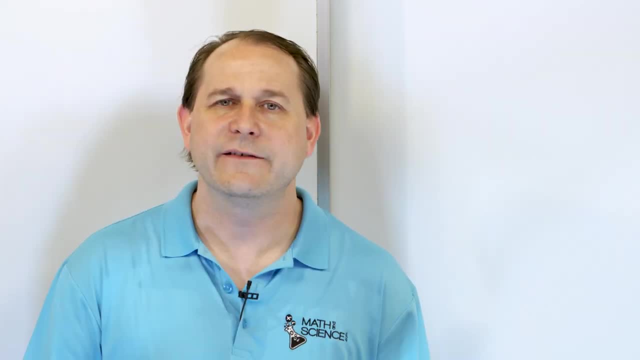 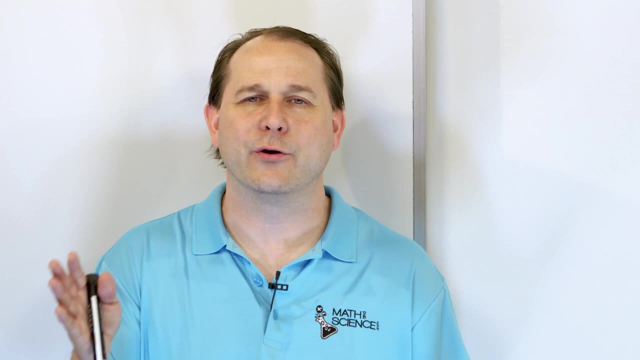 That just means acute angles are the ones that are the most important. So I'm going to go through angles less than 90 degrees, and so that's how we're going to start the discussion. So at first we're going to start learning about these trig functions of acute angles, which are just angles. 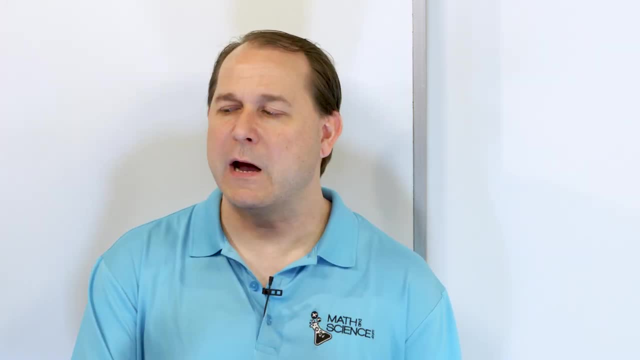 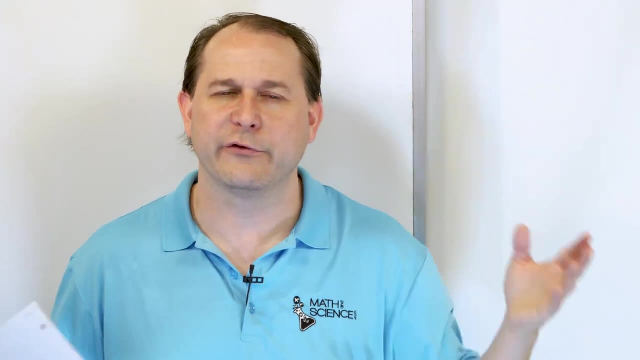 smaller than 90 degrees. But just realize in the back of your mind that as we go through the lessons, we'll be extending it to what happens when the angle is larger than 90 degrees- All these crazy large angles we already introduced we're going to know and have to learn how to take. 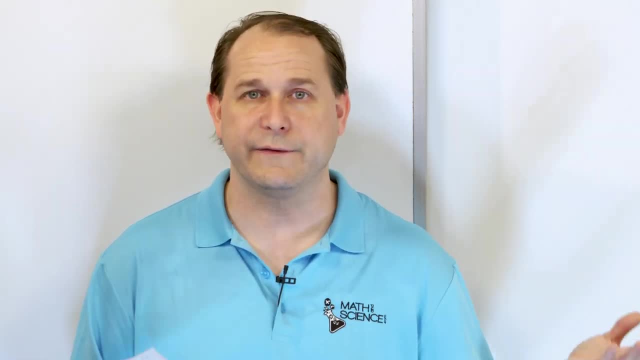 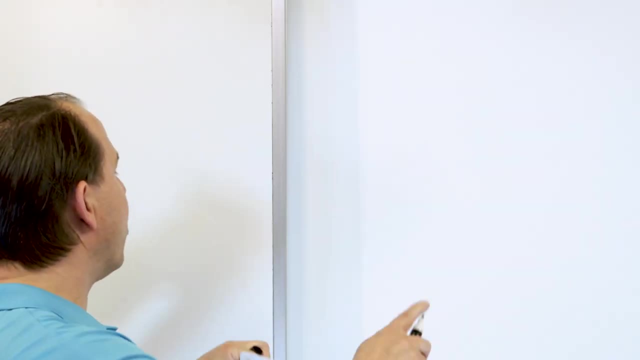 trig functions, sines and cosines and tangents and so on, of all of those angles too. But we have to crawl before we walk, so we're going to talk about the trig functions of acute angles, All right. so what I'm going to do is draw a triangle on the board and I'm going to write all 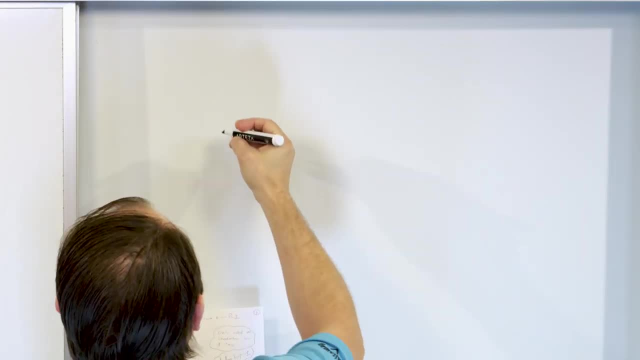 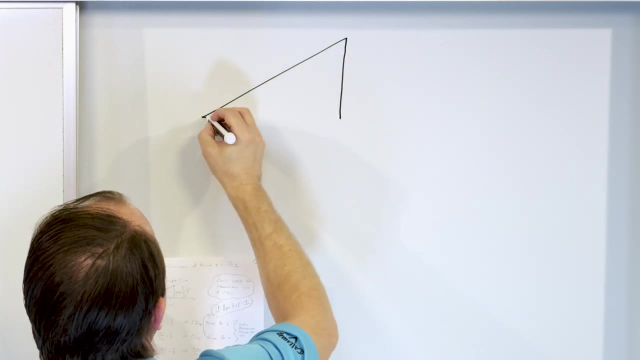 the trig functions down and then we're going to talk about them, and you should understand exactly where they come from by the end of this. So everything boils down to what a triangle is, So we're going to draw a right triangle. When I say triangles, everything boils down to triangles. I 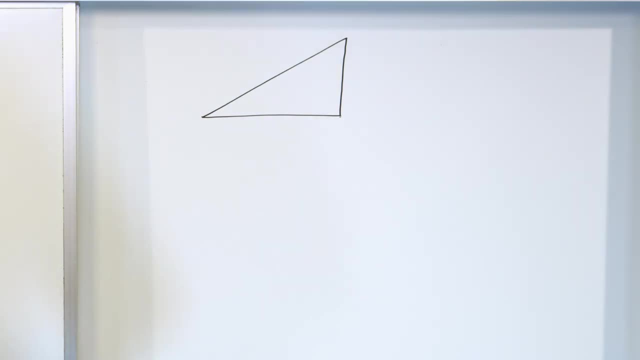 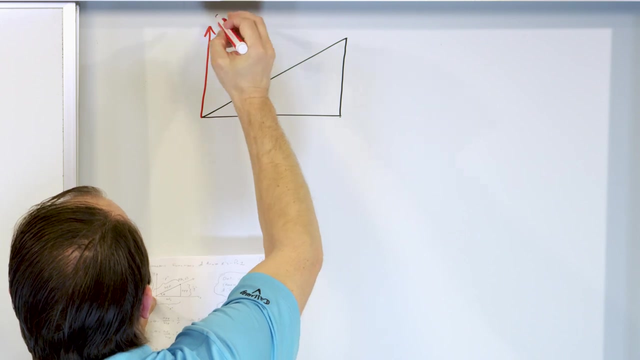 mean right, triangles, okay. So what I'm going to do is draw a little triangle there and then we need to kind of superimpose the triangle on an xy-axis. So the y-axis is the triangle that's going to. that's a terrible y-axis. Let me see if I can clean that up a little bit. The y-axis is: 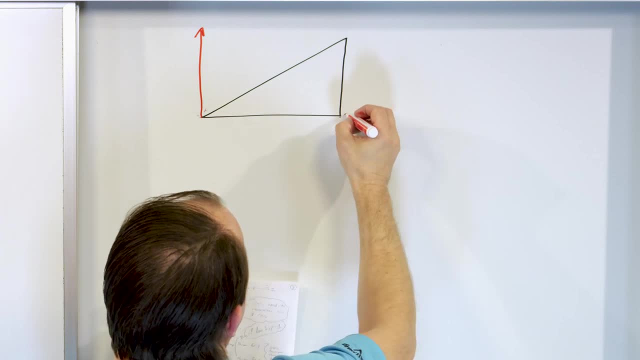 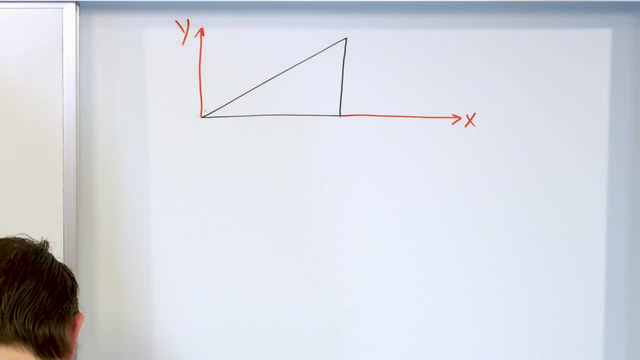 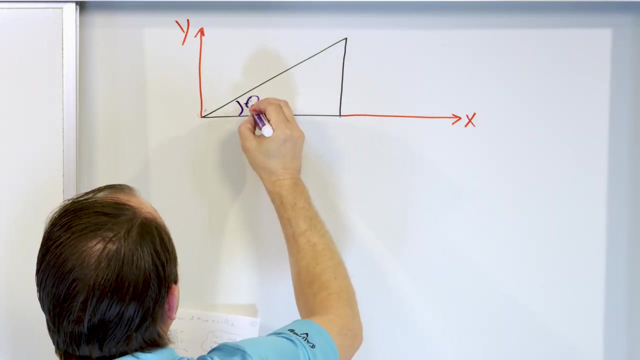 going to be going straight up and down a little better, not too much- And then the x-axis is going to be going across like that. So this is the x-axis. You all know this is always the y-axis And there is some angle. this ray right here is some angle. theta to the x-axis, Remember. 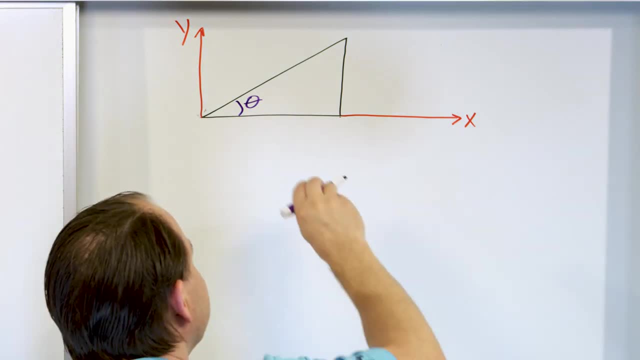 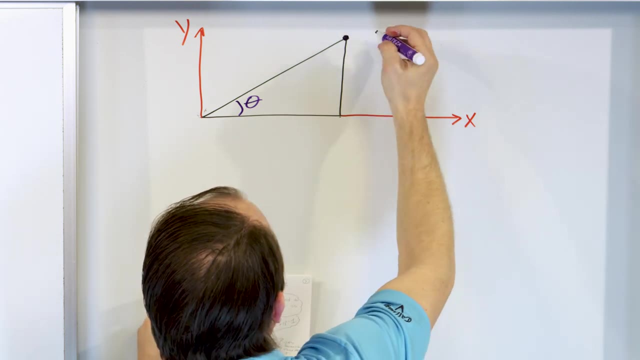 all angles are measured with respect to the positive x-axis, So this is just the angle measure right there. Now the tip of this ray right here there forms some point right at the end here, And so this point has some x and y coordinate over here. I don't know what they are, It doesn't matter. But. 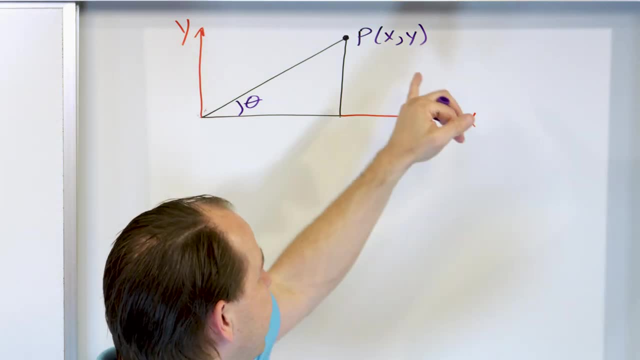 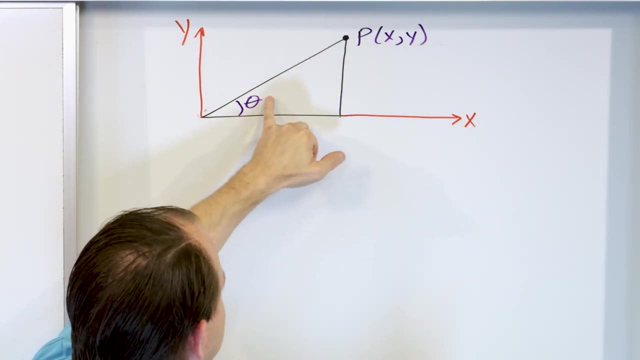 every point in the xy plane has an xy coordinate. So we're just saying there's a point right there at the end. We call it p. It has some coordinates x and y, And when you connect this point to the origin there forms some angle theta right here. All right, Now we have to talk about this triangle. 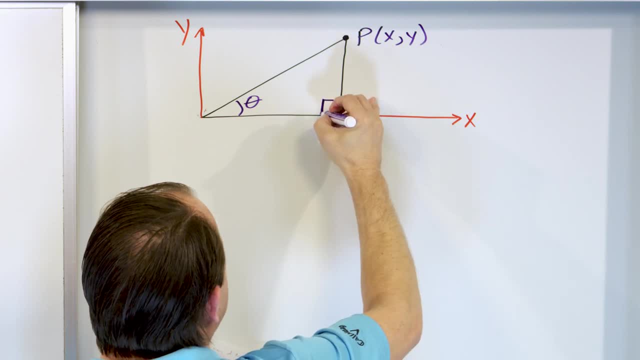 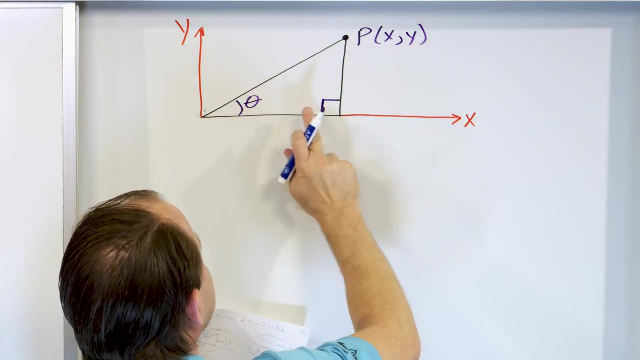 which is the black thing. Now, remember: this is a right triangle because we have a right angle right here. All right, So what we need to do is label a few things Now. the hypotenuse of the triangle is always opposite from the right angle, So we're going to call this hyp. That means hypotenuse. 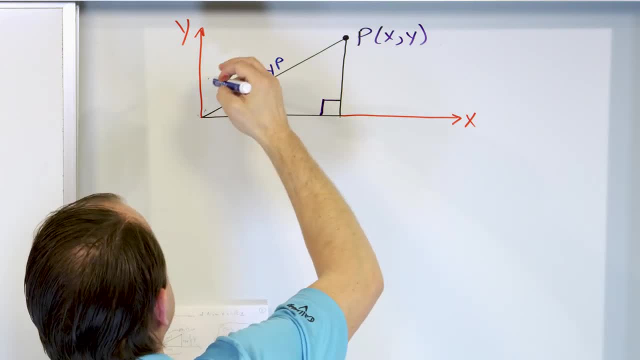 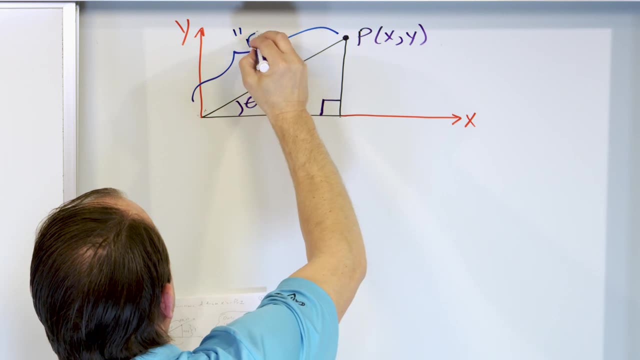 Right, But also we're going to label it in a different way as well. So I'm going to do a little curly brace like this and tell you that this length right here we're going to call it r- You, in different books, might see different letters. It doesn't matter what your book has, or 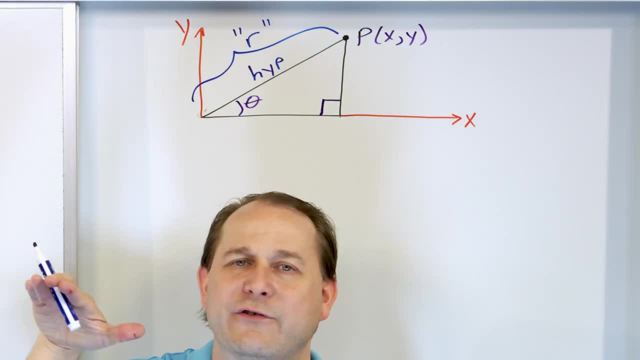 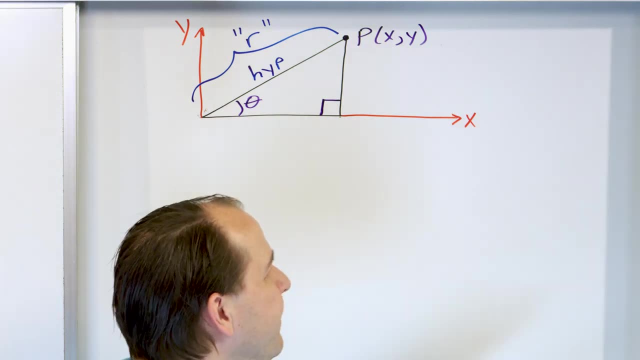 exactly the notation. All I'm trying to tell you is: every triangle- that's right- has a hypotenuse and the hypotenuse- sometimes you call it c for Pythagorean theorem. We're just going to call it r here, So that's what. 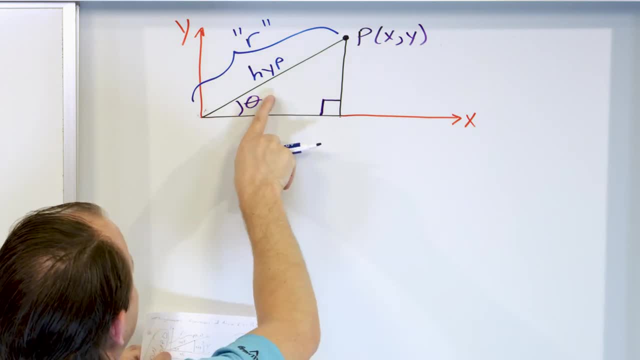 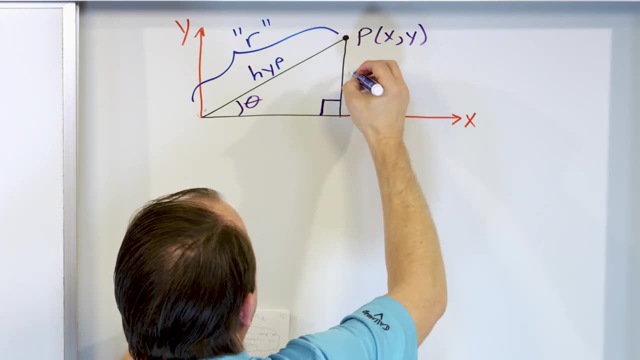 we're doing, And so we have a hypotenuse here. Now this angle has a side of the triangle that is opposite to it. That's this side and an adjacent side of the triangle here. So this side is what we call the opposite side. OPP means opposite And this side of the triangle is called the adjacent. 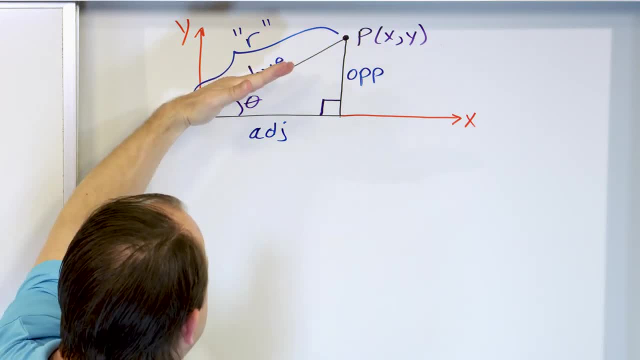 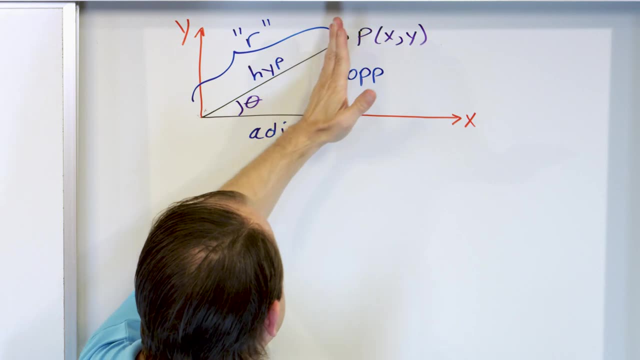 side. So when you look at an angle You need to kind of figure out where the hypotenuse is. and when you go down to the side closest nearest this angle, here that's called the adjacent side and the side opposite to that angle. 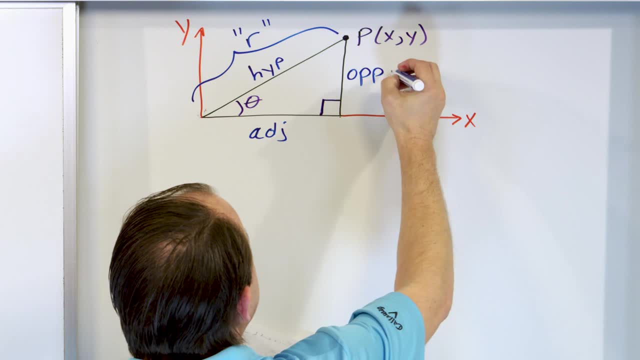 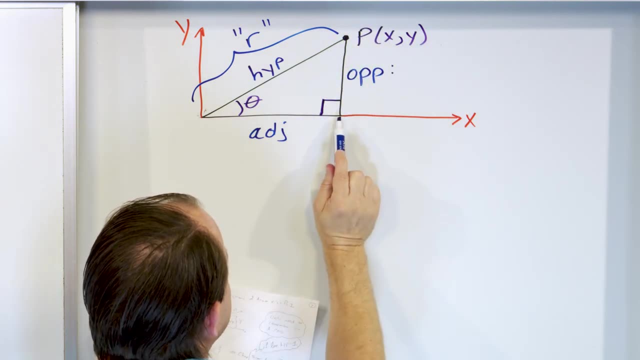 is called the opposite side. okay, So the opposite side is basically, if you think about it, the opposite side of this triangle goes from this point P down to the axis right here. So really, if I kind of get my curly brace in here, 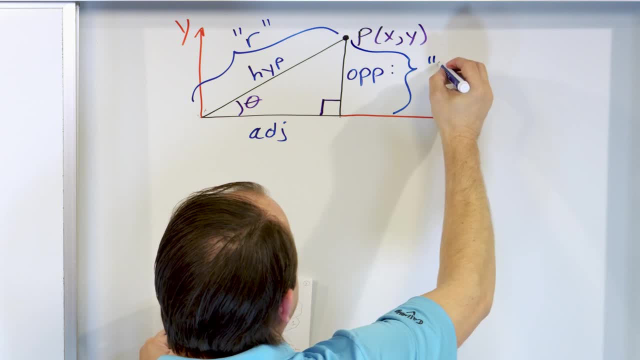 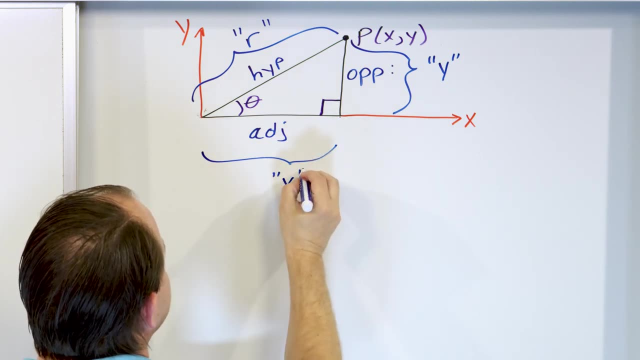 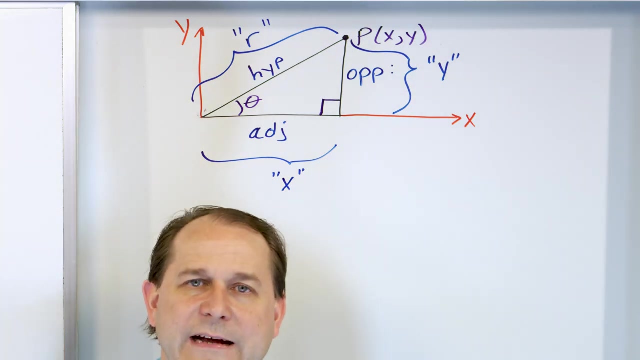 like this, something like this: this distance is y units above the axis. like this, And then this distance right here, this distance is x. The reason I'm drawing all this stuff is because usually, when you first learn trig functions, you talk about opposite and adjacent sides. 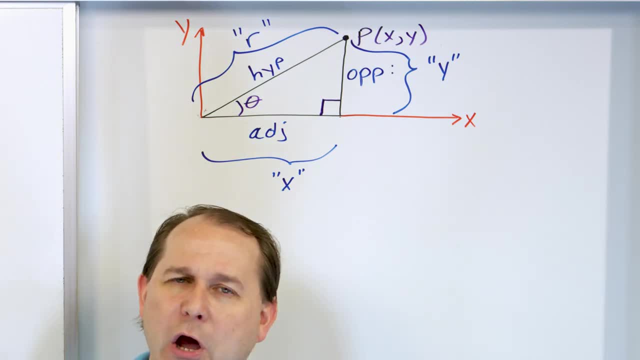 and that's handy for a bit, but you eventually drop that and you don't talk about opposite and adjacent when we get a little farther into the class here We talk about the x side and the y side and all of this. So I'm drawing everything on one figure. 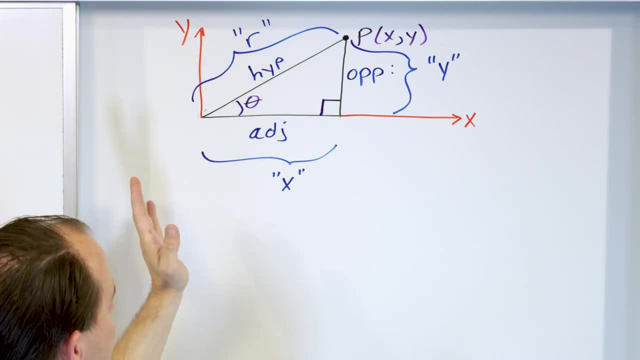 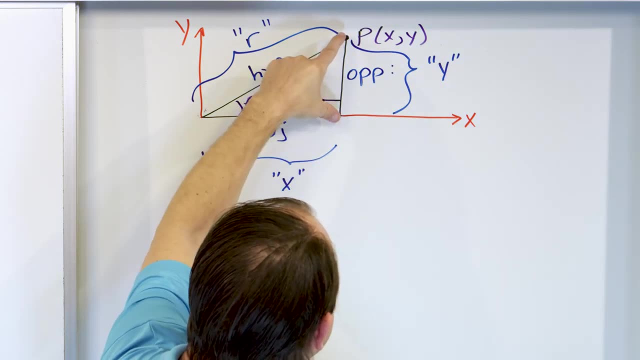 I'm saying: hey, every triangle has a hypotenuse. we also call it r. Every triangle has an opposite side. we also call it y. The reason we call it y is because there's y distance units from here to the tip of this triangle. okay, 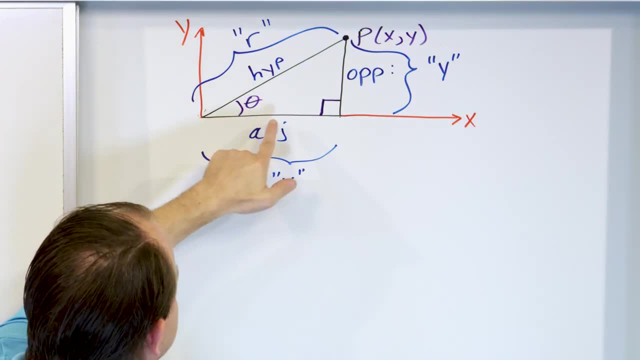 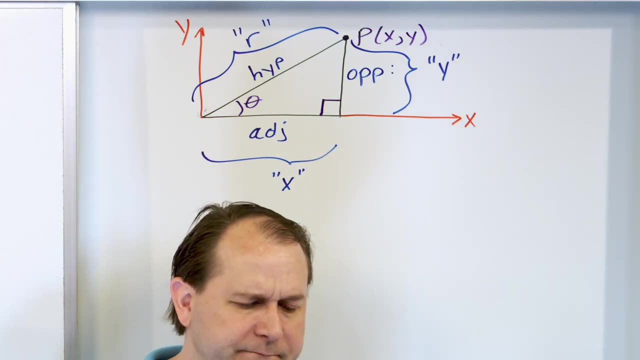 Every triangle also has an adjacent side, adjacent to this angle. We also call this side x, because it is x, distance units from here to here. so x, y and r. So that's what we're basically doing, all right, Now what we're gonna do is use this triangle. 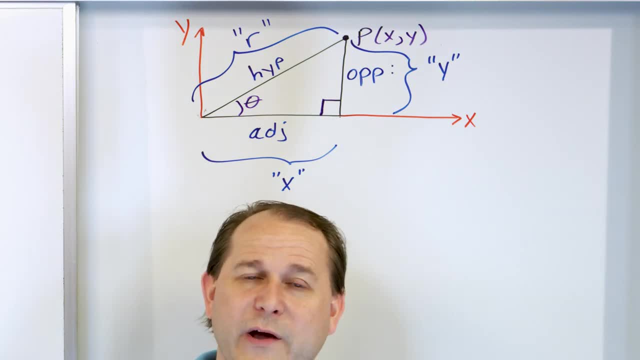 to define the six trigonometric functions, and then I'm gonna show you a quick way to understand how to remember them all. So I really only need you to understand sine and cosine. Honestly, the rest will just fall out of the discussion. 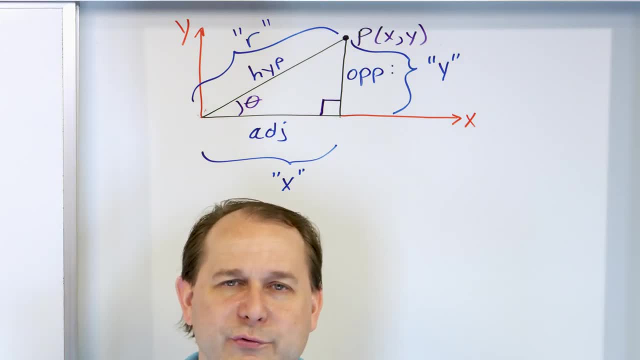 And then we'll solve, of course, some problems toward the end, and a bunch of problems as we go through the lessons here to make sure you're comfortable with it. All right, so the first trig function that we must, must, must understand. 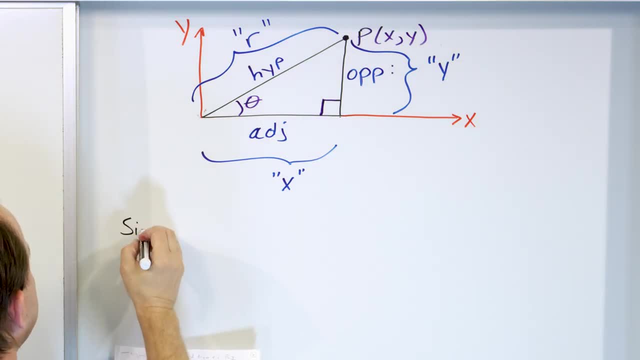 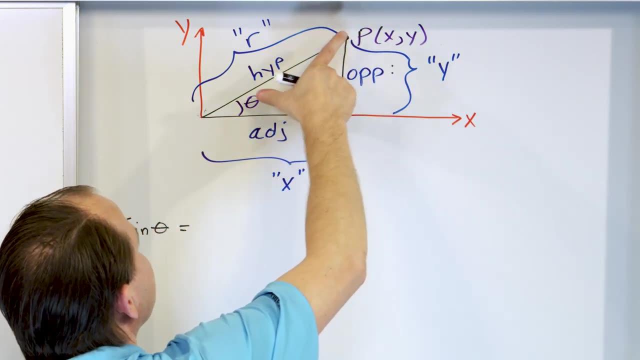 we've already introduced it in the last lesson. It is called sine of this angle, theta. So sine of this angle, theta, is defined to be the opposite side of this triangle divided by the hypotenuse of the triangle. So sine is the opposite side over hypotenuse. 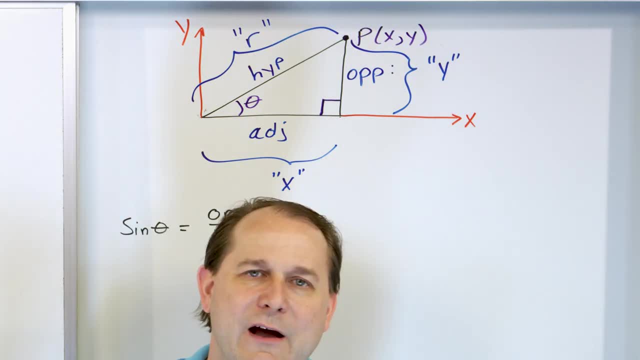 In every textbook that you open, whether it's geometry or algebra or calculus or precalculus or trig or whatever, you'll always see a triangle and it'll have an opposite side, an adjacent side, and you'll see that the sine function. 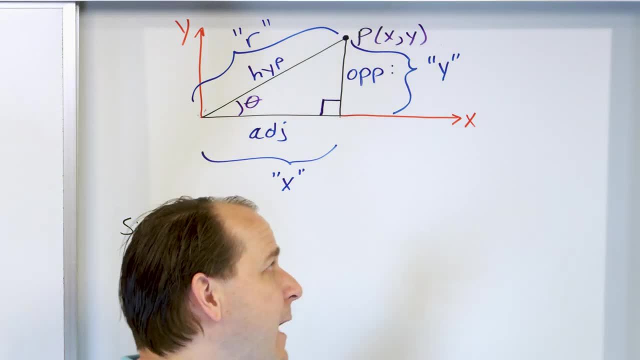 is defined to be the opposite side of the triangle, divided by the hypotenuse. That means, if I actually measure, if I took a ruler and measured this length and then measured this length and divided them, that would be what we call sine of this angle. 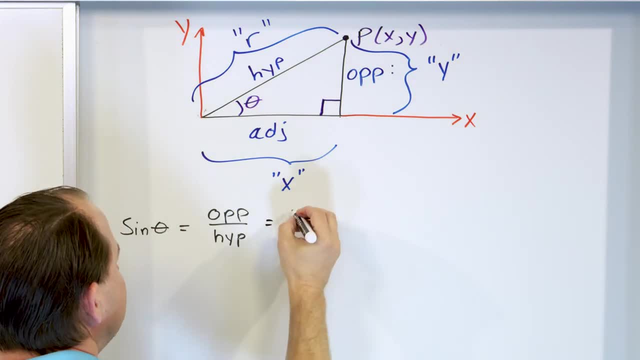 Now, because the opposite side is also called y, we can put a y up here. and the hypotenuse is also called r, we can put an r down here. So the sine of the angle is y over r. It's just the opposite over the adjacent side, right. 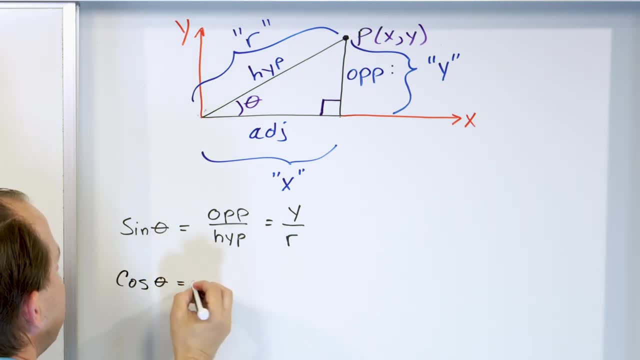 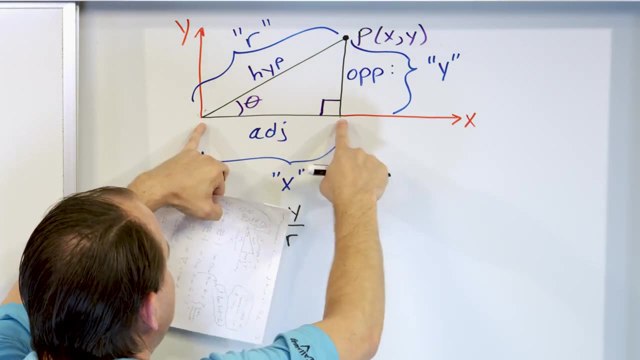 Now the cosine we also introduced in the last lesson and that was defined to be the adjacent side of the triangle divided by the hypotenuse. So if you take this side of the triangle, measure it in however many centimeters it is and divide by this, 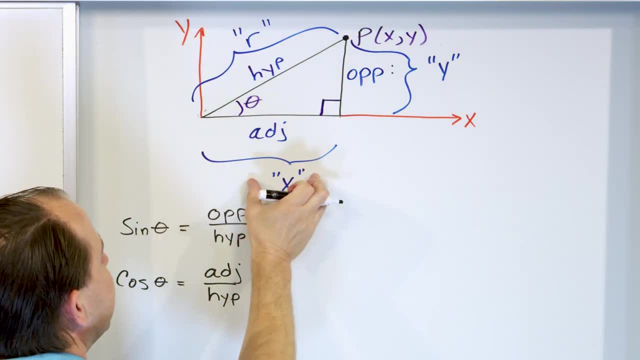 then what you'll get is what we call the cosine. Now, since the adjacent is the x- very important variable- or the x-label, we can say: this is x over r. So you see, we use this opposite adjacent. hypotenuse business at first. 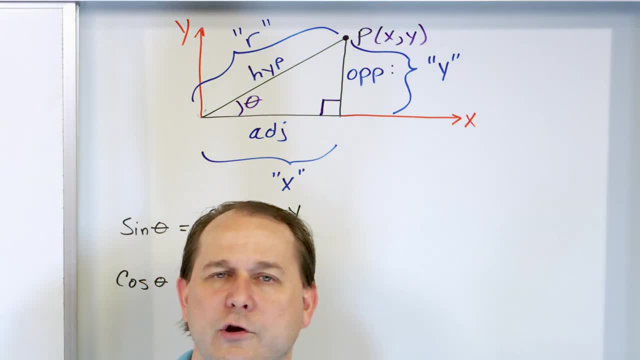 but eventually we're gonna drop all that and we're just gonna start talking about x's and y's and r's. So in your mind you need to have this triangle burned in so you know what that actually is, and that's why I'm drawing it here. 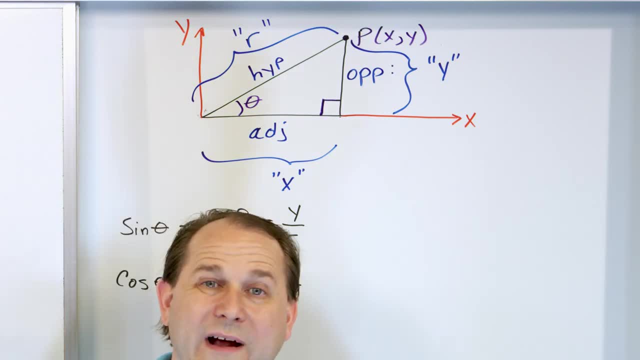 Now, in the last lesson we spent a tremendous amount of time talking about what sine and cosine really mean. If you haven't watched that lesson, I actually really, really hope you pause this. go watch it first. But I'm gonna summarize what we did in the last lesson. 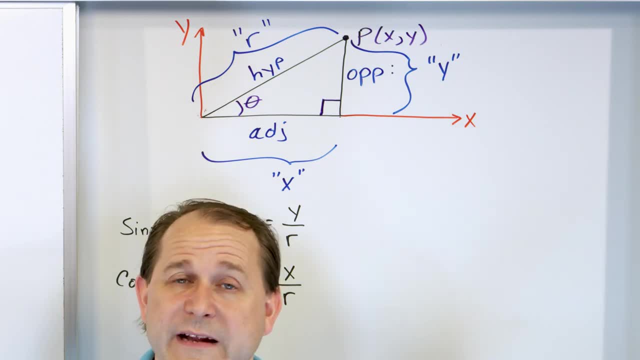 But I'm gonna summarize what we did in the last lesson. We did it in about 30 minutes. in the previous lesson took 30 minutes to go over it in great detail And I'm gonna summarize it in the following way: When you see sine of an angle, 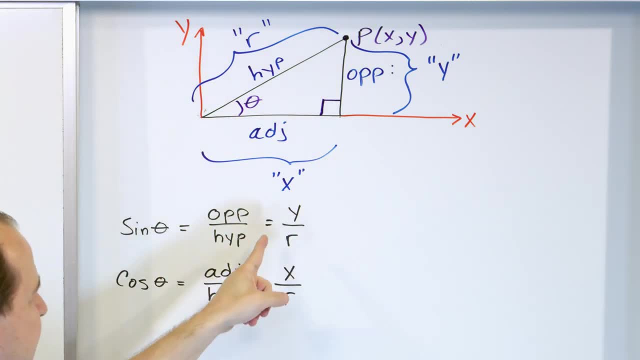 what you really are talking about is: it is the ratio. it is the ratio of how much this triangle goes up. compared to that means division, compared to how much total length of the hypotenuse of the triangle there is. And I told you in the last lesson. 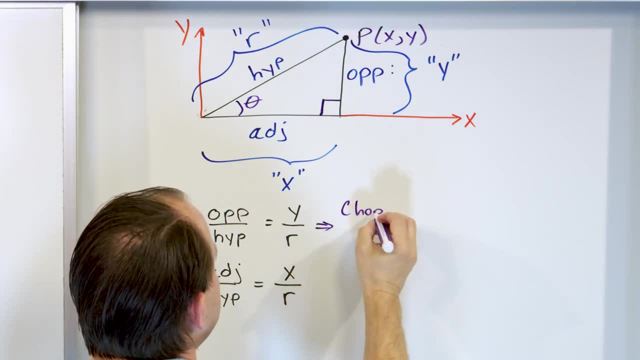 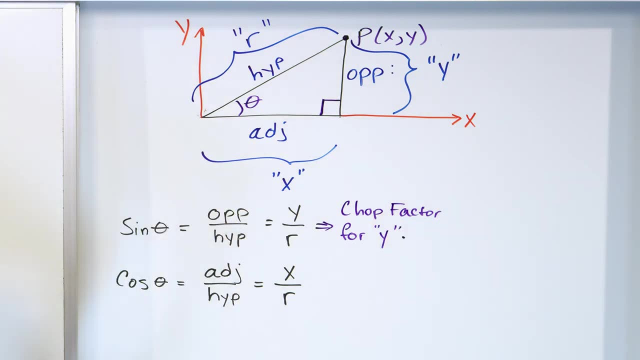 that we called this the chop factor, And I told you in the last lesson that we called this the chop factor. The reason we call it the chop factor- and that's my word. that's not a word that you're going to see in a book anywhere. 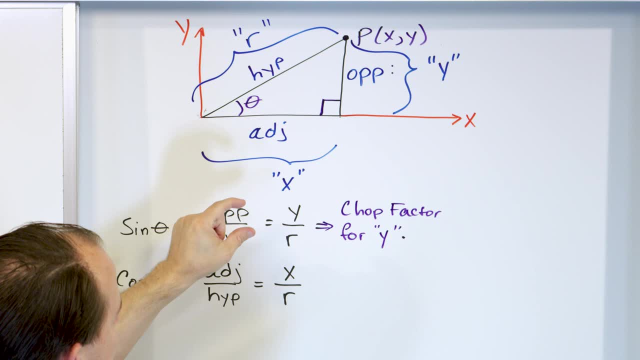 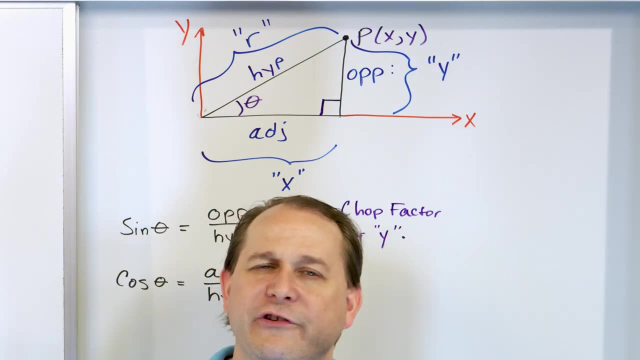 is because it is literally a decimal that comes out. It's a number less than one. When you take y and divide by r, you get a number less than one And it tells you in a number form how much of this triangle is going up in the y direction. 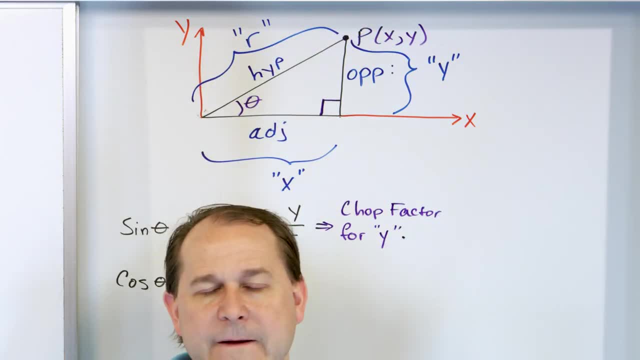 compared to the total length of the triangle, which is the hypotenuse. So, if the chop factor for y is very small, which is the hypotenuse, which is the total length of the triangle, which is the hypotenuse, which is very big. 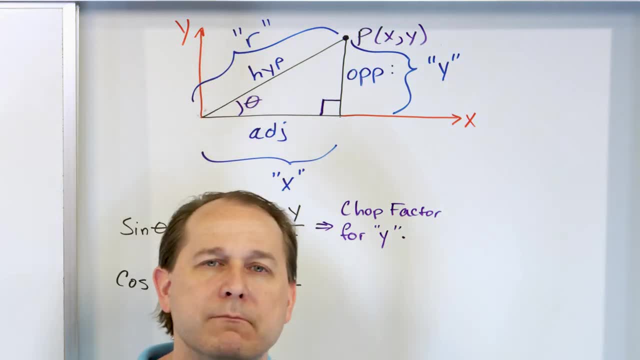 then that means that this y, this triangle, is really tall and most of the triangle is going up. okay, But if you have- I'm going to get to it in a second- but the chop factor in the x direction, if you have a large chop factor in the x direction, 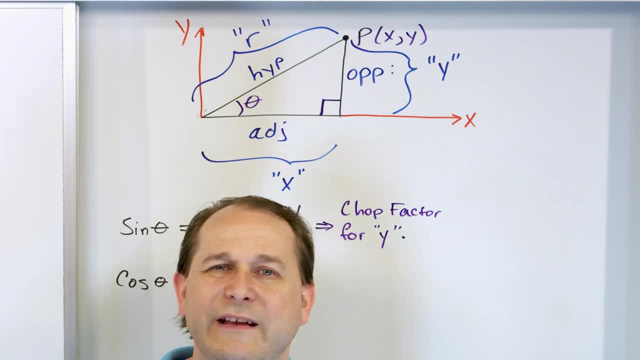 it means that most of the triangle is actually going along the x direction. So these chop factors are my words, but sine basically tells you how much of the triangle is going in the vertical direction, in the y direction. Is it a really tall triangle in the y direction? 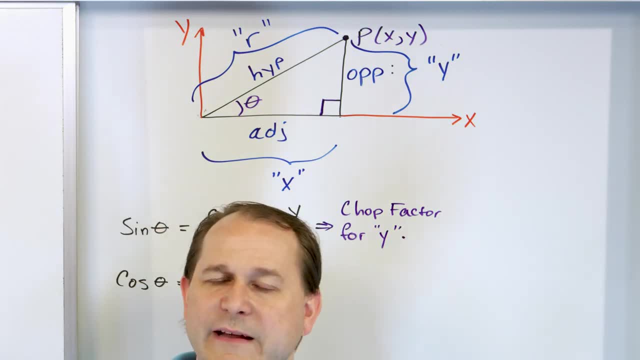 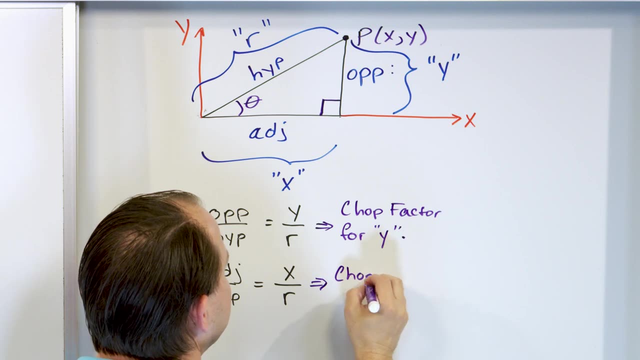 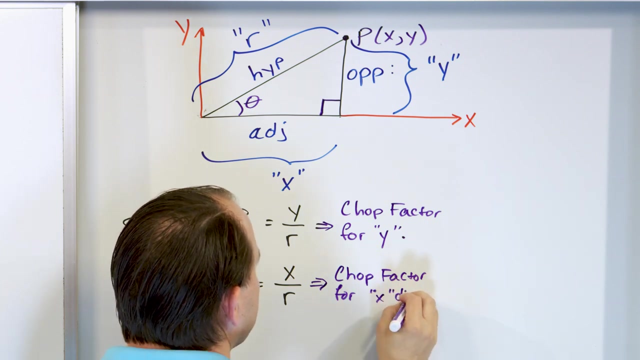 And if you have a very small chop factor in the y direction, it means that that's not the case And the similar thing for here. So we said in the last lesson that this cosine is the chop factor for the x direction, right? 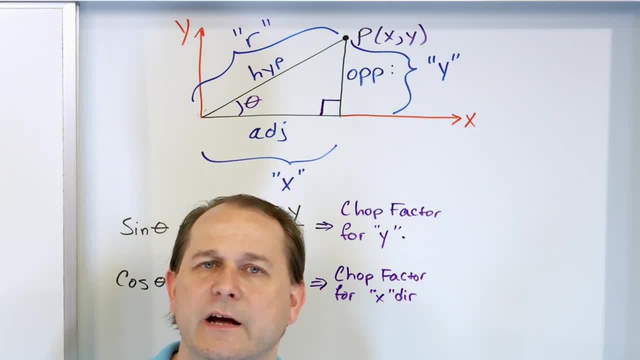 Because we learned in the last lesson that if we know what the sine and the cosine is of an angle and there's a button on your calculator, we're going to learn how to use it later. but if you know what the sine and cosine of an angle is, 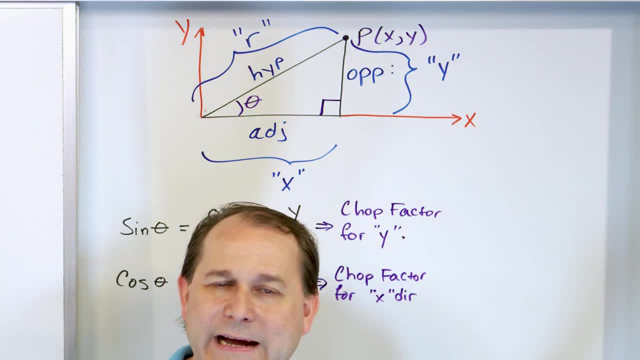 then you know what these chop factors are. Sine goes with y, it is the chop factor in the y direction, and cosine goes with x, that's the chop factor in the x direction. And so, if you know what these chop factors are, 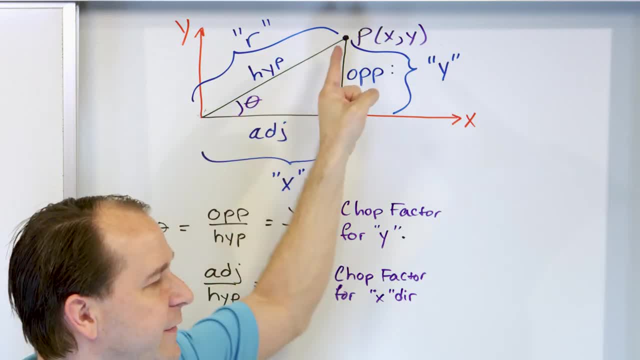 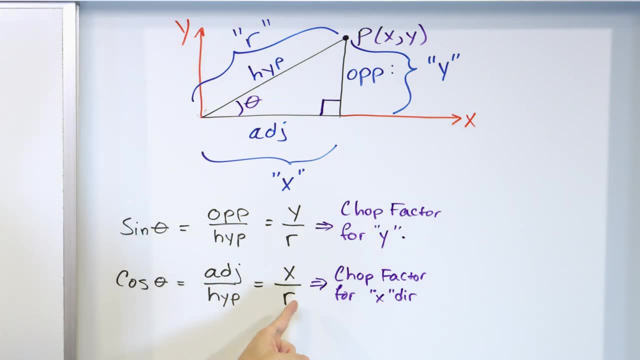 then I can take the chop factor and multiply by the hypotenuse and that will tell me how many units my triangle is in the y direction if I'm multiplying by this one. And if I multiply by this one, it's telling me how many units it is in the x direction. 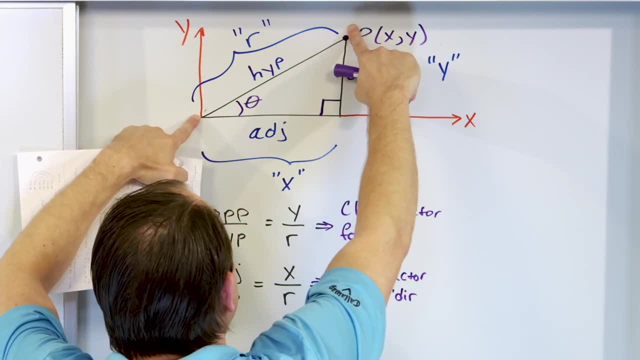 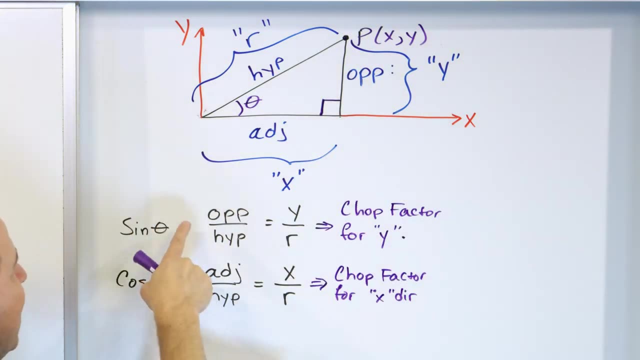 In other words, if I know that my triangle has a hypotenuse of 10 meters, if I multiply by the sine, which is the chop in the y direction, then I'm going to get this side of the triangle Because, look, it's opposite- over hypotenuse. 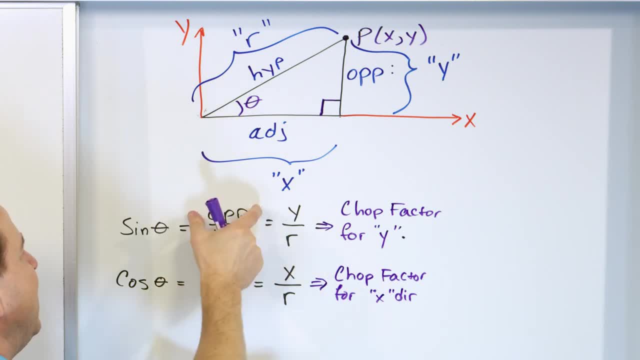 If I then multiply by the hypotenuse, the hypotenuse will cancel and I'll be left with the opposite side. That's why it's called the chop, because when you multiply by the hypotenuse, if you multiply the sine of the angle times the hypotenuse. 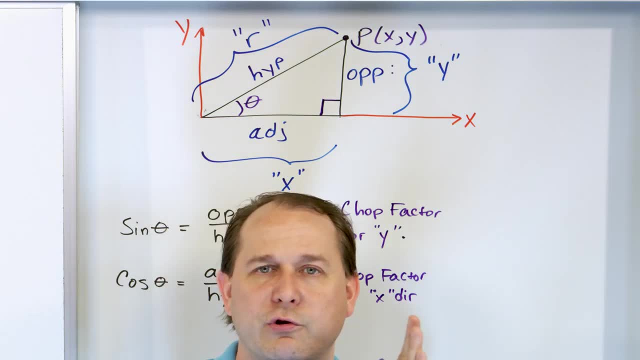 it cuts the hypotenuse down and only tells you how much of it goes in the vertical direction. If you take the chop in the x direction and multiply it by the hypotenuse, then what you're understanding, as the answer is, it's chopping down that hypotenuse. 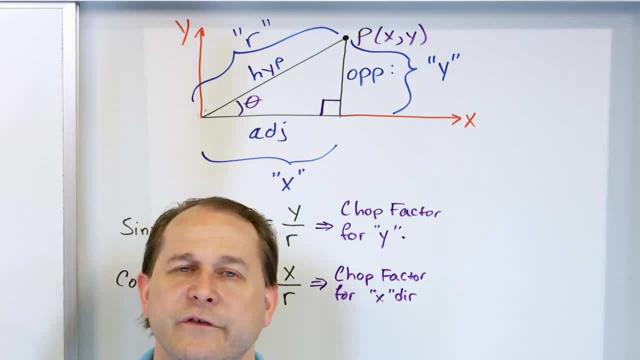 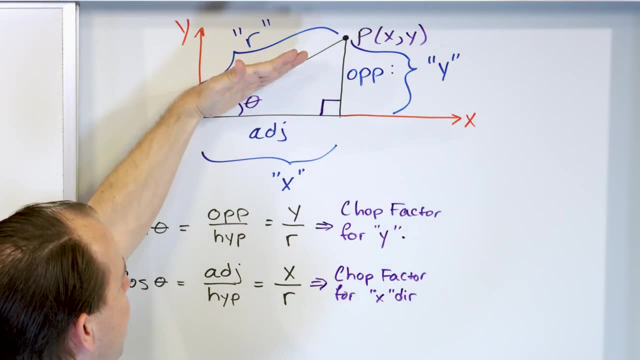 and telling you how much of this hypotenuse exists in the x direction. So I call it chop in x and chop in y, because when I multiply those factors times the hypotenuse, if I multiply, the hypotenuse times the sine. 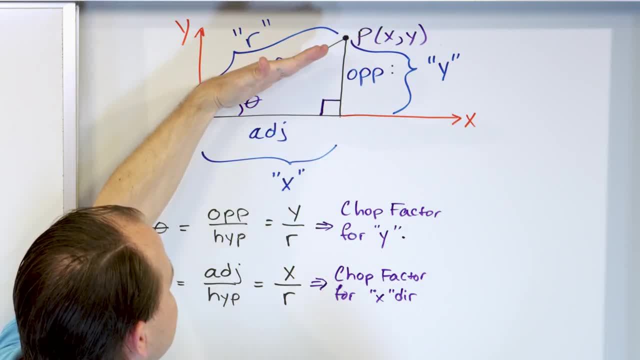 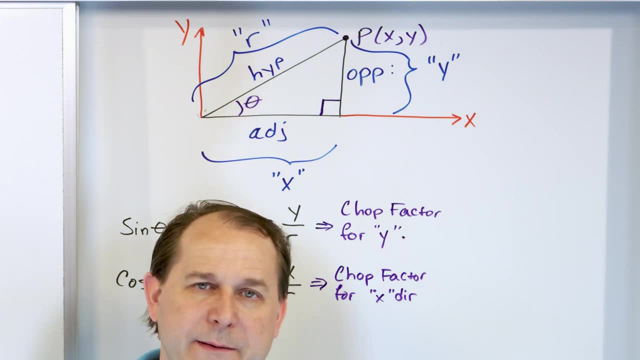 it gives me the length of the opposite side. If I multiply the length of the hypotenuse times the cosine of this angle, it gives me the length of the adjacent side. And that we're going to learn through solving many, many problems. 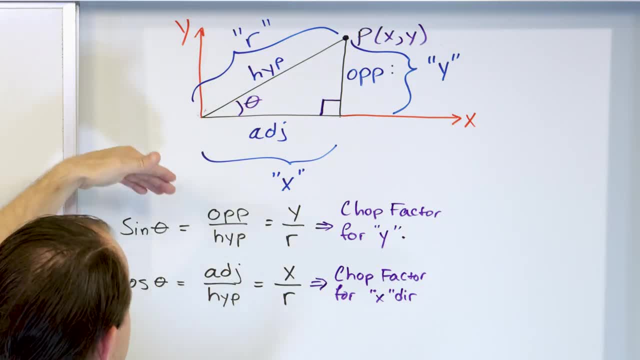 That's why I call it the chop factor. Another way you can look at it is: it's a projection, If I shine a light in this direction. the shadow, if I shine a light in this direction. if I shine a light in this direction. 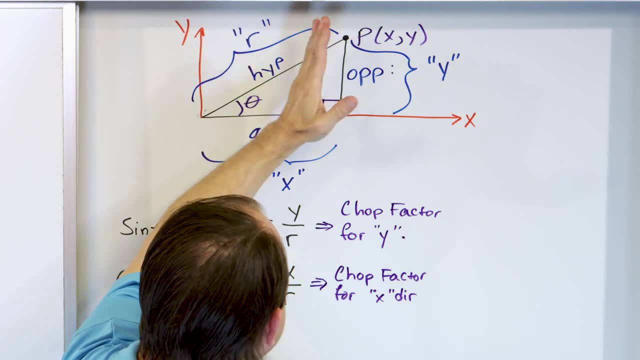 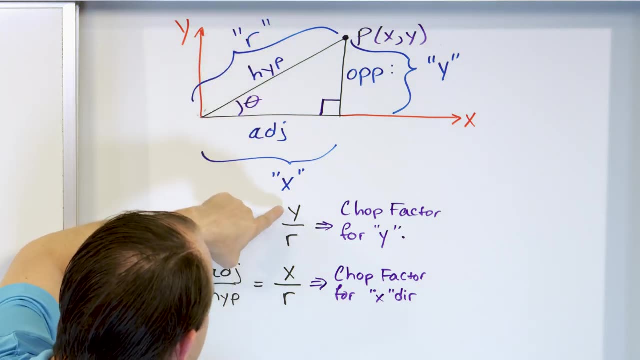 if I shine a light in this direction, the shadow that the hypotenuse creates over here against a screen- if I put a screen here- would be the length of this triangle. So the sine of the angle is basically telling you, since it's a ratio of y to hypotenuse. 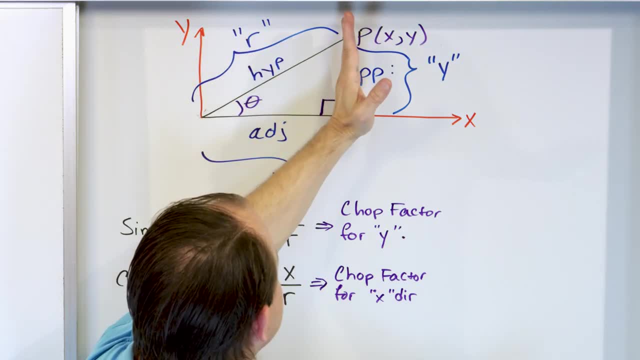 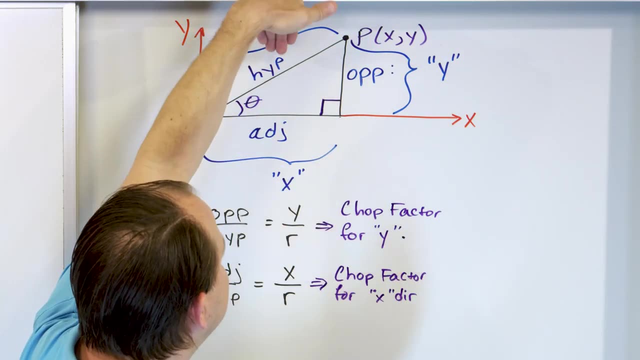 it's telling you how much of that shadow is going to exist over here, And so it's kind of a projection of that hypotenuse onto a screen over there in the y direction. Or if I put a light vertically underneath like this, it would cast a shadow down there. 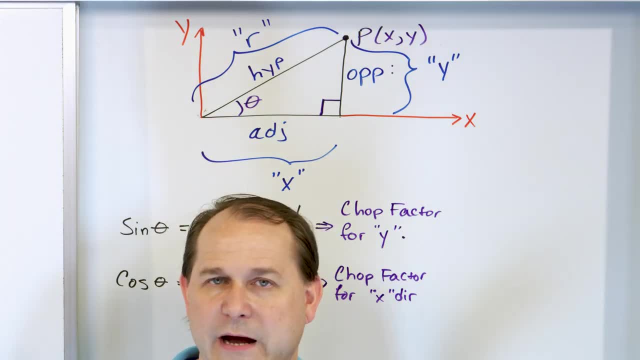 So the sine is kind of a projection in the y direction of the hypotenuse, And the cosine is the projection of the hypotenuse in the x direction. So whether you think chop in x and chop in y, or projection in x, projection in y, it's all the same thing. 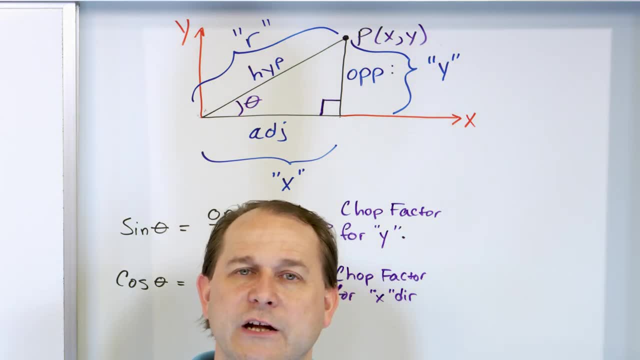 The sine goes with the y direction, The cosine always goes with the x direction, And that is something you must remember. All right, so now that we know what sine and cosine are and we've kind of revisited what we already learned in the past, we need to talk. 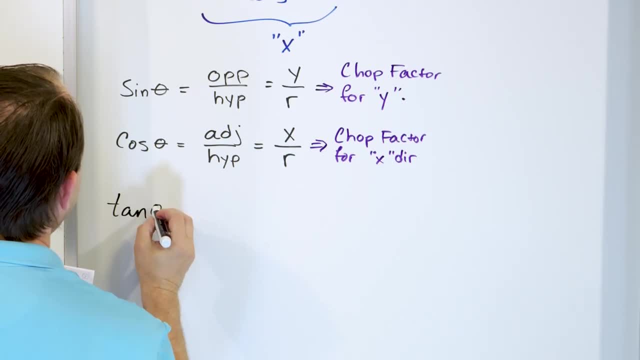 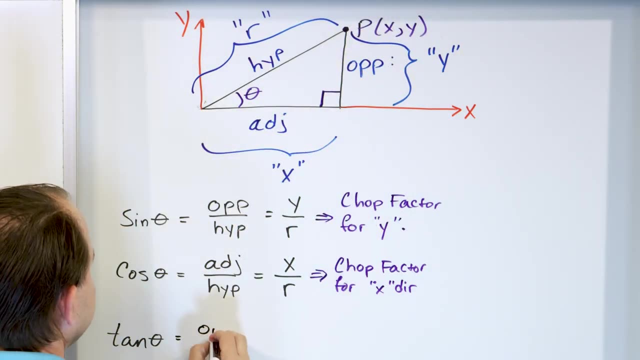 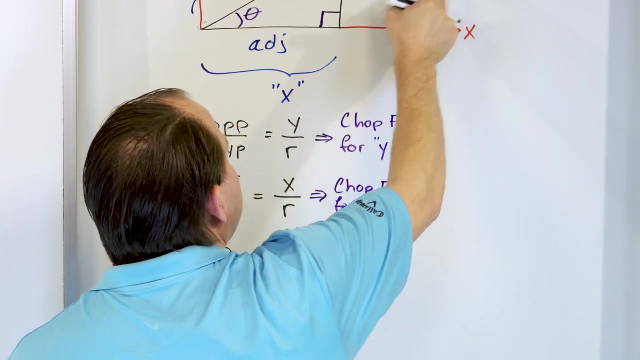 about the tangent function. So the tangent of some angle, theta, is defined as follows: The opposite side divided by the adjacent side. So the opposite side divided by the adjacent side. like this: So the opposite side is y and the adjacent side is x. 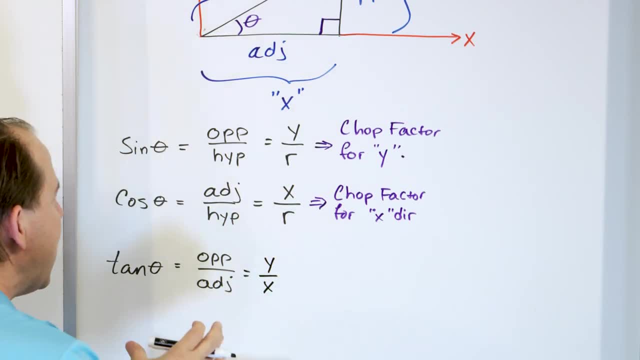 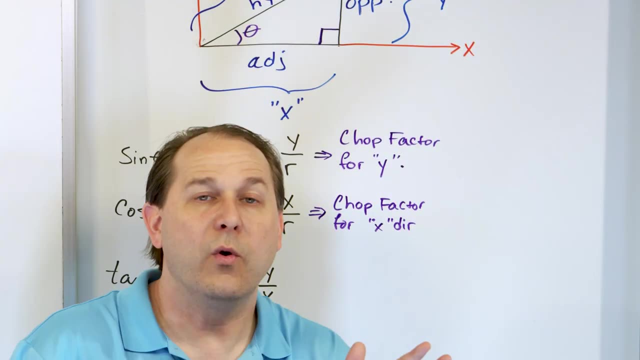 So if I put it in that notation, it will be y over x. Now we said that the sine is the ratio of how much the triangle goes up compared to its total length, So it's telling you what fraction of the triangle is going in the vertical direction. 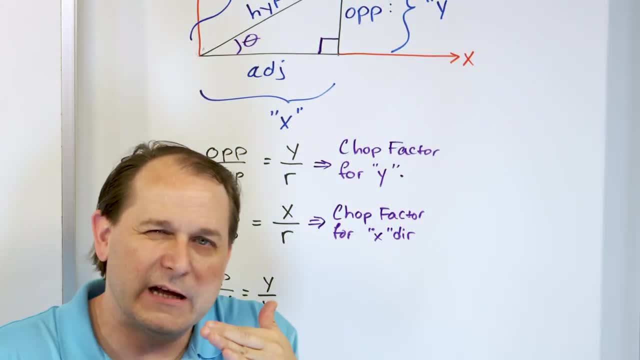 The cosine is the division of x, 2, and 1.. So the cosine is the division of x, 2, and 1.. So it's telling you how much of the triangle is going in the horizontal direction. That's why the chopping and the projections come into play. 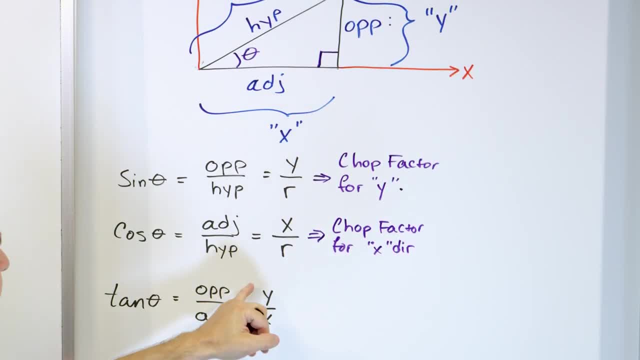 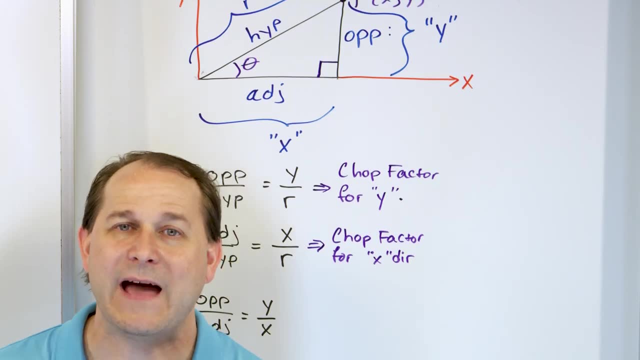 But the tangent doesn't involve the hypotenuse at all. It's just the y direction divided by the x direction, y divided by x, y divided by x. So what does that remind you of? That should be reminding you of the slope of a line. 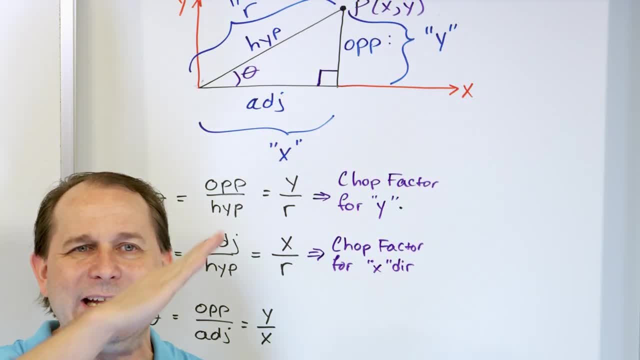 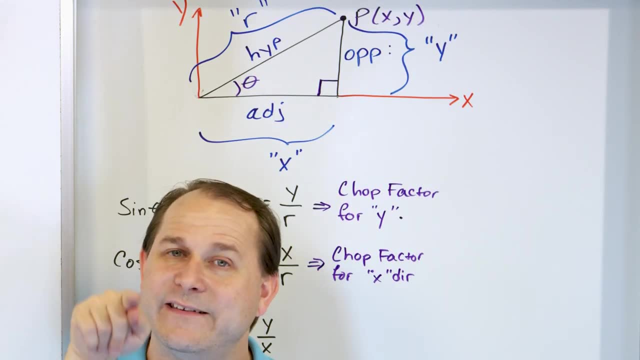 rise over run. Remember, we learned with a line, any line: if you go and look at how many units it goes up, that's the rise, How many units it goes over, that's called the run. The rise is always in the y direction. 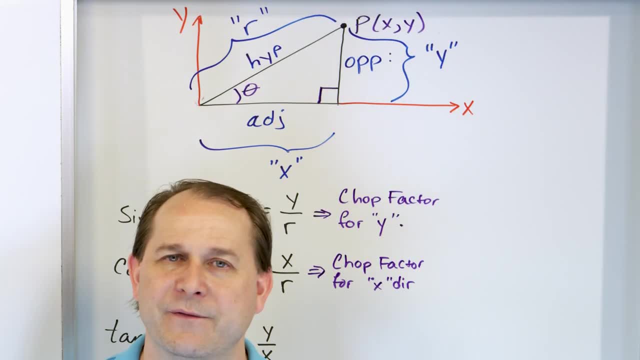 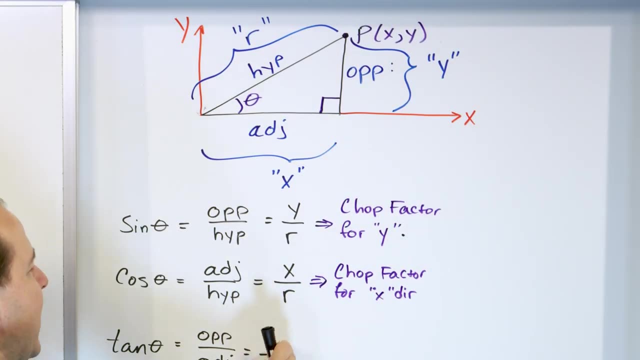 The run is always in the x direction. So when you calculate slope of a line, a long time ago you were always taking how high it goes in y and dividing by how high over it goes in x, y over x. All this is doing is the rise is how many y units is up. 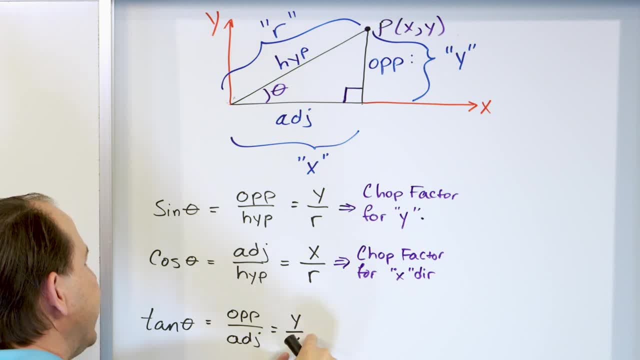 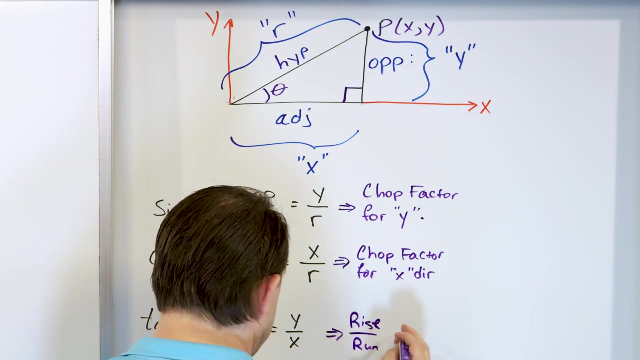 and the run is how many x units over. So when you take y divided by x or opposite over adjacent, the thing that we're calling the tangent of this angle is really rise x, Rise over run. So this is really rise over run. 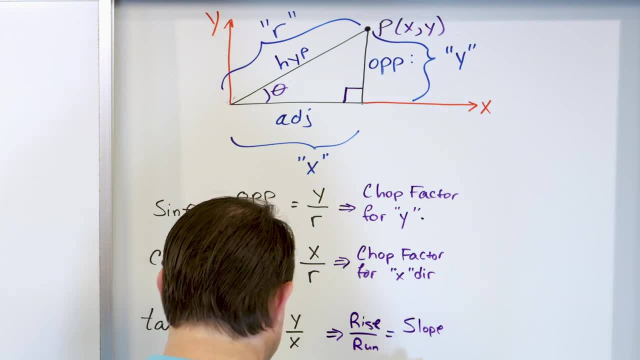 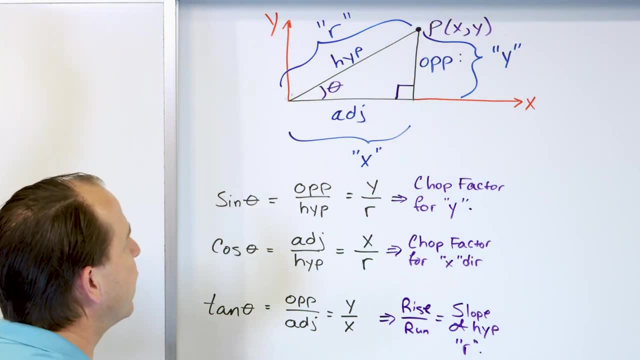 And basically that's going to equal to the slope of the hypotenuse r, because the hypotenuse is kind of the line r we're talking right here. So if you were to draw this, if you calculate y over x, you're calculating the slope of this hypotenuse line. 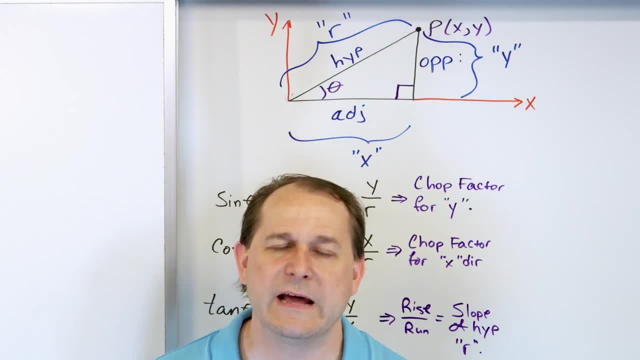 That's not something you often see in books, but that's all the tangent is doing. It is the ratio of y to x, which basically means the slope, The slope of that line. OK, Now, now we get into a little bit of a sticky territory. 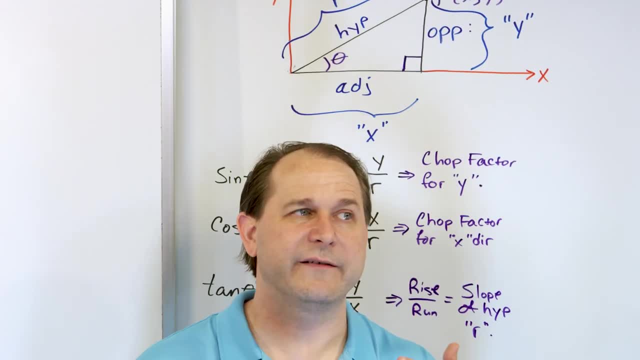 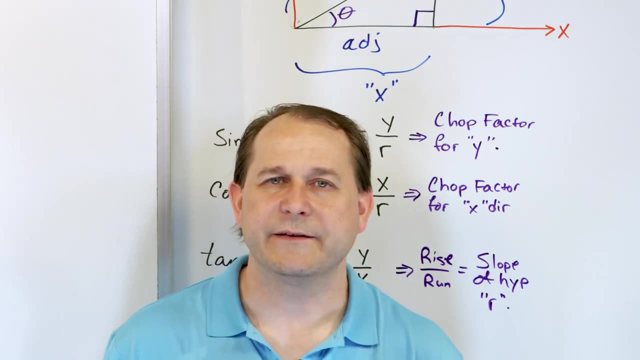 because sine cosine we understand Tangent is just y divided by x, So it's just the sides of the triangle And I can explain it to you as the slope of a line. Those kind of make sense. But then we get into the next three. 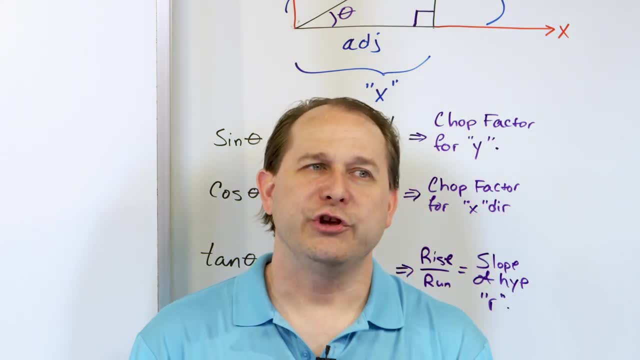 Cotangent, secant, cosecant, And then you're kind of like your brain falls apart, usually the first time, because it doesn't seem to make a lot of sense. Why do we need three extra functions? OK, I'm going to get into the why we need three extra functions. 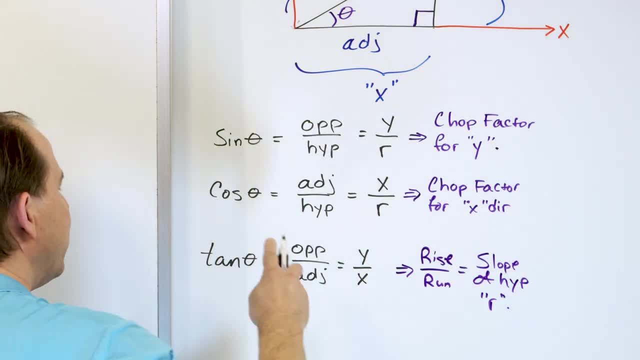 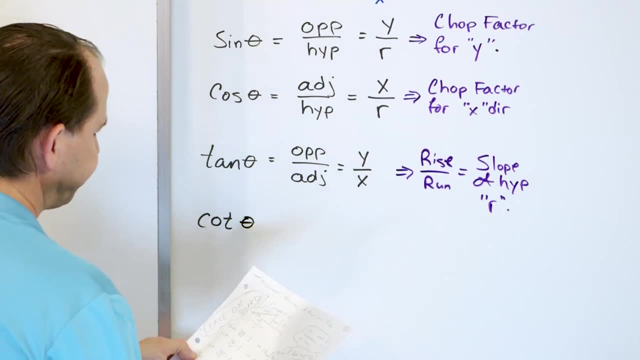 a little bit later, But for now let me write down exactly what they are. So we have this thing called a tangent. We also have something closely related called the cotangent. C-O-T means cotangent of theta. Cotangent is defined to be 1 over the tangent of theta. 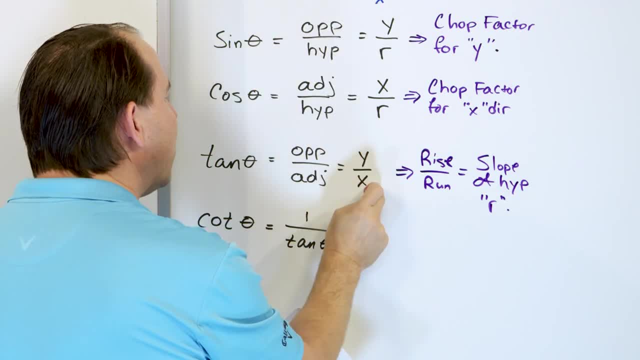 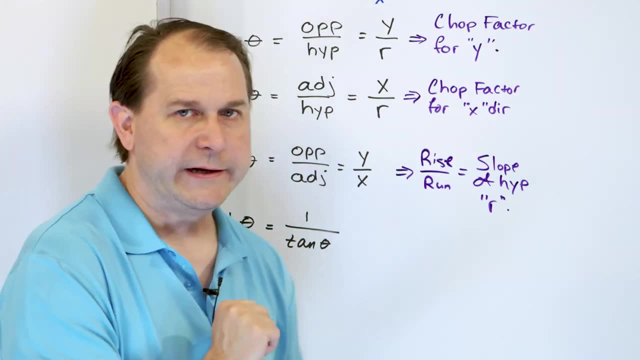 So, literally, if I take a triangle like this and I calculate y over x and I get the tangent, I know what the tangent is. Let's say, the tangent is 3, OK, or something like this. If I take 1 over 3, which I know what the tangent is. 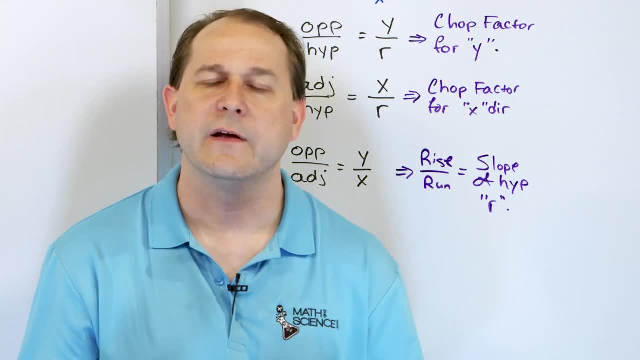 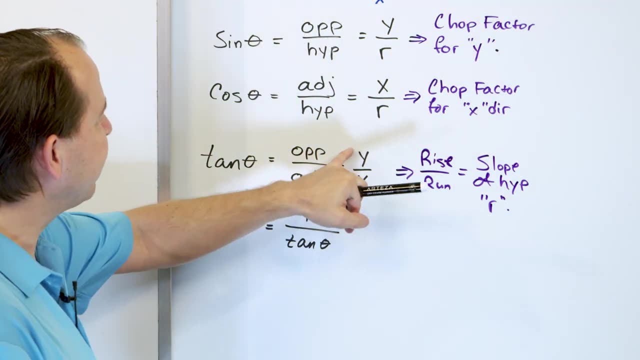 if I stick it in there and say, well, 1 over that. that's what the cotangent is. So you see, the cotangent comes directly from the tangent, It comes directly from the tangent And the tangent is just involving y and x. 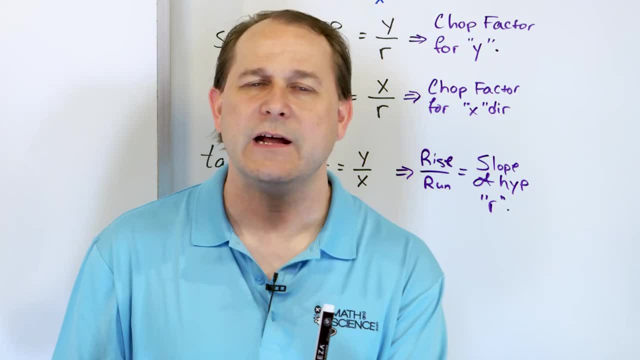 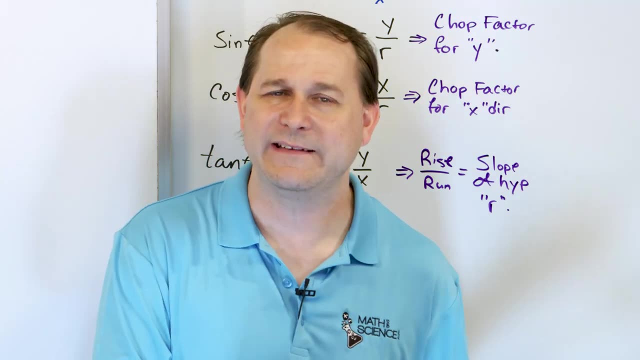 So, really, when I told you the most fundamental things are sine and cosine, that was absolutely true. Sine and cosine are the most fundamental. Tangent can come from sine and cosine and cotangent comes from the tangent. So you see, that's how we remember these things. 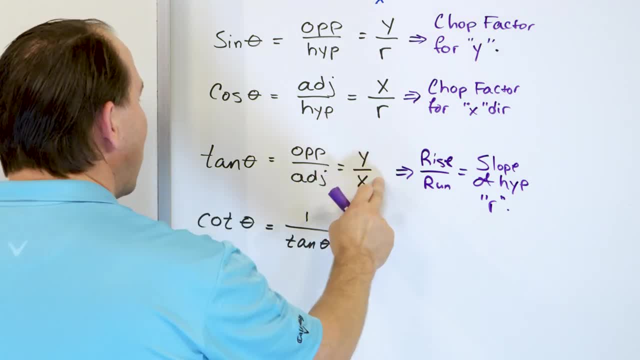 So 1 over the tangent. We have a tangent there. Now what is tangent equal to? It's equal to y over x. So if you think about it, 1 over y over x. if you were to actually flip and multiply, 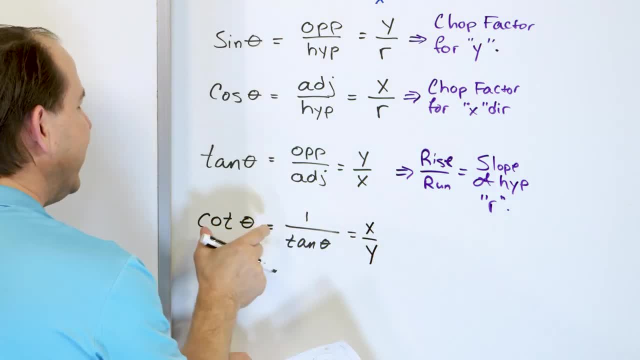 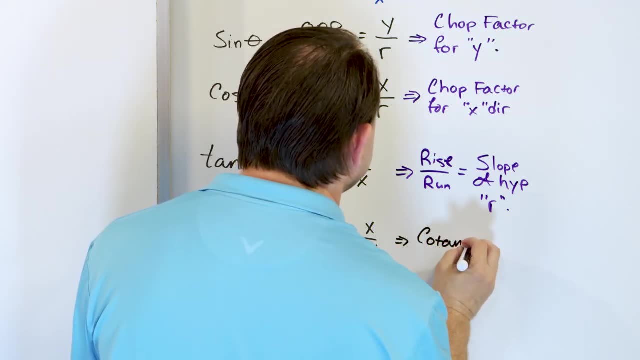 what you would get is x over y. So x over y is cotangent, because it's equal to the 1 over the tangent, And we call this cotangent like this: There's two more. There's one more called the secant. 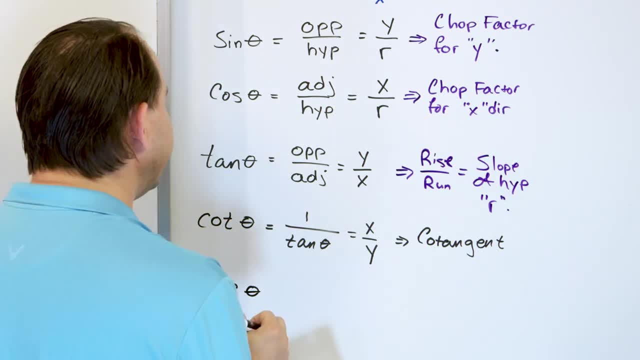 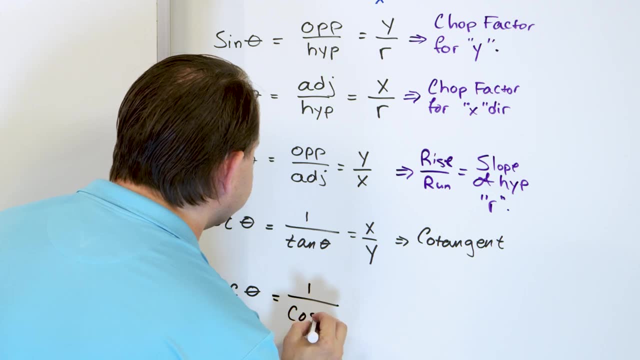 We call it sec of theta. And what is the secant equal to? Well, if the cotangent was 1 over the tangent, the secant is 1 over the cosine of theta. So you see, once you know what the cosine is. 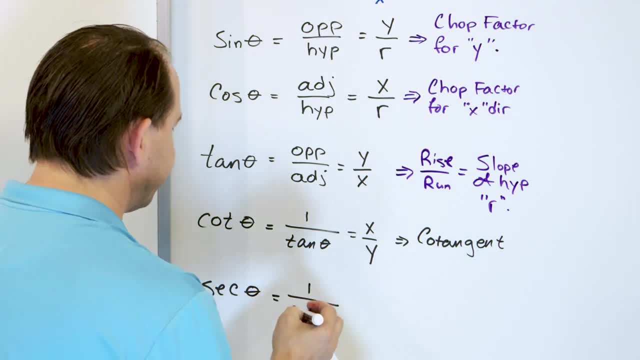 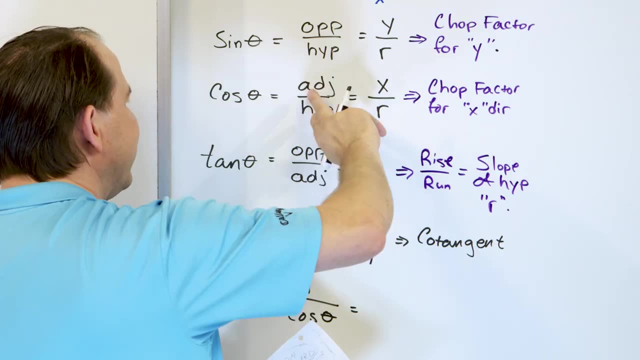 you take 1 over that number and you get something that we call the secant. But since, when we go up to the cosine, the cosine was adjacent over hypotenuse. So if we do 1 over this, this is going to get flipped over. 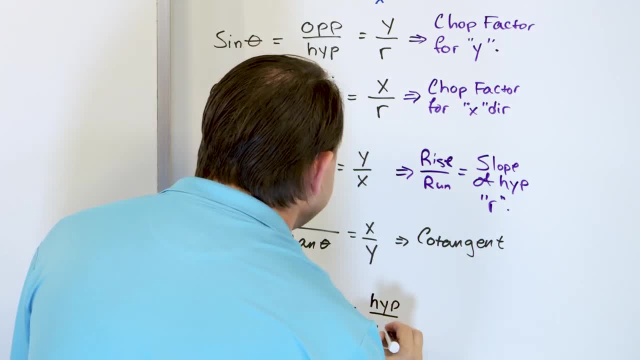 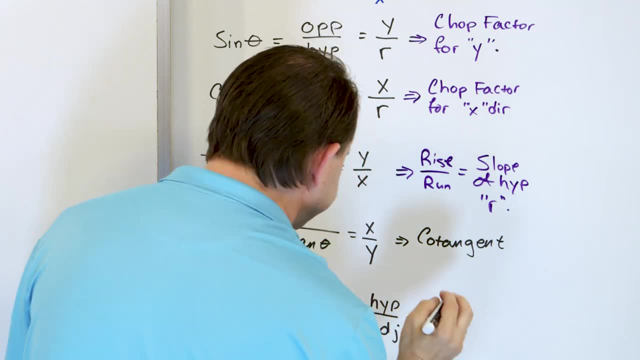 So it's going to be the hypotenuse over the adjacent side. So again, x over r. if we would do 1 over that and flip it over, it would be It would be r over x. Now a lot of students try to remember these things. 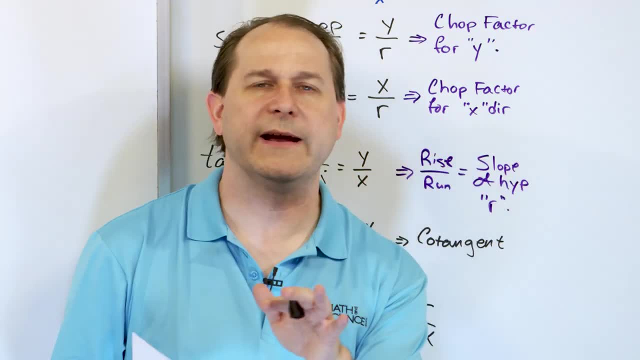 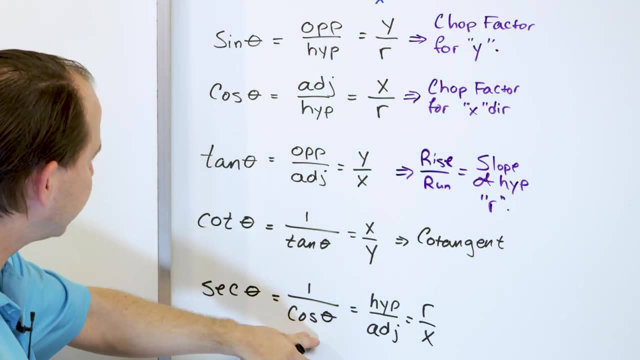 Oh, the secant of theta is hypotenuse over adjacent, It's r over x. It's so confusing You don't need to remember any of that. All you need to remember is the first two of these things, because if I tell you, the secant is 1 over the cosine. 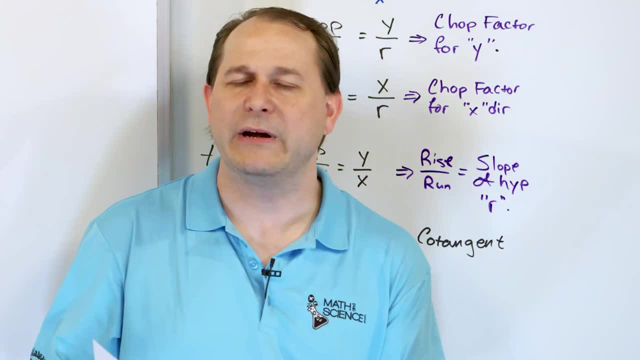 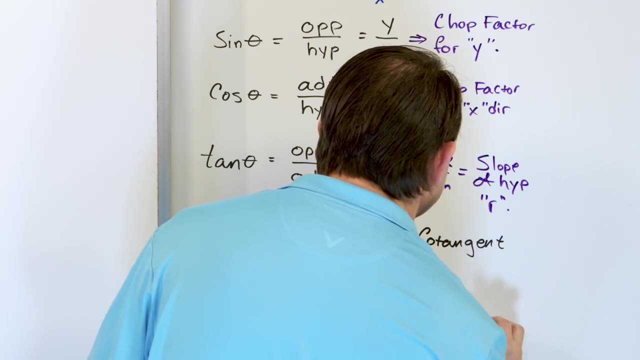 then you already have remembered what the cosine is. You don't have to remember anything new. It's just 1 over that And this thing is called the secant, like this: The last one I want to write down is called the cosecant. 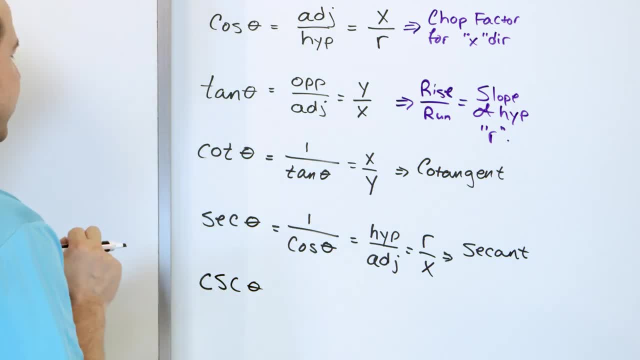 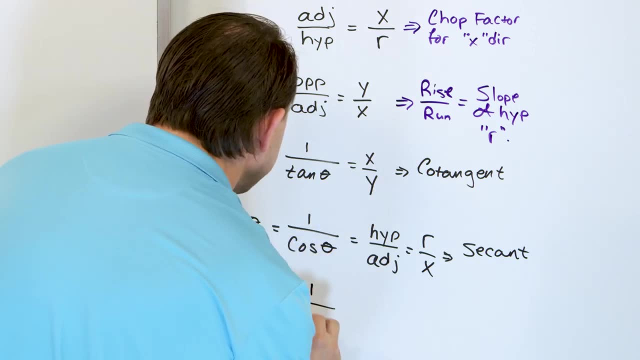 which is C-S-C of theta. C-S-C means cosecant And you might guess if this was 1 over tangent. this is 1 over cosine. then the cosecant is 1 over the sine of theta, like this: 1 over the sine. 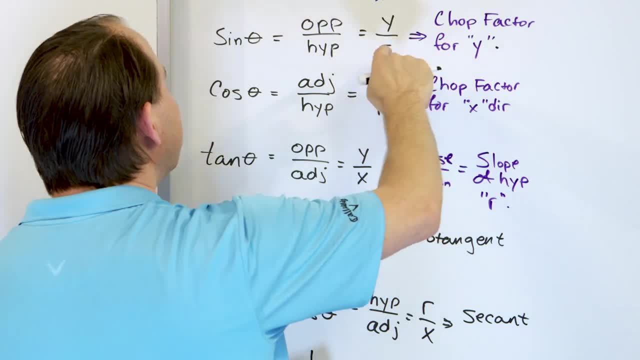 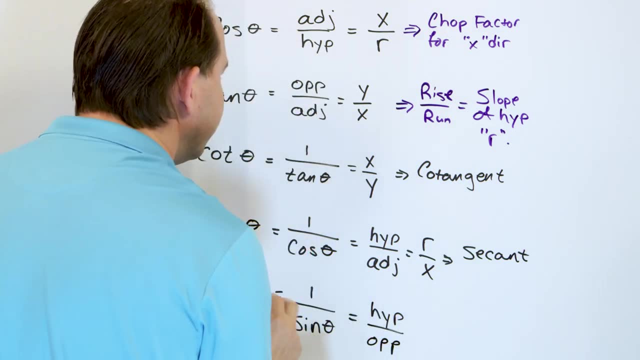 And since the sine of theta was opposite, over hypotenuse, which is y over x, if you do 1 over those things, then what you get is the hypotenuse over the opposite side. just divide those. exactly the same thing as r over x. 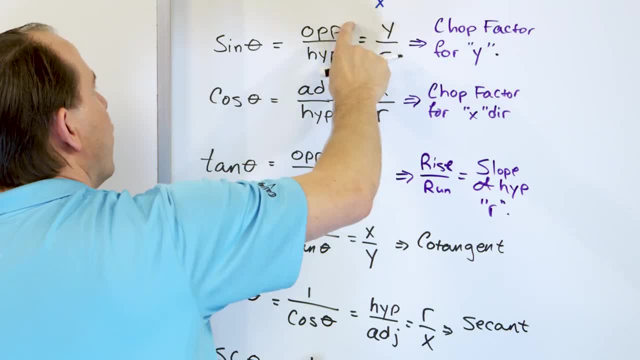 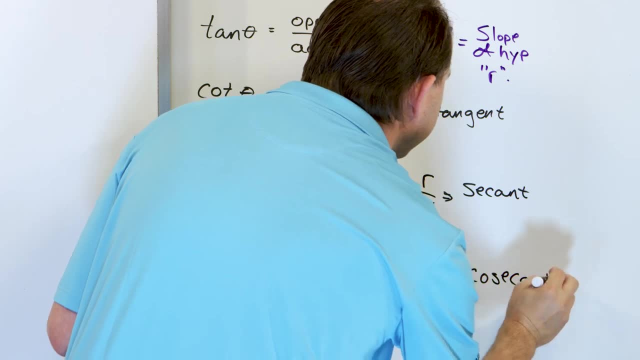 Over y, So do 1 over. this means you flip it over 1 over. this means you flip it over right. And how do you spell it? You spell it as cosecant. all right, cosecant. Now, before I go any farther, I want. 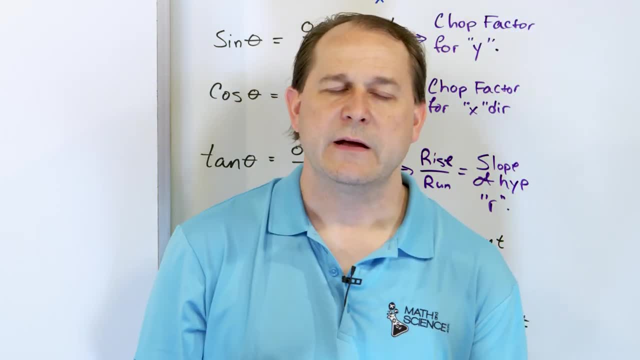 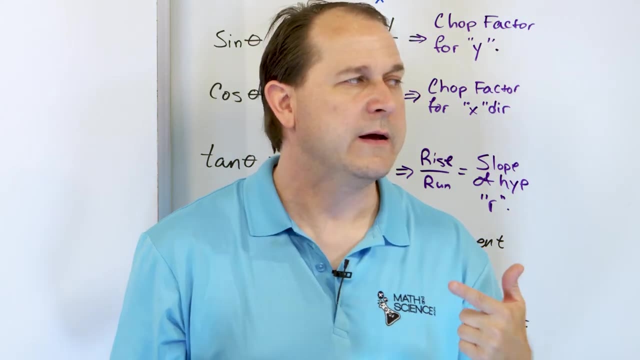 to tell you an easy way to remember all these and how they're related to one another. The most fundamental equations here are sine and cosine. Those are the most fundamental ones that we have to learn, and I devoted an entire lesson to it. All right. 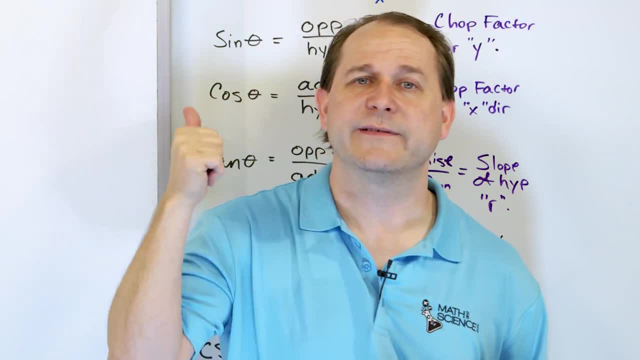 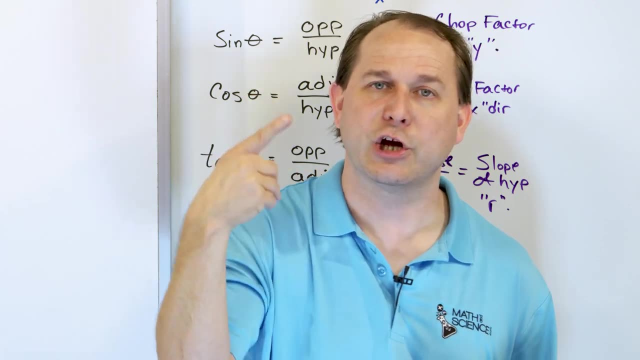 So the way you need to remember these things, I want you to remember them in this sequence: Sine cosine tangent, cotangent, secant, cosecant. Say it one more time: Sine cosine, tangent, cotangent, secant, cosecant. 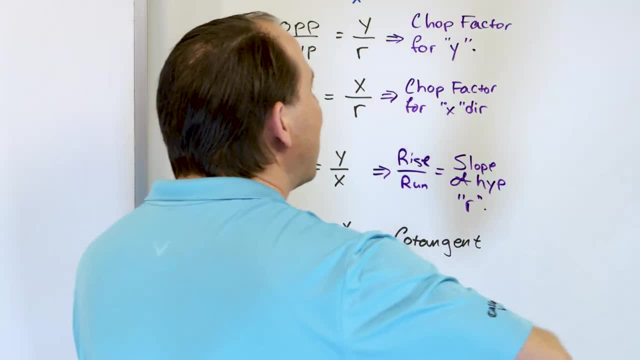 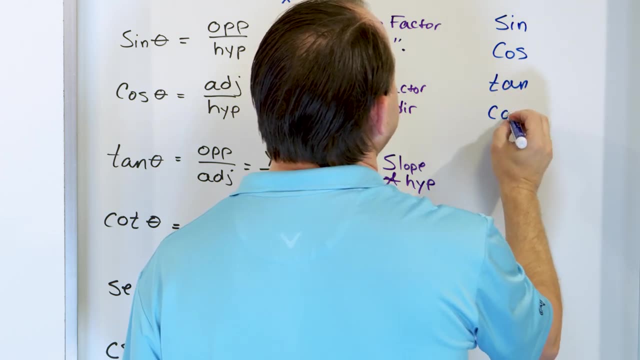 Remember them in that order. This is the reason why, Because if I write them down, then what I'll have is sine, then cosine, then tangent, then cotangent, because that comes right after the tangent, then secant, then cosecant. 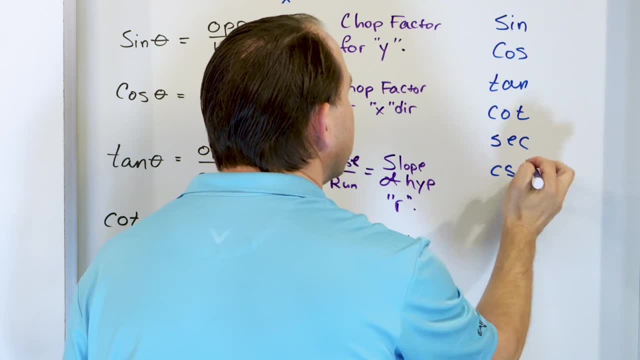 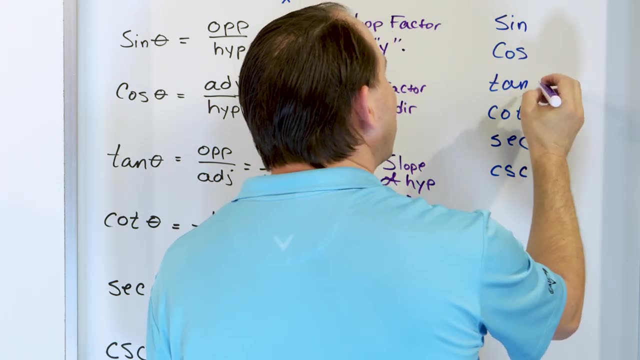 I want you to remember this order, Because here is the reason why, When you write them down in this order, I can draw like a little rainbow kind of thing. Connect the tangent to the cotangent. Connect the cosine to the secant. 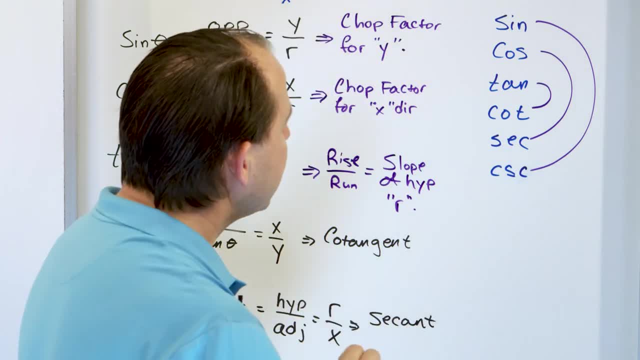 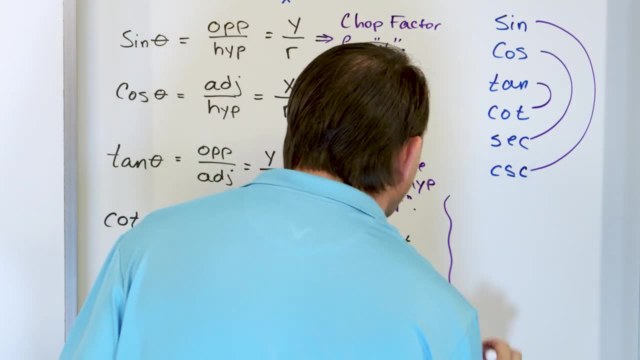 Connect the sine to the cosecant like this. I call it the trig rainbow, if you want to, And what that tells me, what it tells us? I'm going to draw a little dividing line so I don't get in the way here. 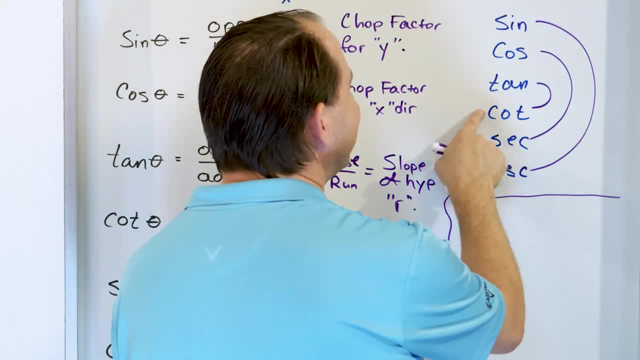 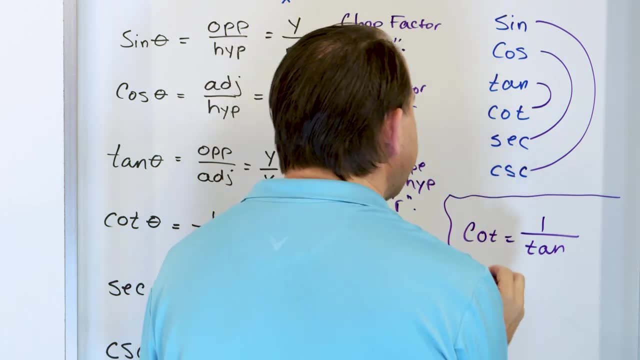 Without memorizing this entire thing, what it tells me is that the cotangent is 1 over 1.5.. All right, It tells me that the secant is 1 over the tangent. Cotangent is 1 over tangent. It tells me that the secant is 1 over the cosine. 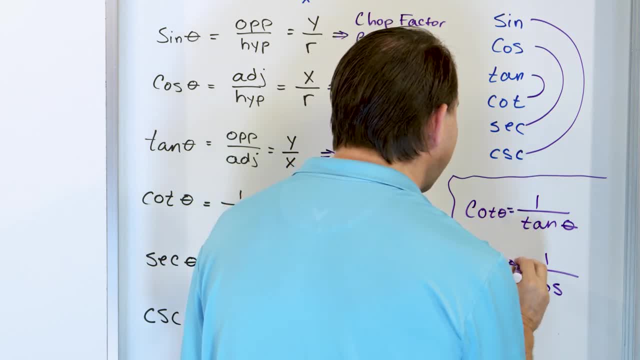 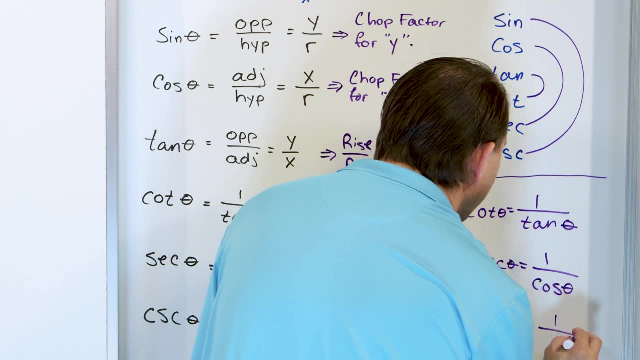 And by the way, when I say cotangent, I mean cotangent of some angle, secant of some angle, cosine of some angle And then cosecant. what do you think that's going to be equal to? Cosecant of some angle? is 1 over sine of the same exact angle? 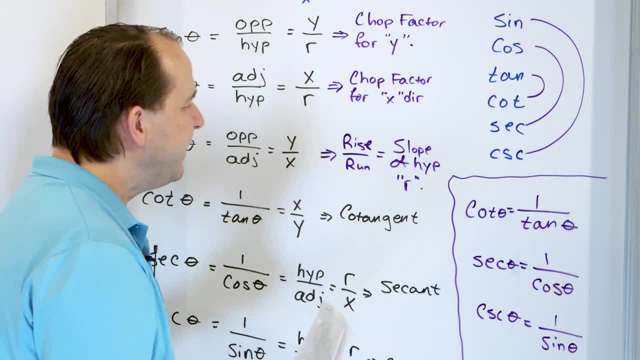 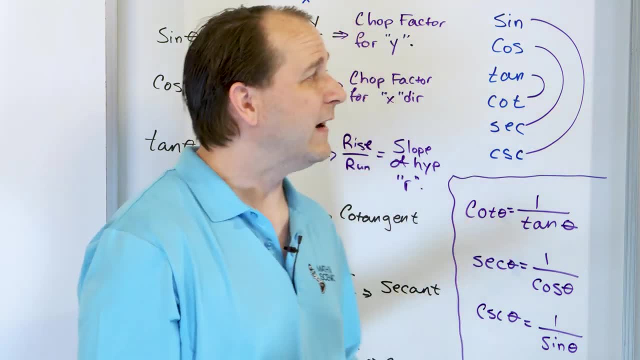 Secant is 1 over cosine. Cotangent is 1 over tangent. These are your very first introduction to trig identities. I don't really like introducing them so early, but we have to introduce them early, Otherwise students are going to try to memorize this chart. 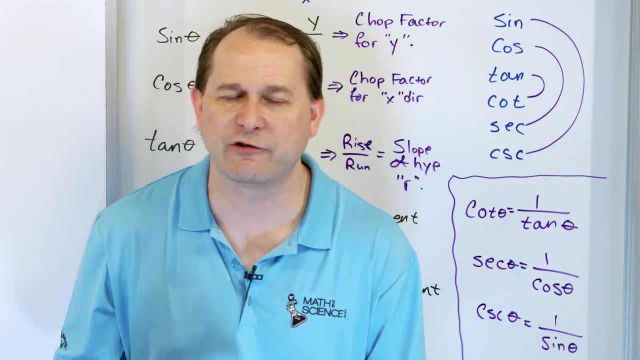 And I think it's a tremendous waste of time to memorize that chart. You don't need to memorize the chart. I'm just putting it here because you're going to see it in your book And I want you to know that I'm covering everything. 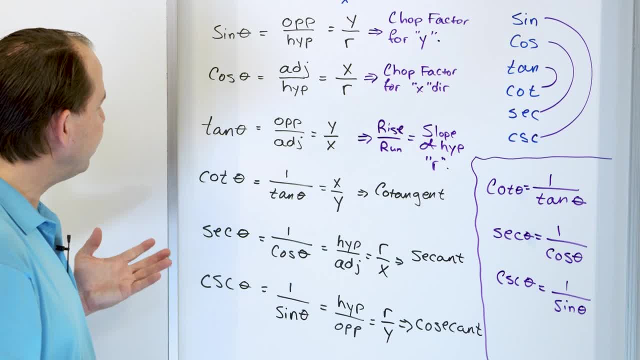 But you don't need to remember that the cotangent is x over y. You do not need to remember that the secant is r over x. You don't need to remember that the cosecant is r over x. All right, It's r over y. 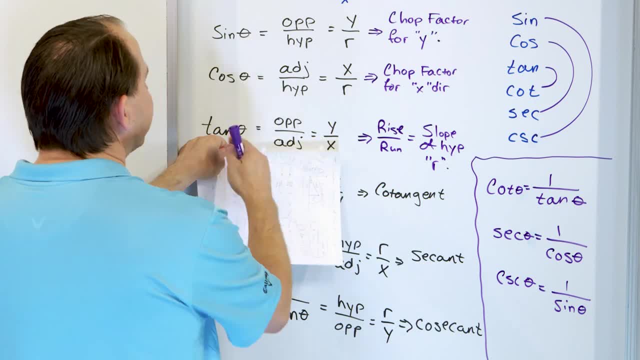 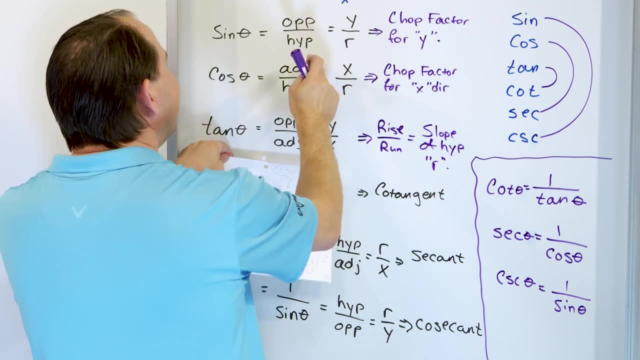 You don't need to remember any of that. All I really want you to remember, at most, is the first three. Sine is y over r, opposite over hypotenuse. Cosine is x over r, which is the adjacent over the hypotenuse. 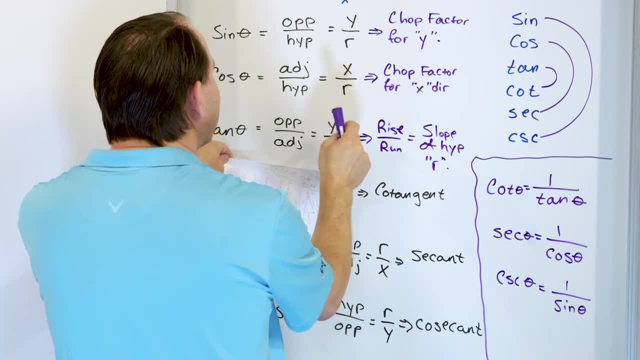 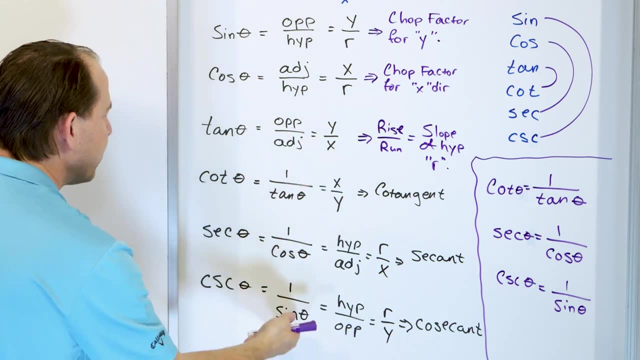 Tangent is the slope of the line. You can remember that because it's the slope. y over x are opposite over adjacent, But all of these other ones is just 1 over tangent, 1 over cosine, 1 over sine. A lot of students try to memorize these. 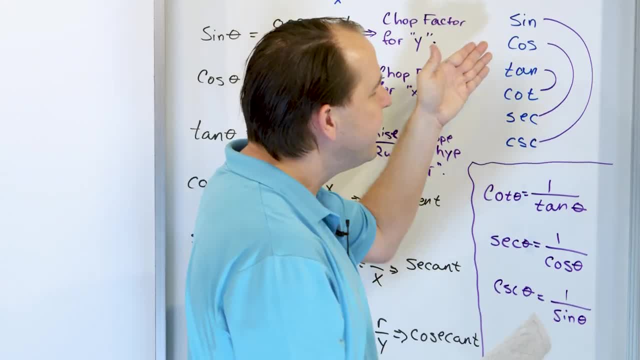 but you don't need to remember it because if you just put it down in the correct order, then you have always you remember exactly what you're doing, Exactly You can draw it and you can see Cotangent is 1 over tangent. 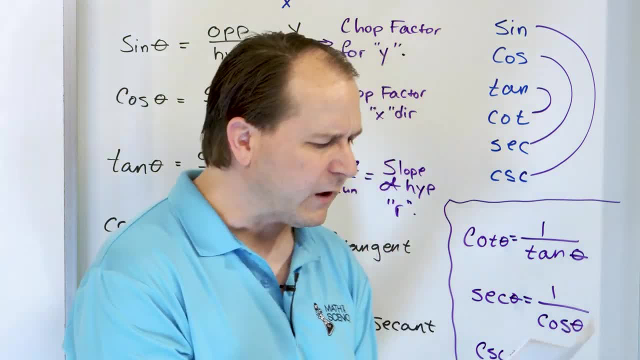 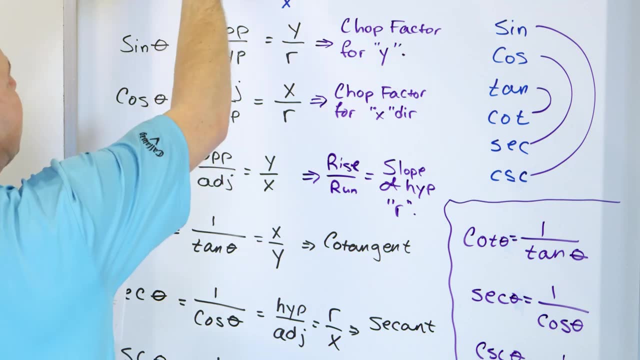 Secant is 1 over cosine, Cosecant is 1 over sine. All right, A couple of notes I want to go through. We said that sine is the chop factor for y, which means the projection of this hypotenuse in the y direction. 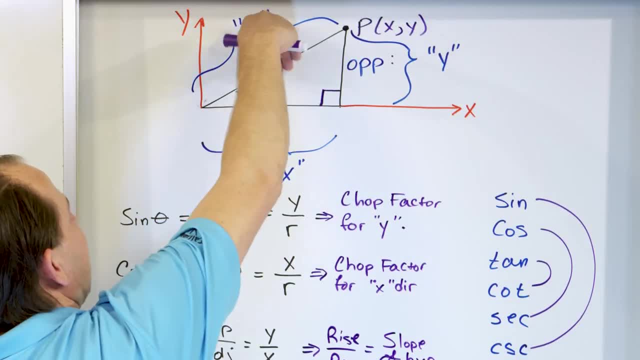 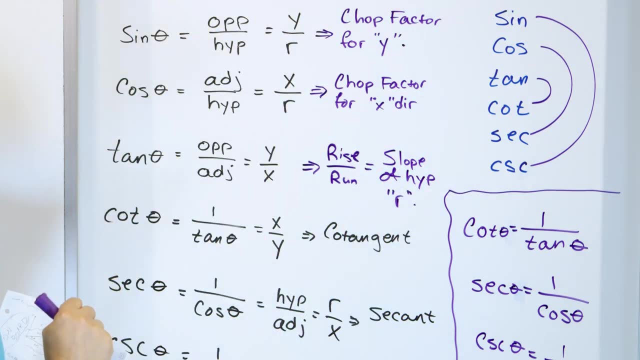 Cosine is the chop factor for x. Another way to think of it is the projection of the hypotenuse in the x direction. Tangent means rise over run, which is the slope of this hypotenuse, of this triangle. Cotangent is 1 over x. 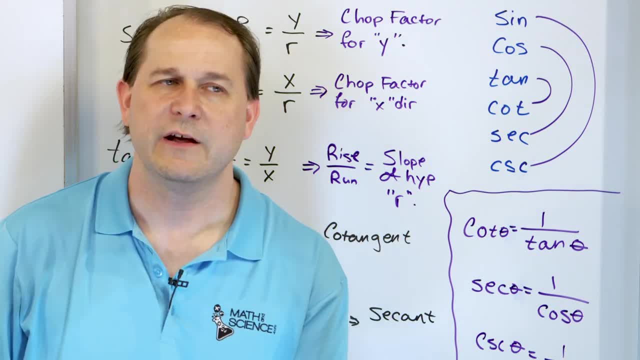 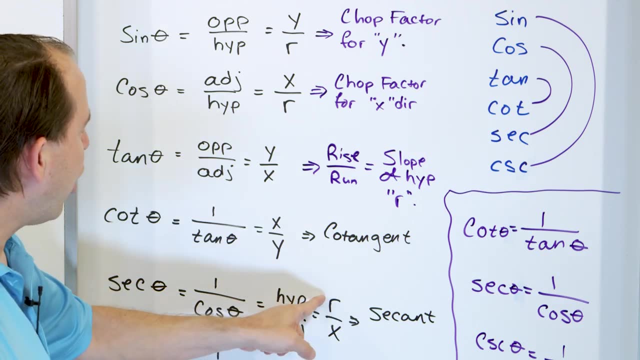 Run over the tangent. it's literally the opposite of the slope calculation, just defined differently as run over rise. That's all it means. And then, when you look at secant and realize that it's r over x, all it's telling you. 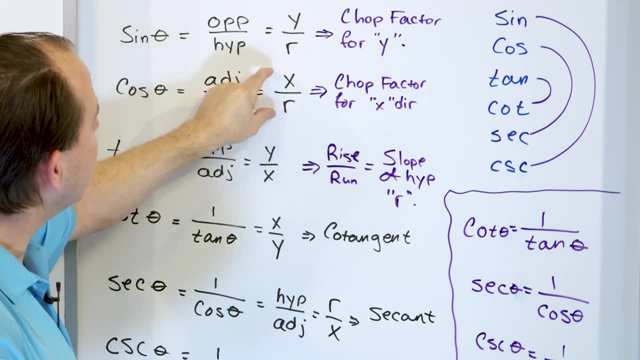 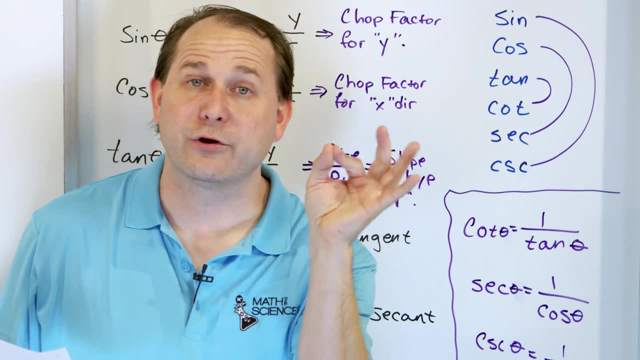 instead of x over r being the ratio of the x direction to the hypotenuse, the secant here is r over x. When you take the hypotenuse, which is a bigger number, and you divide by x, it's just telling you how many x parts. 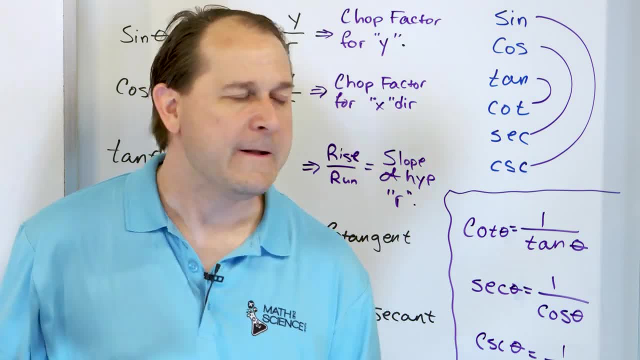 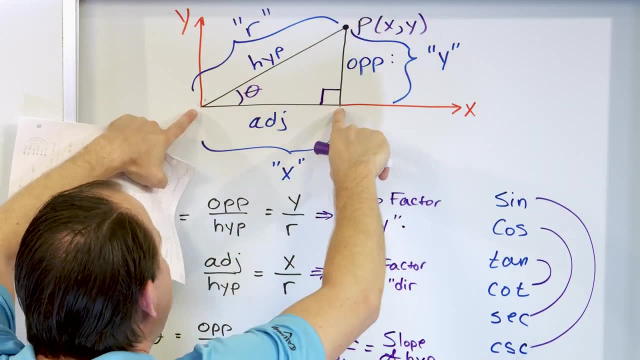 how many adjacent sides of the triangle fit into the hypotenuse. That is what a secant is. It's basically telling me I'm going to take the hypotenuse r and I'm going to divide by x How many x directions, how many of these adjacent sides? 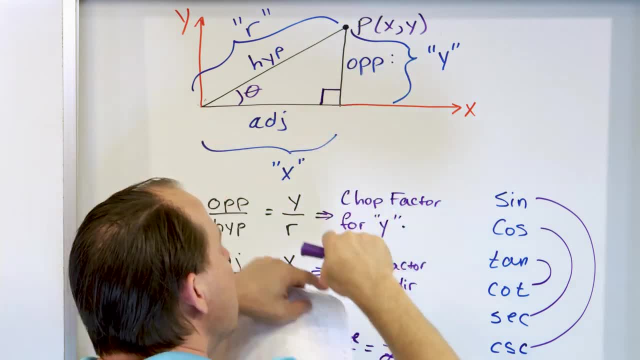 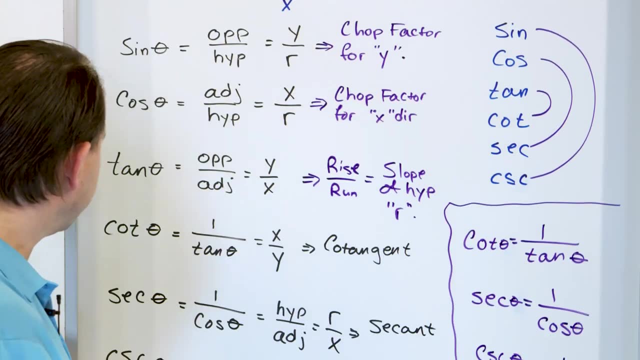 fit in there? Is it 1.2? Because this is longer? Is it like 1.2 of these lengths of this triangle can fit, or more or less? And when you have the cosecant it's just the hypotenuse? 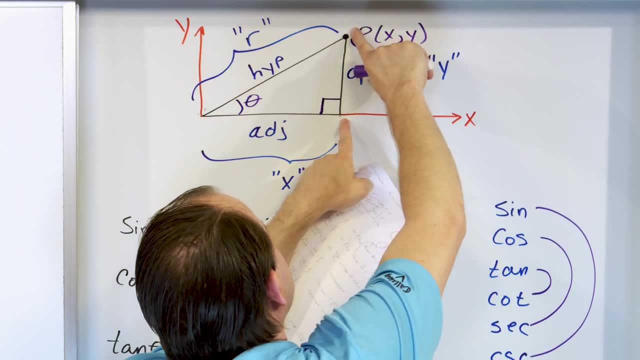 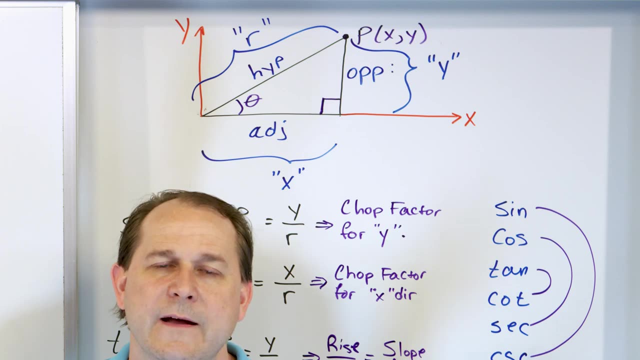 divided by the y direction. How many of these y distances can fit in one of those hypotenuses? So the secant and the cosecant are just flipped upside down sines and cosines, which means they're telling you how many of those adjacent and opposite sides. 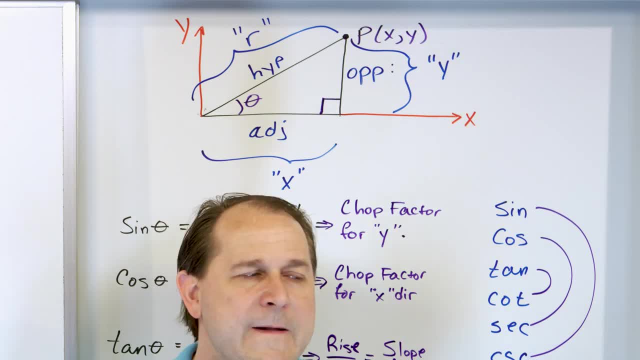 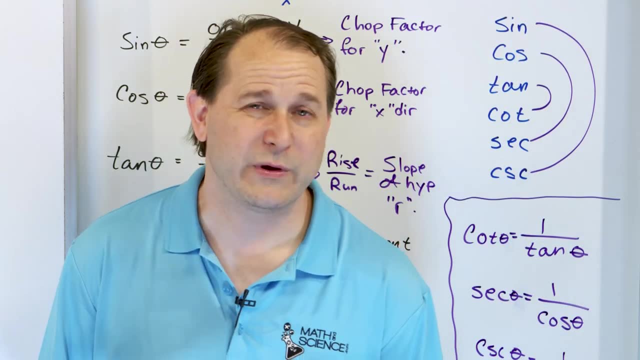 fit into in terms of division, fit into the hypotenuse, But the deeper reason, or the deeper understanding is: why do we even need cotangent, secant and cosecant? The real reason we have them defined is because, when you get farther down the road, 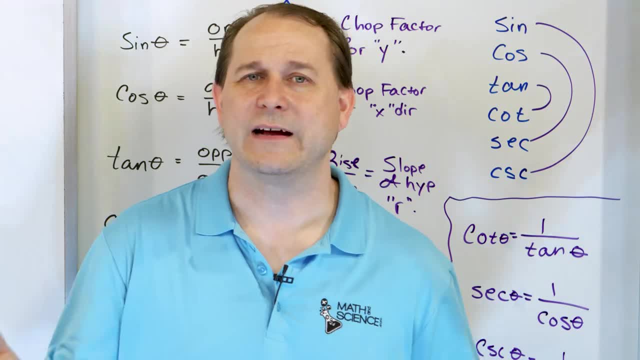 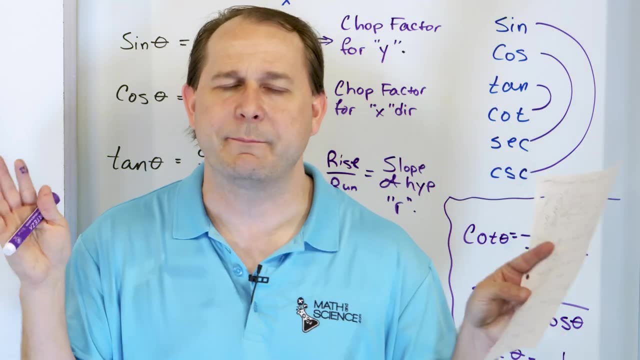 you're going to be writing equations, lots of equations that involve sines and cosines. I mean they pop up everywhere, in every branch of science: math, engineering, physics, chemistry, I can go on and on Every branch. they pop up everywhere. 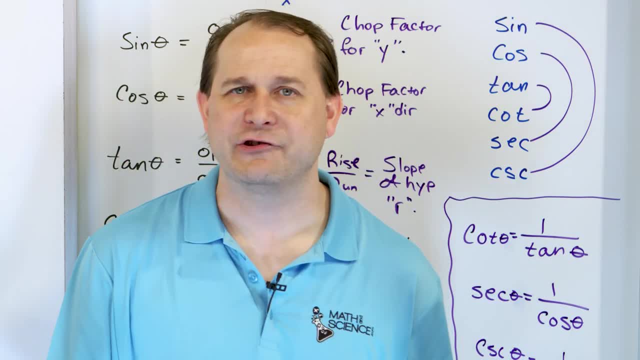 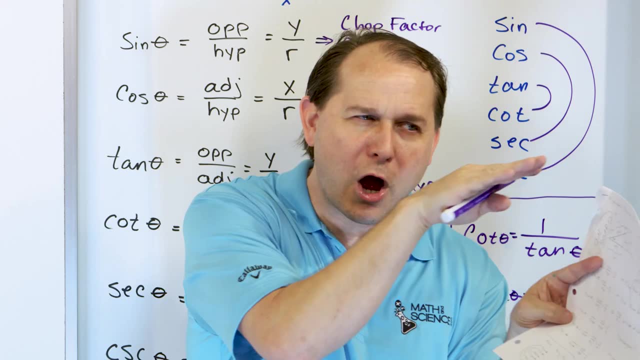 So what happens if you have the sine in the denominator of a fraction? Well, you could leave the sine in the denominator of a fraction. What if you have a cosine function in the denominator on the bottom of a fraction? Like you just manipulate some equation. 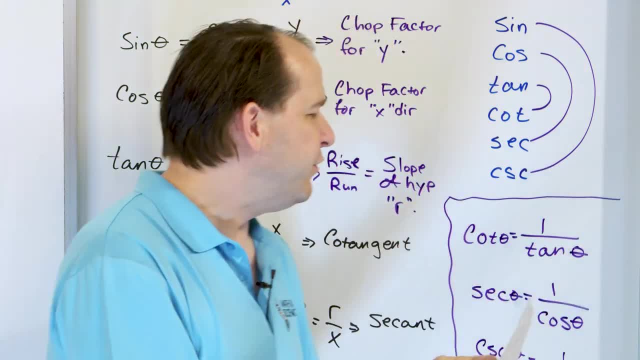 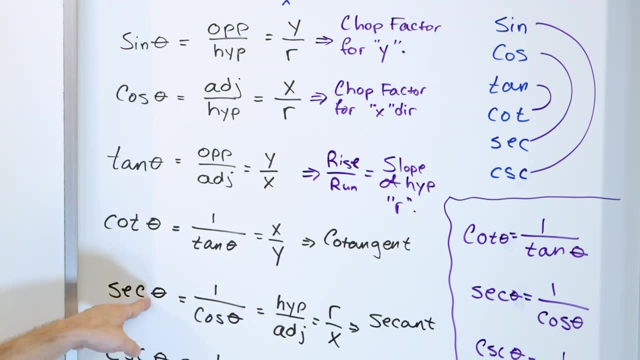 and you get it on the bottom there. What do you do? Well, you could leave it there, But then you could also, if you want to take a little shortcut here, call it. if the cosine's in the bottom, we'll just write the whole thing in terms of a secant function. 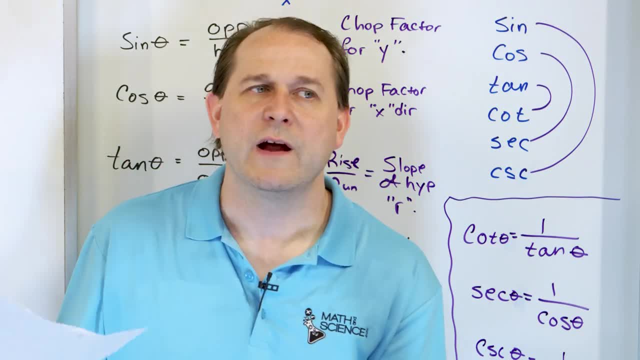 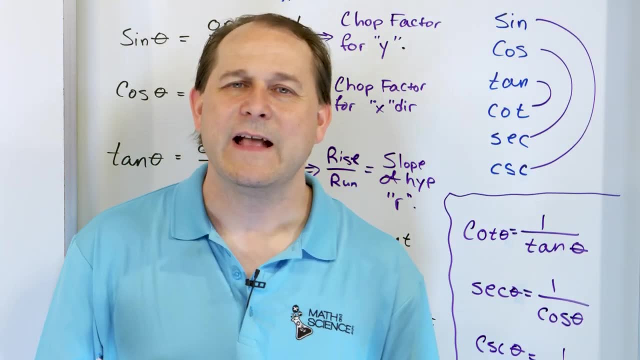 If the sine ends up in the bottom of some fraction somewhere, instead of leaving that ugly fraction there, we'll just write it as a cosecant. So the reason we have the cotangents and the cosecants and the secants is really because sometimes those trig 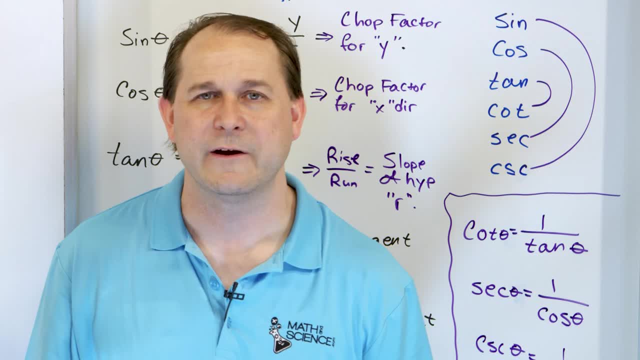 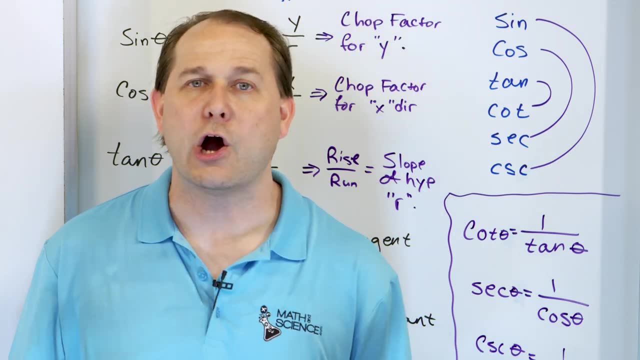 functions end up on the bottom of fractions when you solve equations later, And instead of leaving it like that, we have different names, so we can get rid of all the fractions and call them secants and cosecants. That's why I'm trying to harp on the idea. 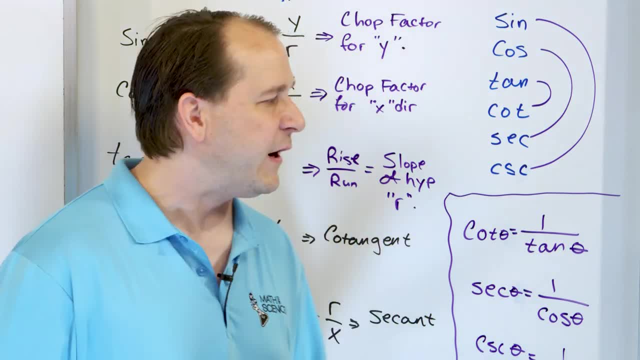 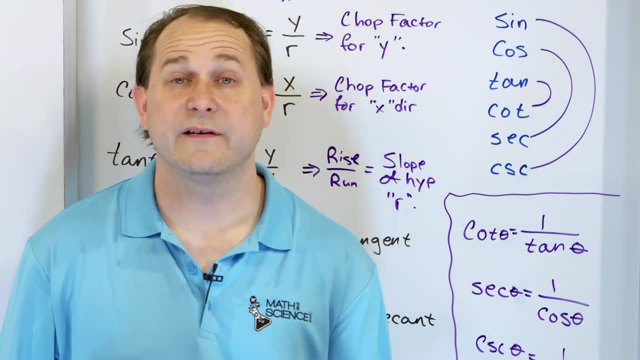 that cosecants and secants and cotangents are not that important. They come from everything, above All right Now that we have introduced what these are. we've done tons of talking. we need to solve some problems. We're going to solve a couple of problems here. 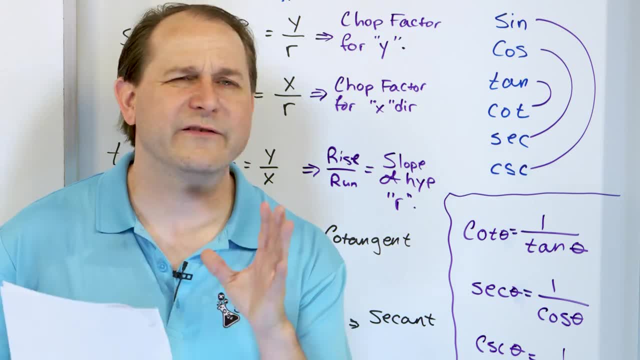 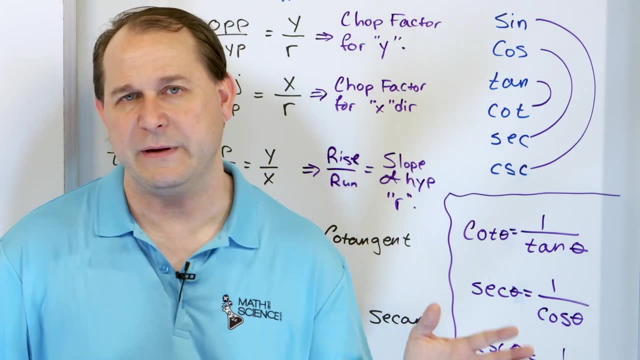 And then over the next several lessons we're going to be solving tons so many problems like this that you're going to get bored doing them. But I really want you to do all of them, Because this stuff does not come naturally to most people. 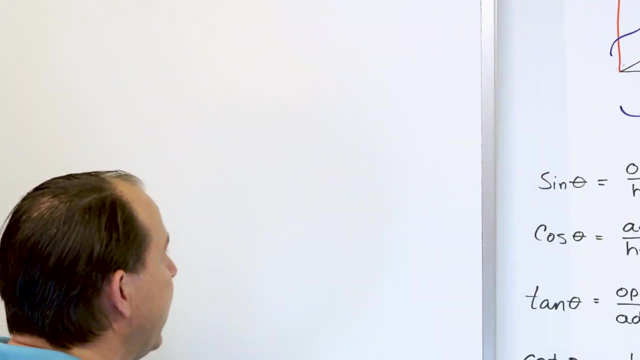 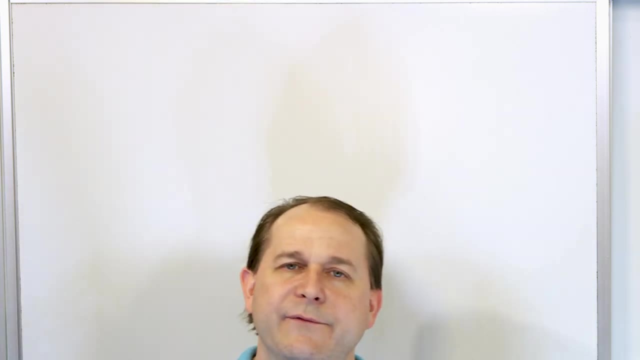 You have to work a ton of problems, And that's what we're going to do. So let's go ahead and start and solve our very first problem. All right, The problem is very simple. I'm going to give you a triangle and I 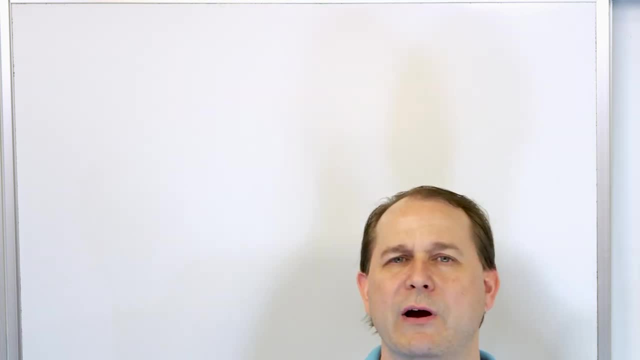 want you to calculate the sine, That's six trigonometric functions. If you ever see a problem that says find the six trig functions, what they want is here we go: sine, cosine, tangent, cotangent, secant, cosecant. 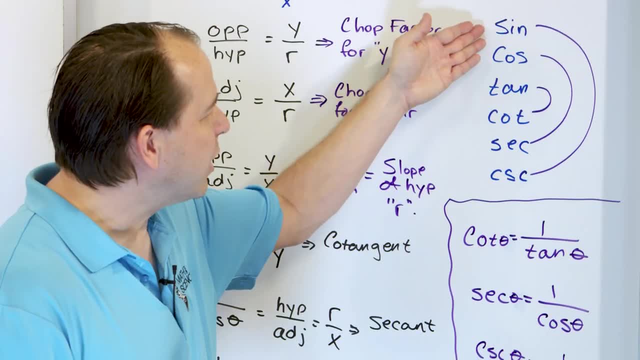 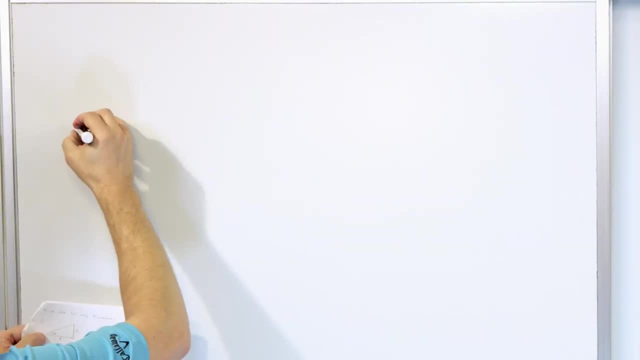 I want you to do them in that order, Because if you remember that order, then you'll automatically remember these identities down here without having to memorize anything. So what do we do? The first problem goes like this: Here's a triangle. 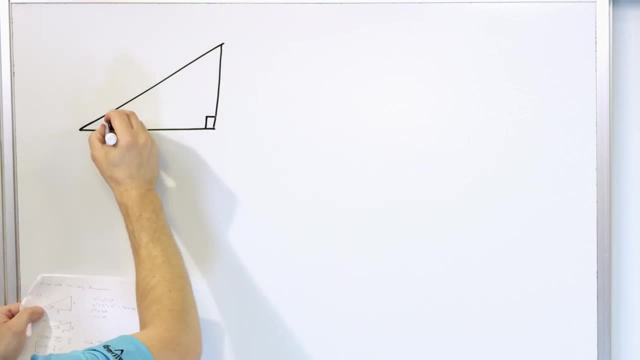 We're going to get very, very, very comfortable with drawing triangles in this class. There's some angle theta right here which I kind of bought. Sorry about that. Some angle theta right here. This side has a length of eight and this side 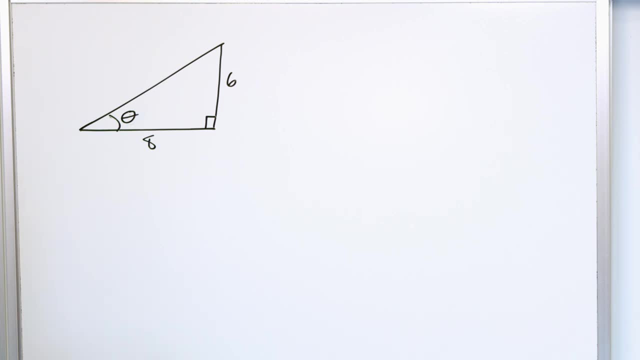 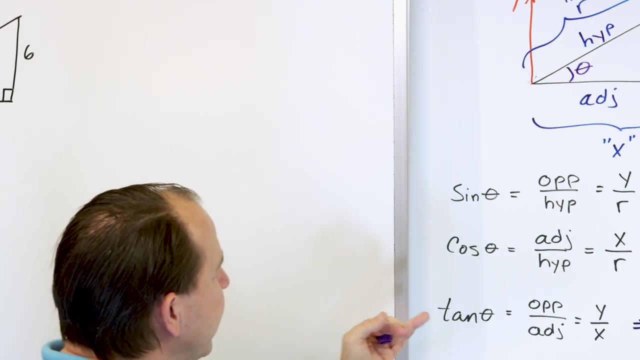 has a length of six. And the question is: I want you to write all six trigonometric functions of the angle theta in this drawing here. How do we do that? Well, we know from experience that sine is going to be opposite over hypotenuse. 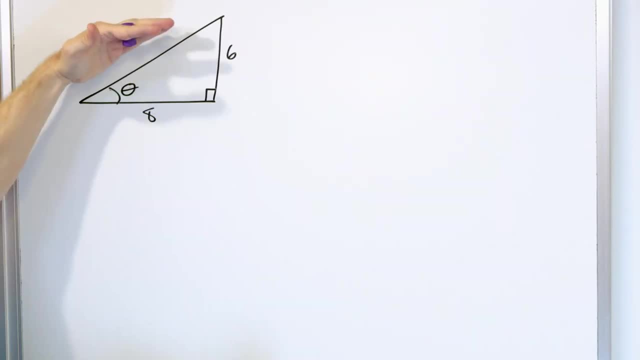 and cosine is going to be adjacent over hypotenuse, But in our drawing we were not given the hypotenuse, So a lot of students would look at that and say, well, how do I do it? I don't have a hypotenuse. 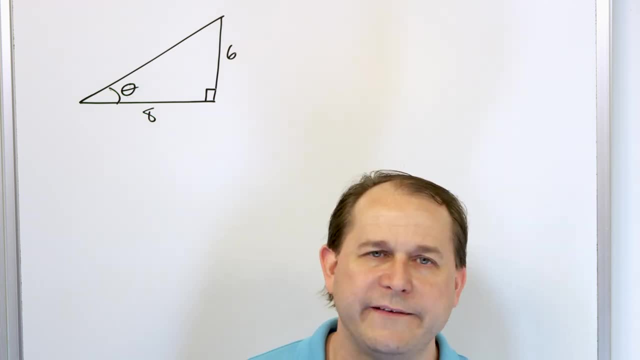 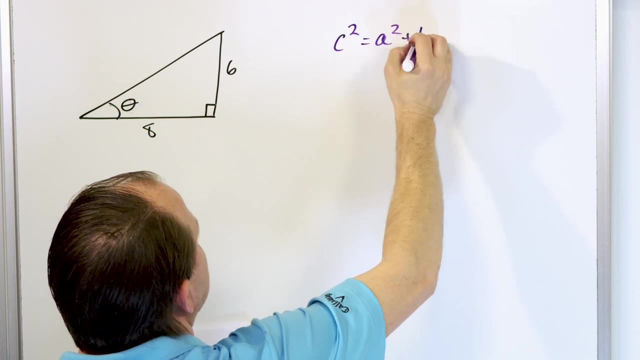 But all of these are right triangles, So the Pythagorean theorem always applies. So if you don't have the hypotenuse, you have to figure it out yourself. c squared is a squared plus b squared. Now I'm calling this c. 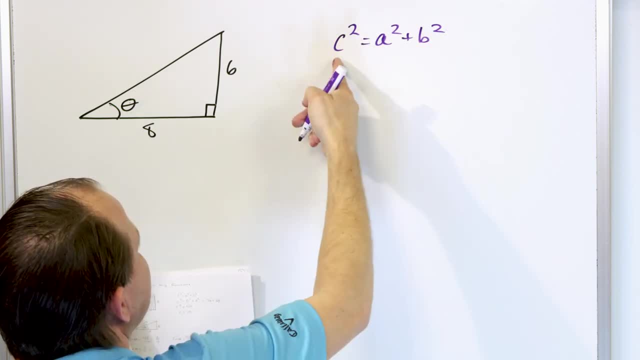 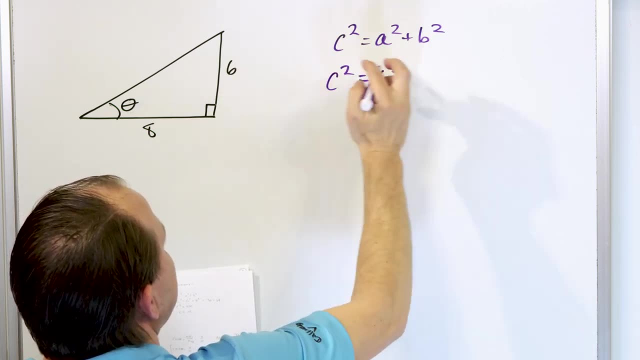 I know over there I called it r. I mean, you have to work with me here. So the Pythagorean theorem is always written like this. So we say c squared is here, we go with 6 squared, this side squared, plus 8 squared. 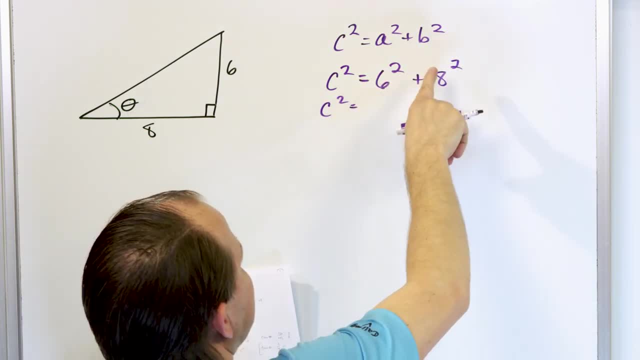 So c squared, when you do 6 times 6 is 36, and then 8 times 8 is 64, and add them together you're going to get 100.. And so the distance there you take, the square root. 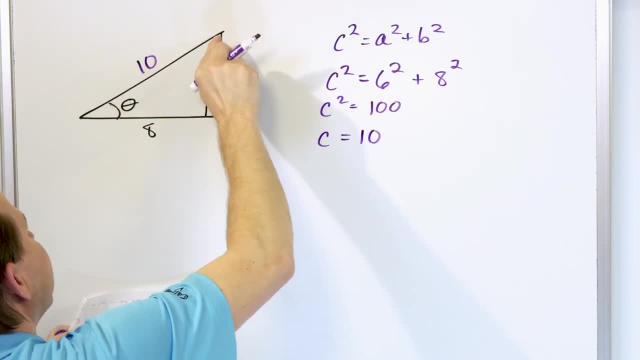 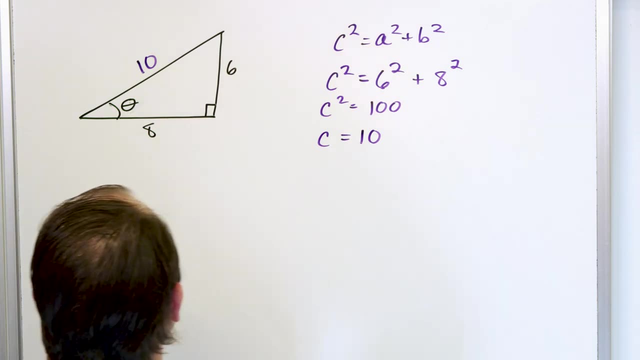 of both sides, you get 10.. That means that the length of this hypotenuse of the triangle is actually 10.. We know that that's true because we can always use the Pythagorean theorem to find the lengths of the other sides of a right triangle. 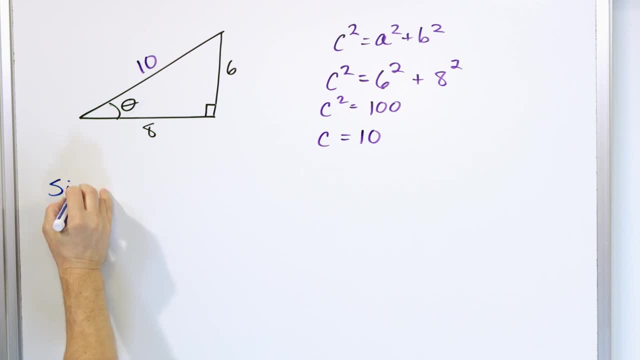 Now we have to find the six trig functions. Here we go. The sine of the angle is the opposite side of this angle. over the hypotenuse, The opposite side is in the y direction, of course, because it's y and the value of it over there is 6.. 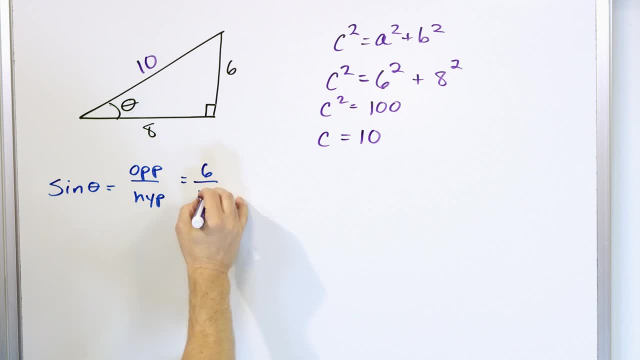 So we get 10.. So we can look at the y direction and we can say that this angle is 3.5.. So we get 10 divided by the hypotenuse. The hypotenuse is 10.. So the answer is 6 over 10.. 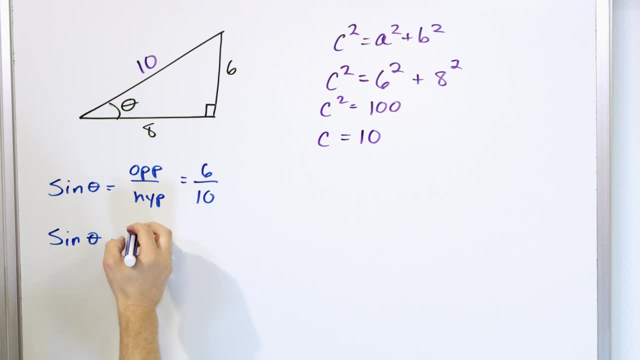 But that's a fraction. So what we can really say is that the sine of the angle, and we divide here by 2, and we divide by 2,, 6 divided by 2 is 3.. 10 divided by 2 is 5, so we get 3 fifths. 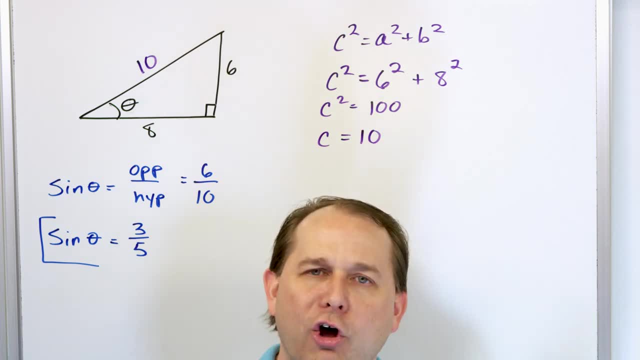 So the sine of this angle is 3 fifths. What is it telling me? It's telling me that the ratio of how tall the triangle is in the y direction compared to the length of the hypotenuse is 3 tenths. 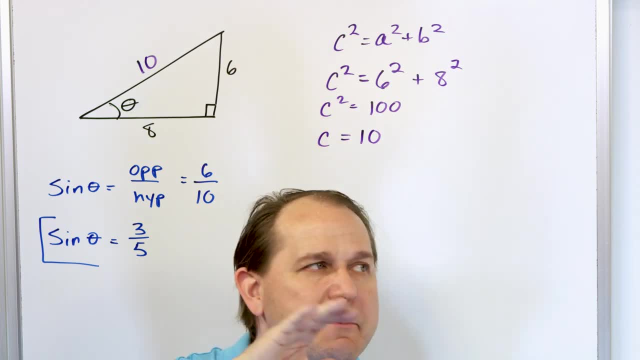 In other words, it doesn't go up very high compared to the length of the hypotenuse because it's a pretty small. I guess it's more than half. I said 3 tenths, I'm sorry, 3 fifths. 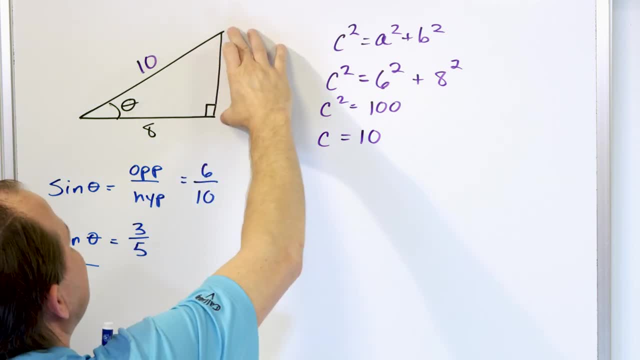 So it's a little bit more than half. So when you look at this triangle you can see- and probably I didn't draw it exactly right- but the ratio of this divided by this is a little bit more than half. In other words, this thing is shorter than this. 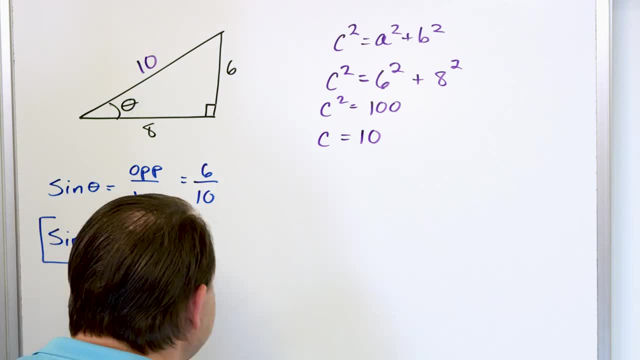 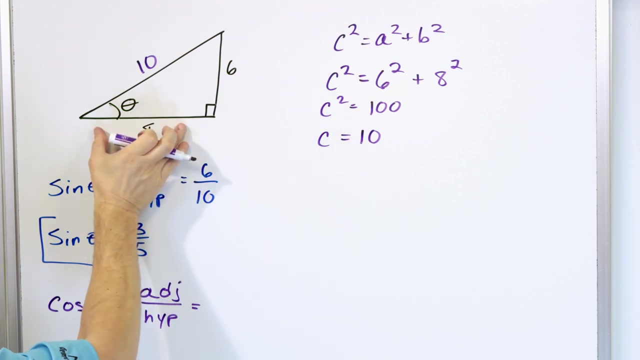 by about a half. a little bit more than a half, All right. So let's go and calculate the next one. So we have cosine of the angle. is the adjacent side divided by the hypotenuse, Adjacent is x, which means the x direction here. 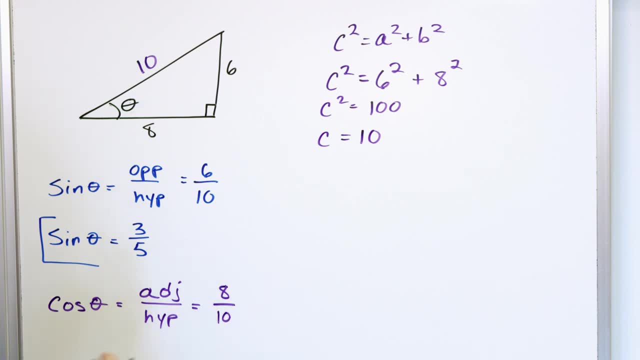 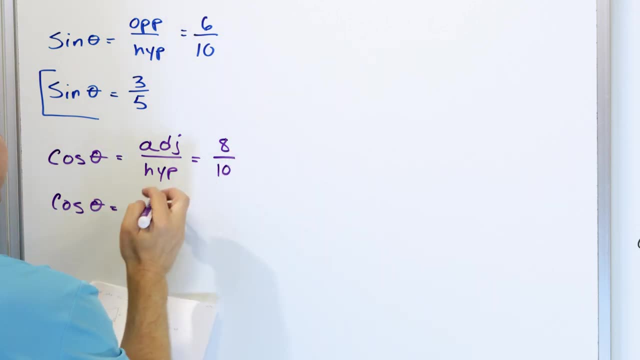 is 8 units over there, and then divide by the same 10.. You're always comparing to the hypotenuse, so 8 over 10. And so what you get is the cosine of the angle. We can divide by 2 and divide by 2.. 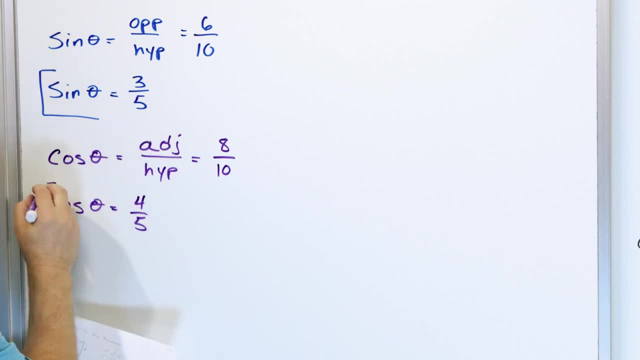 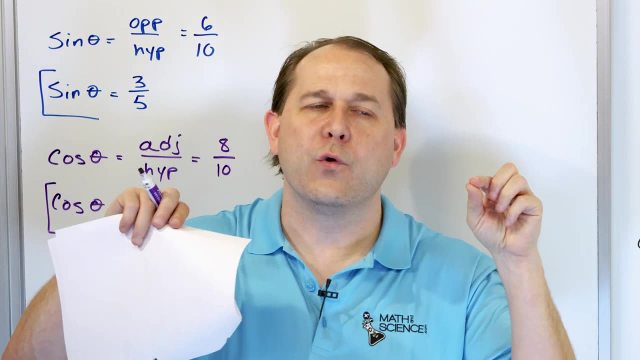 So what we'll get is 4 fifths. So the cosine of the angle is 4 fifths. That's the second trigonometry. So what does this actually mean? It means that the triangle stretches in the x direction 4 units, for well, I shouldn't say 4 units. 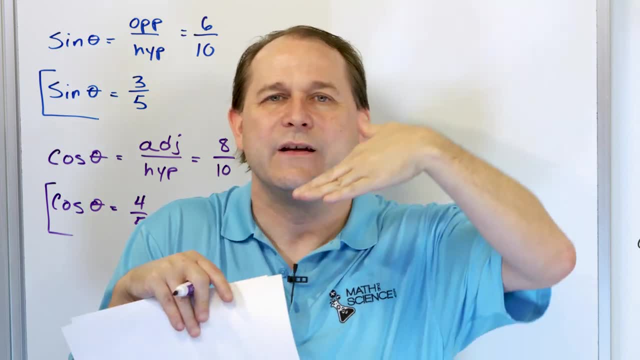 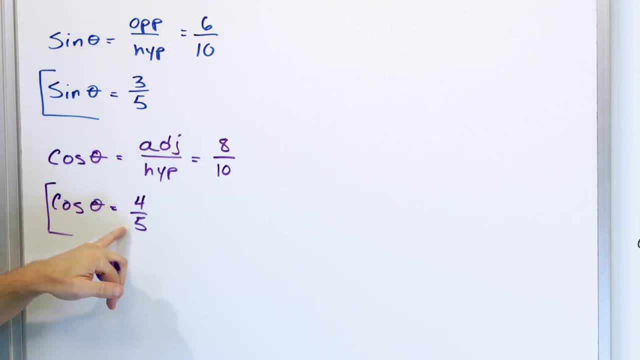 I should say that, compared to the hypotenuse, the ratio of the x to the hypotenuse side is 4 fifths much, much higher than before. So, compared to the hypotenuse, the triangle stretches more in the x direction. 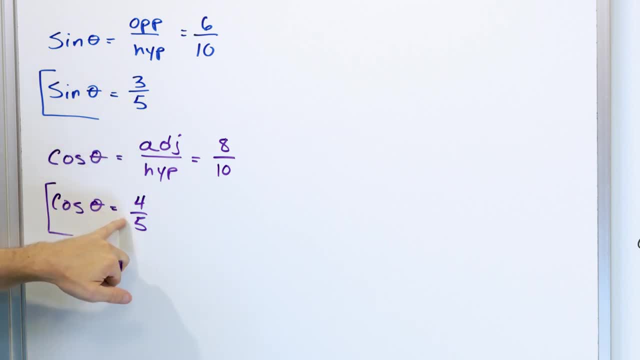 compared to hypotenuse, because this is a number closer to 1 as compared to the sine. All right, So let's go back and calculate the tangent of the angle And let me go back and say that this sine and this cosine, 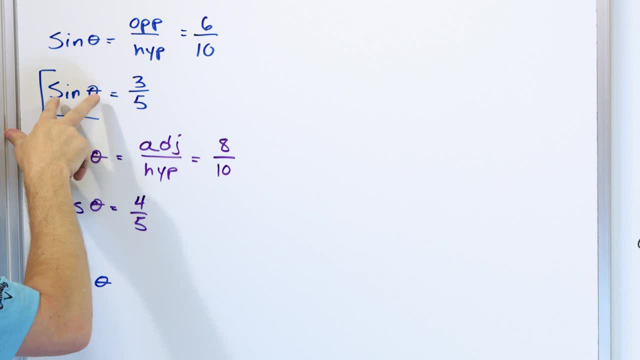 these are the chopping factors, Another way to say it. remember sine goes with y and cosine goes with x. So the chopping factor in the y direction is 3 fifths and the chopping factor in the x direction is 4 fifths. 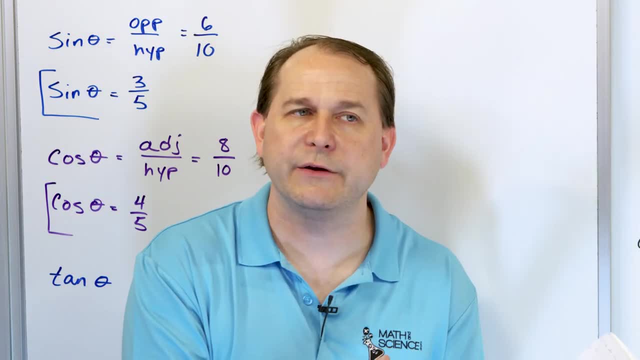 And that means when we take those chopping factors and multiply by the hypotenuse, they tell us the other sides of the triangle. We're going to do a lot more practice with that. We're going to do that in just a minute, All right. 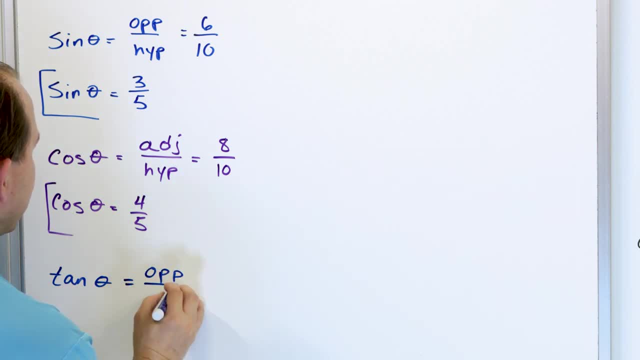 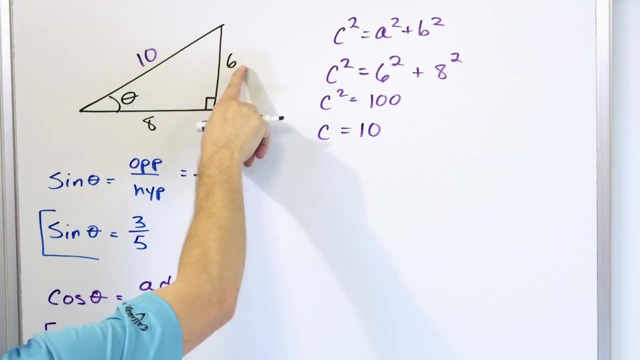 So the tangent of this angle is going to be equal to the opposite side over the adjacent side, which is y over x. which is, what is it equal to here? 6 over 8.. So the opposite side is 6, and then 8.. 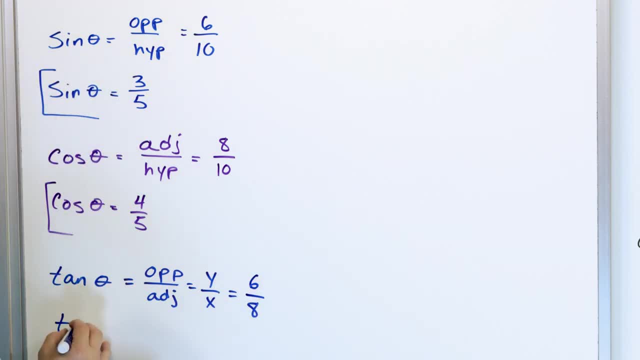 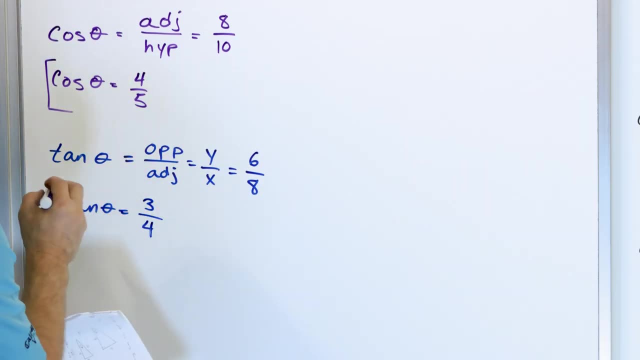 6 for the y direction, 8 for the x direction. So the tangent, when you divide by 2, you're going to get 3 fourths. Let me just check myself: 3 fourths: What is this telling me? 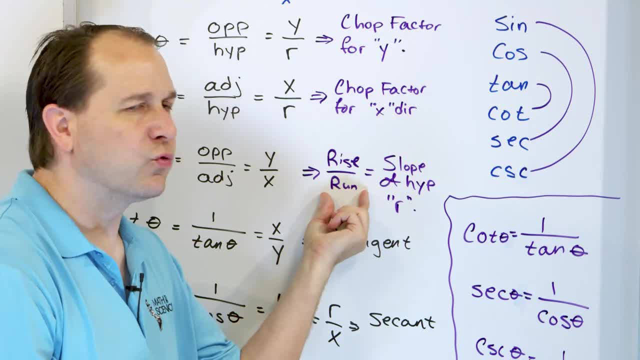 The tangent, remember, is going to be 3 fourths. It's really just another way of telling me rise over run of that triangle hypotenuse. It's the slope of the hypotenuse, So this fraction is literally rise over run. 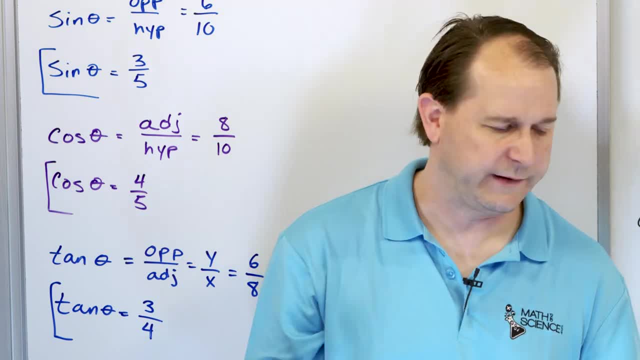 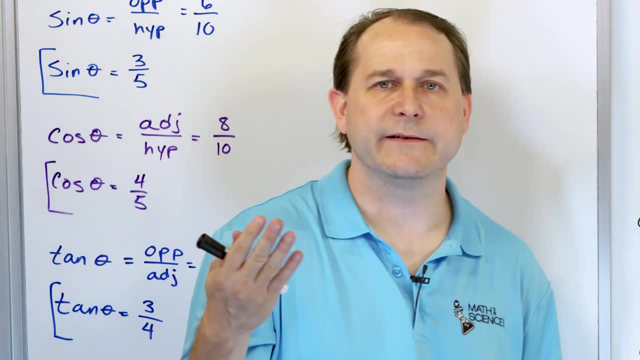 How much does the hypotenuse go up compared to how much does it go over? That's what it's telling me. And then I have to do and ask myself: we've done sine cosine tangent, Now I have to do cotangent, secant and cosecant, right? 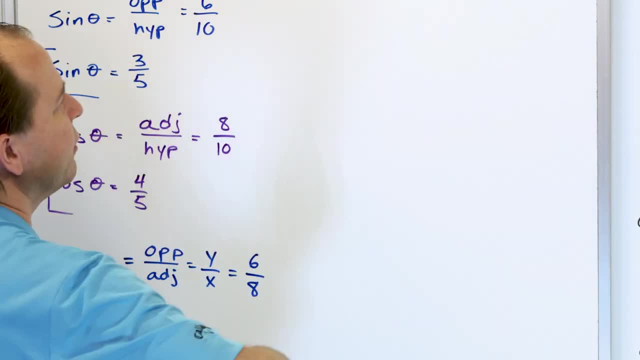 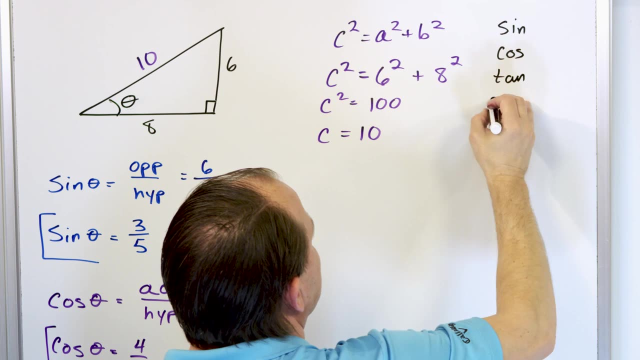 Cotangent, secant and cosecant. Maybe I should go look at that chart. No, you don't need to go look at that chart, Just write it down. We say sine cosine tangent, Cotangent, secant, cosecant. 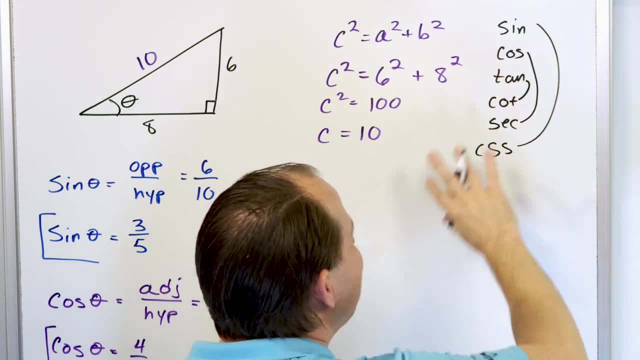 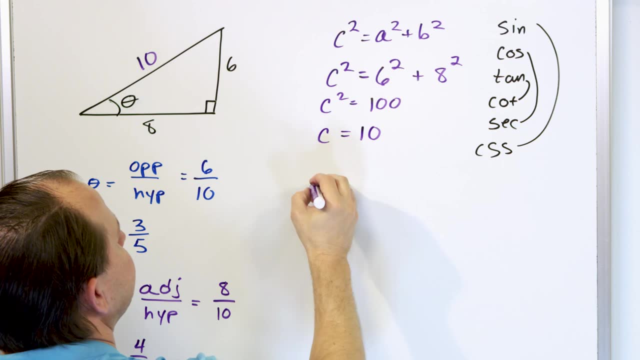 And this one goes with this one, and this one goes with this one, and this one goes with this one. Now you have everything already in place, You don't have to remember anything else. We now know that the cotangent of an angle. 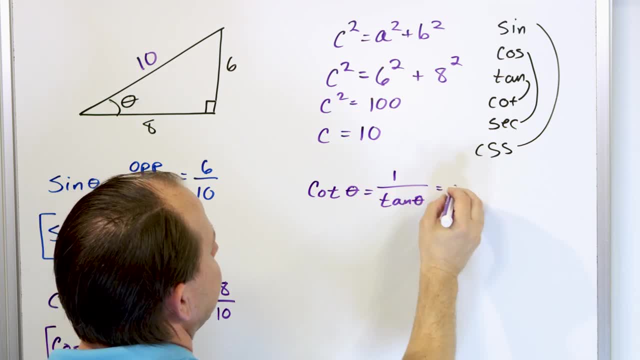 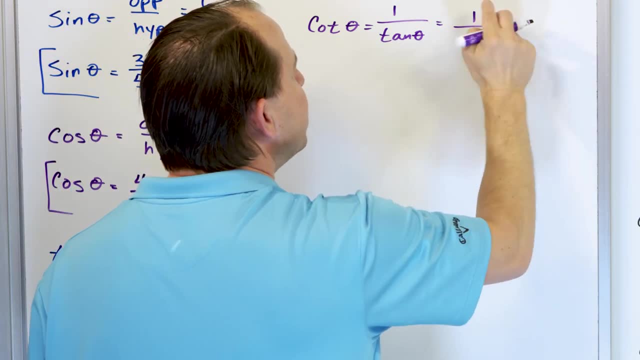 is 1 over the tangent of the angle. But the tangent of the angle, we already know what that is: It's 3 fourths. So we put it down here: It's 3 fourths, which means the numerator is 1 over 1.. 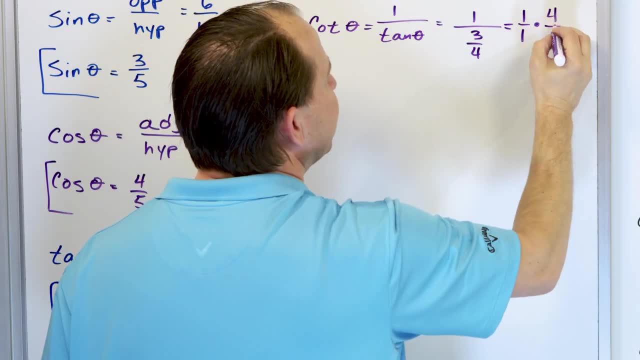 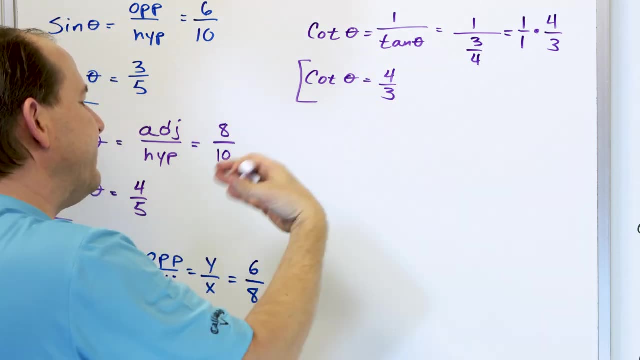 Change this division to multiplication, Flip the fraction over And then the cotangent of the angle is 4 thirds. I told you the cotangent is like a flipped over version of the slope. It's run over rise, This one's rise over run. 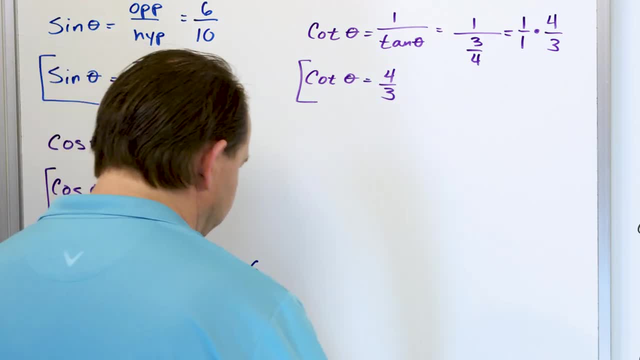 This one's run over rise. That's how it's defined. That's what you have to kind of work with, because that's what it is, All right. so now we have the cotangent, Let's go find what the secant of this angle is. 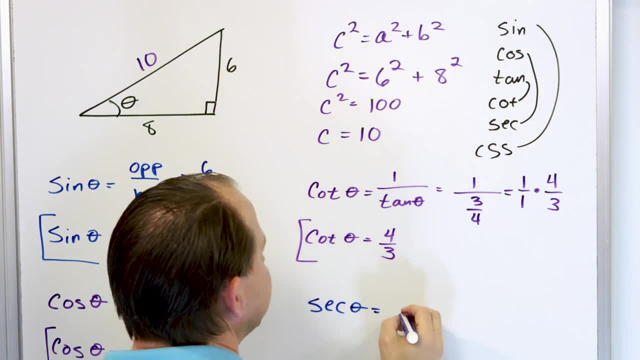 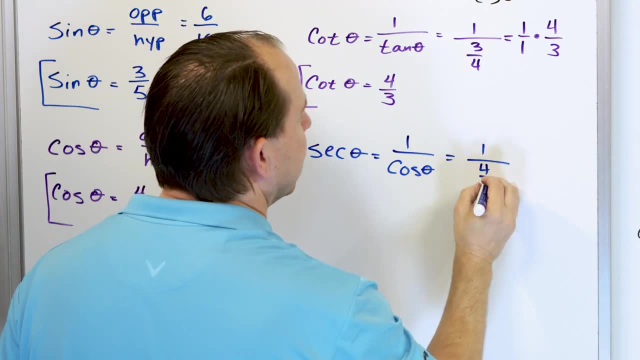 We don't need to memorize or look at that. We say: well, the secant is the 1 over the cotangent, The cosine, And that means 1 over the cosine. Cosine is 4 fifths, which means it's going to flip over. 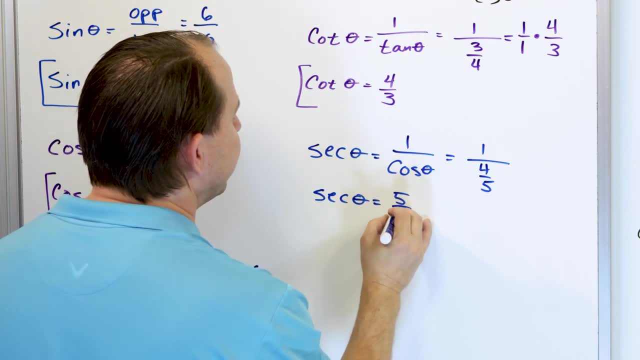 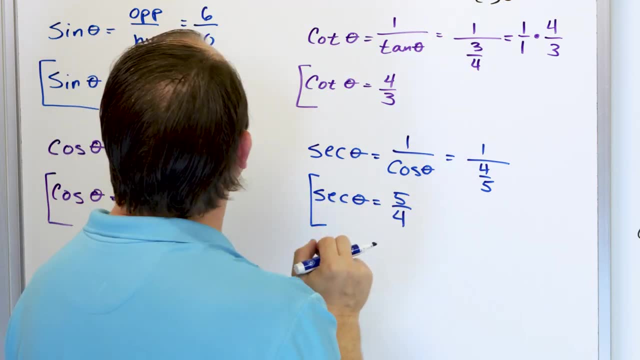 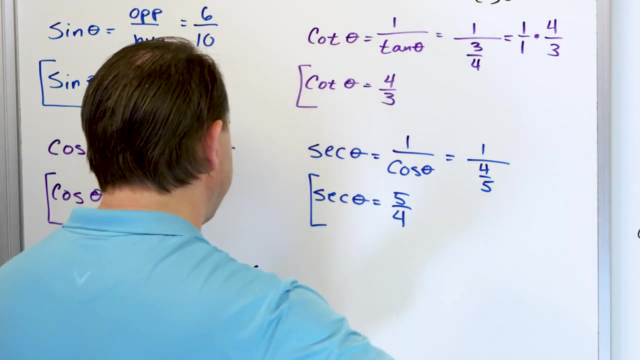 And so the secant is going to be 5 fourths Hypotenuse divided by the other side of the triangle, there, the x direction there, And then we have cosecant. Cosecant Theta Is 1 over. What is it? 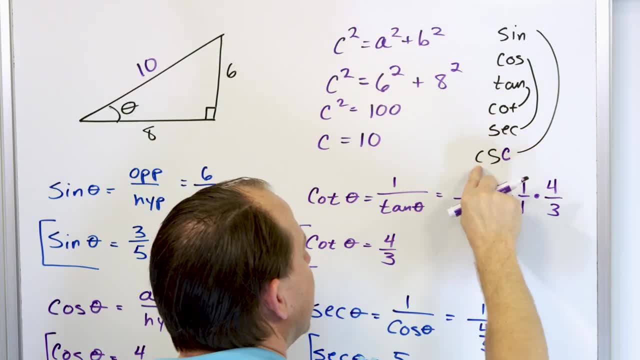 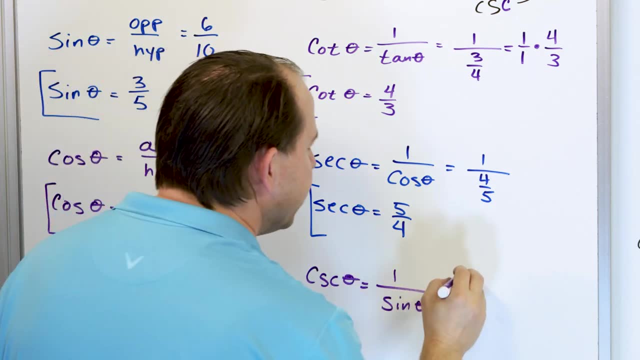 I forget. Well, let me go over here. Of course I need to write it correctly: Cosecant: 1 over sine. What did I already calculate for sine? It's 3 fifths, So it's going to be 1 over 3 fifths, which means the cosecant of this angle. 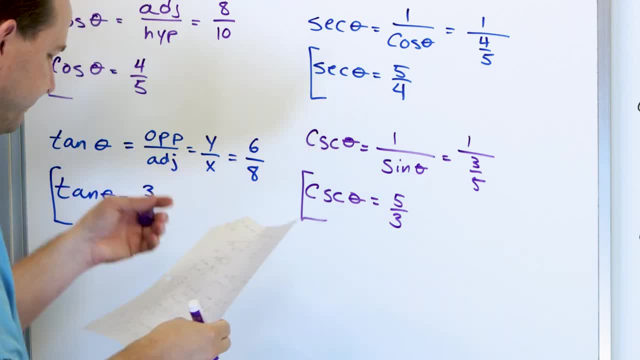 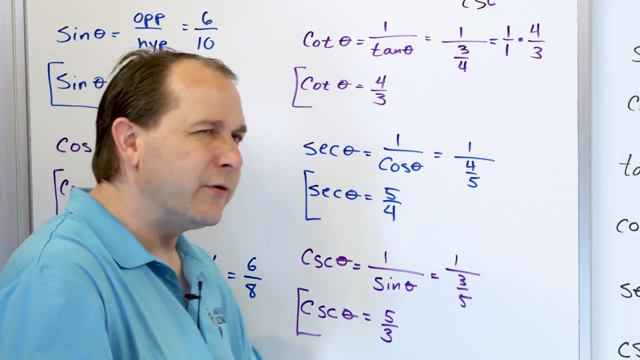 is 5 thirds, 5 thirds And the cotangent. let me just double check myself: The cotangent's 4 thirds, The secant's 5 fourths And the cosecant is 5 thirds. So if you're ever given a problem that says find the 6 trigonometric function, 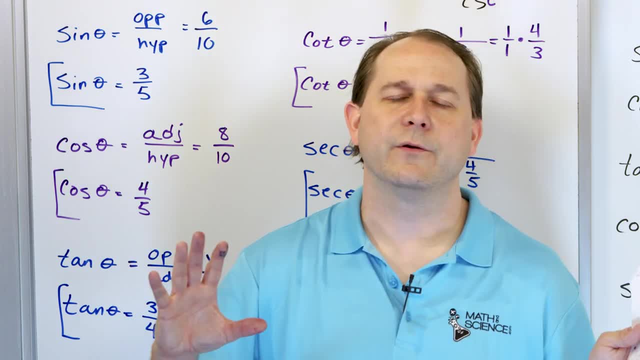 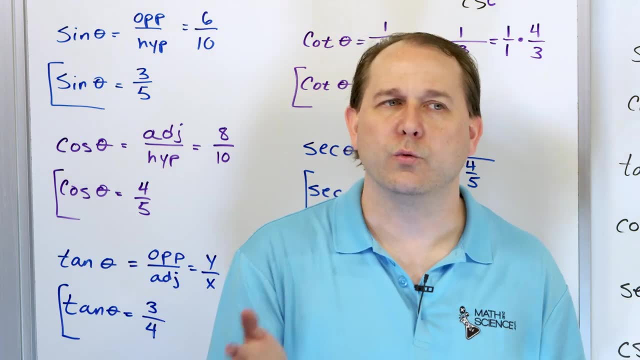 you're always going to do the same thing. You're going to write the triangle. You have to know what the hypotenuse is and the other sides of the triangle to find sine and cosine. Tangent is basically the slope: rise over, run y over x. 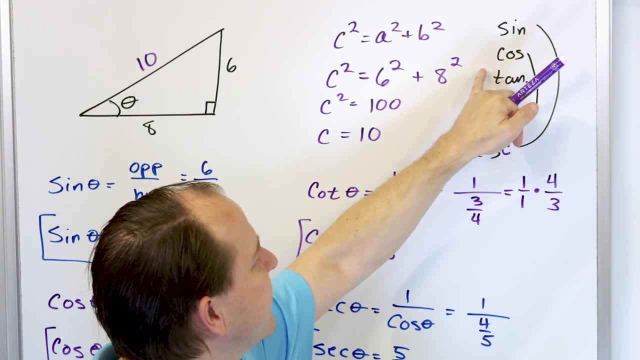 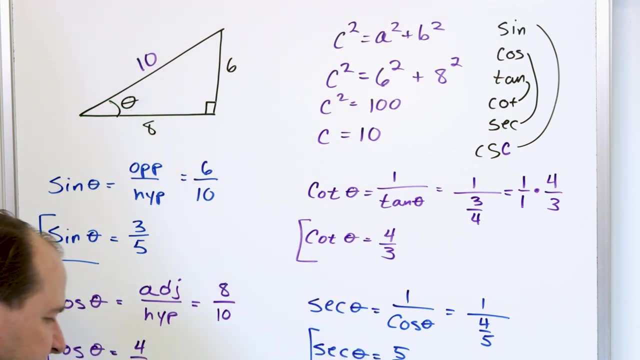 And then the remaining 3 come from this trig rainbow: The cotangent's 1 over the tangent, The secant is 1 over the cosine And the cosecant is 1 over the sine. And this is it. You would circle all of these and say these are the 6 trig functions. 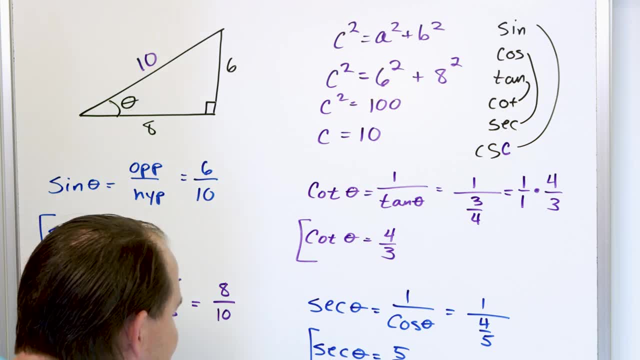 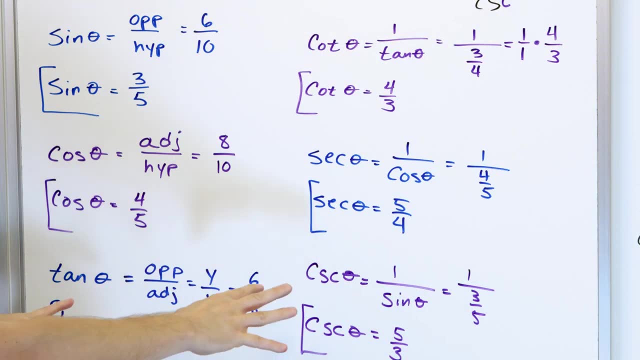 But I want to go a touch deeper, because I spent so much time in the last lesson talking about what the meaning of sine and cosine is. So now we know what the 6 trig functions are for this triangle. We also know what the 3 sides of the triangle are. 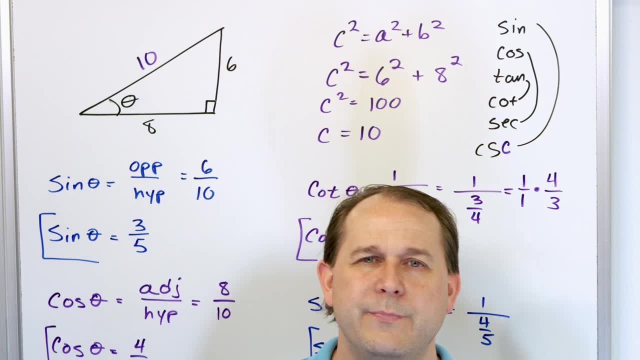 And so we can do a little bit of checking. you know, When you do basic division for the first time, you learn how to divide And then you're always taught to check yourself by like multiplying, to go backwards and multiply and figure out and make sure that you got the right answer. 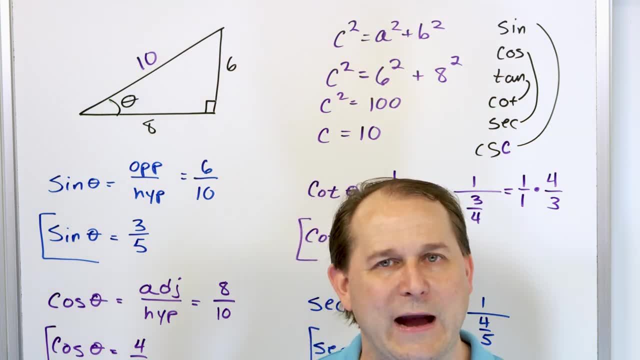 You know, when you do an equation you're always taught you get the answer for x and you plug it back in and see if you're correct. So now we have calculated the 6 trig ratios and we can use some of them to check and make sure that we're. 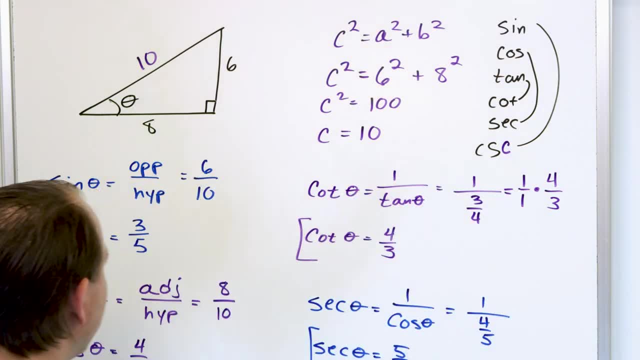 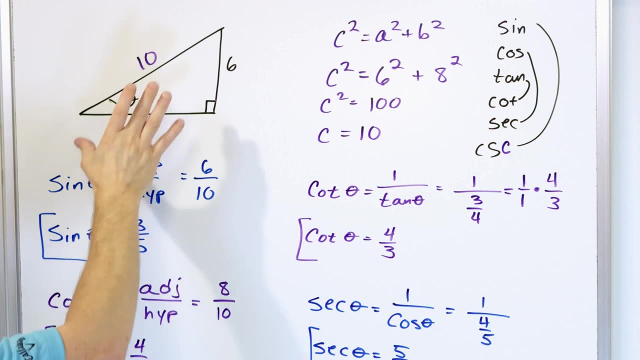 calculations were right. Remember how we're going to check. here is the following thing: The sine function is the chopping function in the y direction. It takes the hypotenuse that you have and it chops it So that it I don't have 10 anymore. 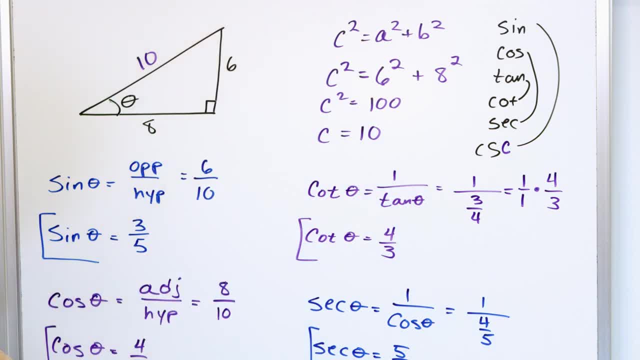 It chops it down and it should give me 6 in this direction. The cosine is the chopping factor for the x direction. I should be able to take this hypotenuse and chop it down, so it should give me the 8 back. 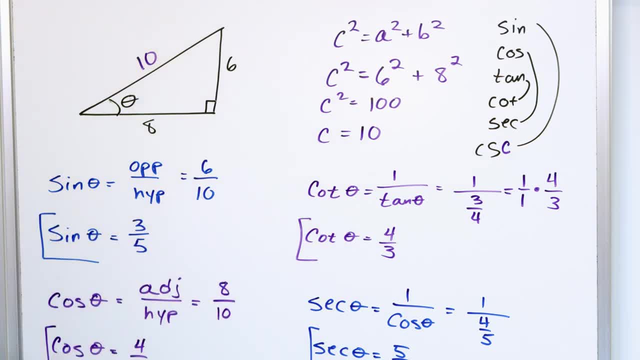 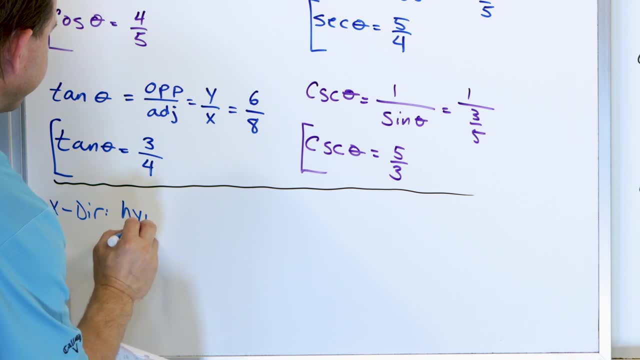 How do I check and see if this is actually happening right? So, for the x direction, what I'm basically saying is the following: If I take the hypotenuse and I multiply by the cosine of the angle, it's the hypotenuse times the chopping factor in the x direction. 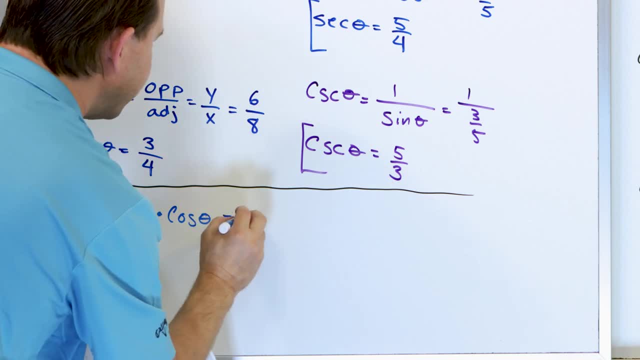 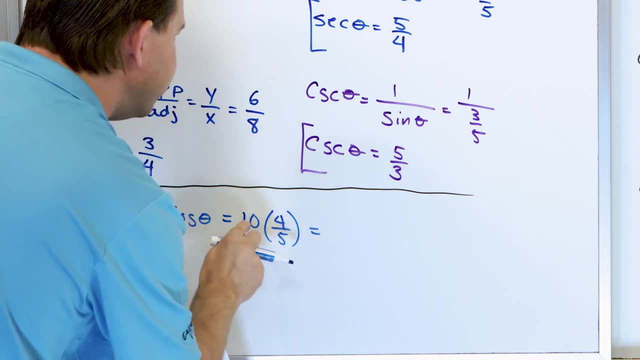 Then what I'm going to get? the hypotenuse was 10.. What is the cosine Go over here? the cosine is 4 fifths. So when I multiply this, what do I get? Multiply the tops, I get 40.. 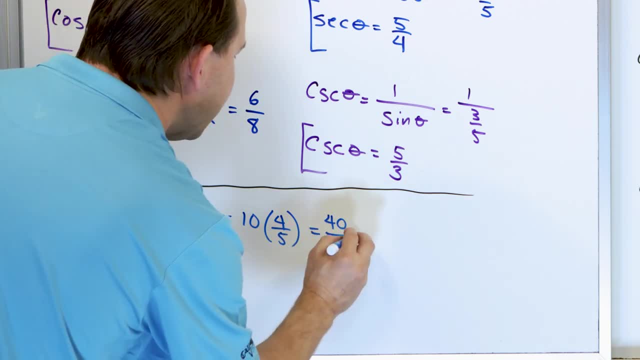 Multiply the bottom 5 times 1 is 5.. And what do I get? 40 divided by 5, that's 8.. So you see what's happening. The x direction when I take the hypotenuse and I chop it in the x direction. 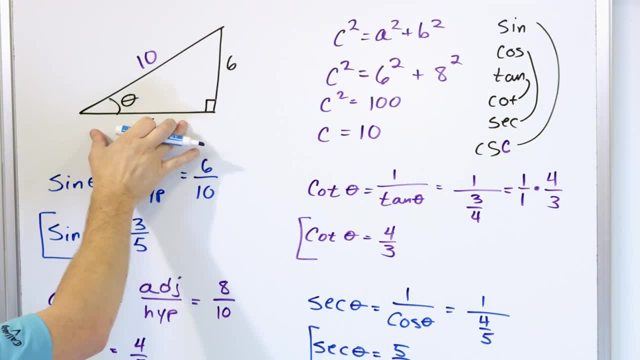 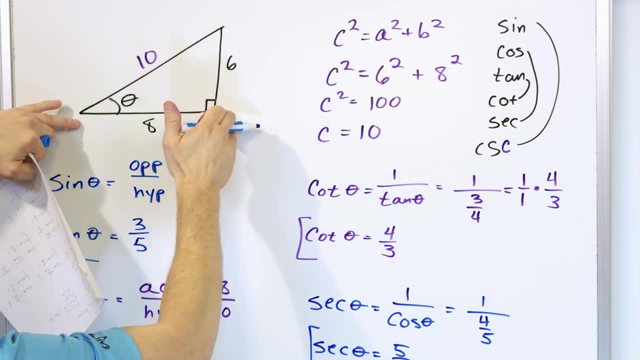 I get an answer of 8, which is exactly what my triangle is. The cosine function: when you multiply it times the hypotenuse chops it down and it kind of cuts it so that it gives you the x portion of that triangle. 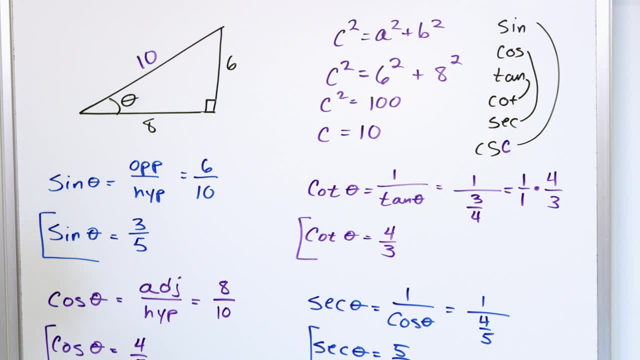 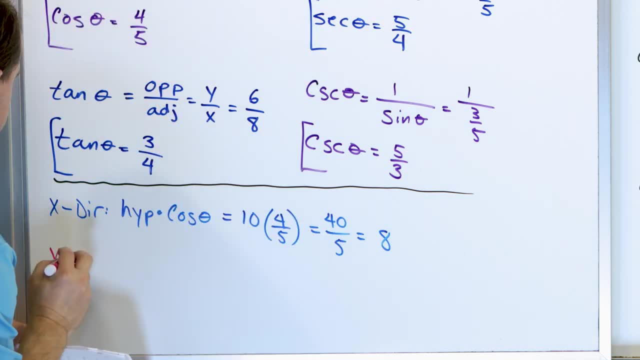 the portion that lies along the x axis that chops it in the x direction. What do you think is going to happen when we do the exact same thing for the y direction? If I take the hypotenuse and I multiply by the sine of the angle, 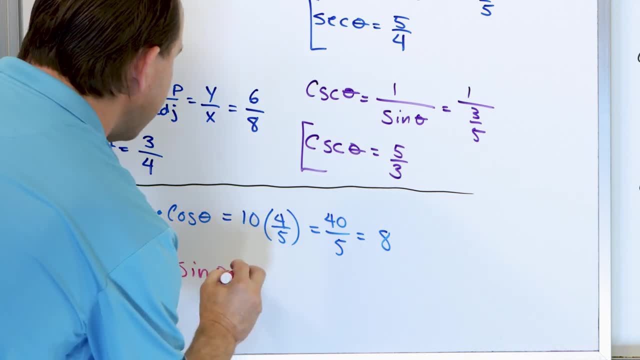 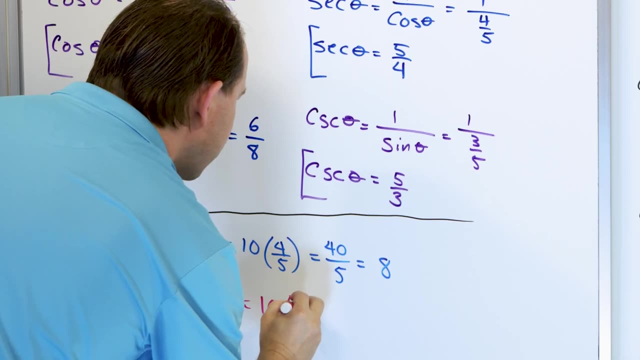 it means I'm multiplying by the chopping factor in the y direction. The hypotenuse never changed, it's still 10, but the sine is the chopping factor in the y direction. it was 3 fifths. So multiply by 3 fifths, what do I get? 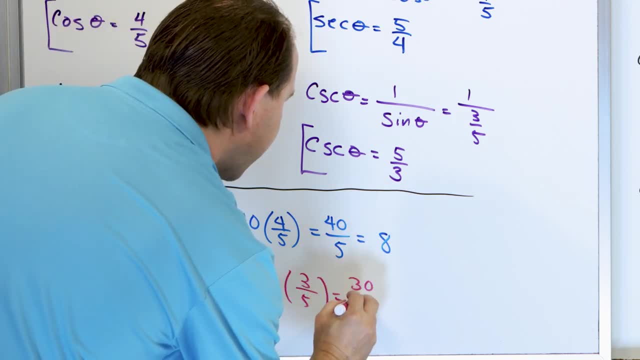 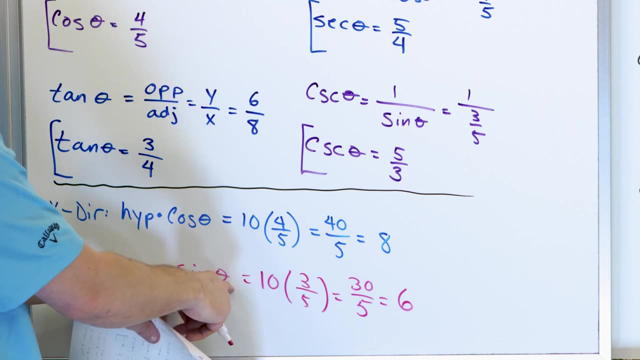 I'm going to get on the top 30, on the bottom 5, and I divide those and I get 6.. So when I take the hypotenuse and I'm multiplying by the chopping factor in the y direction, I get an answer of 6,. 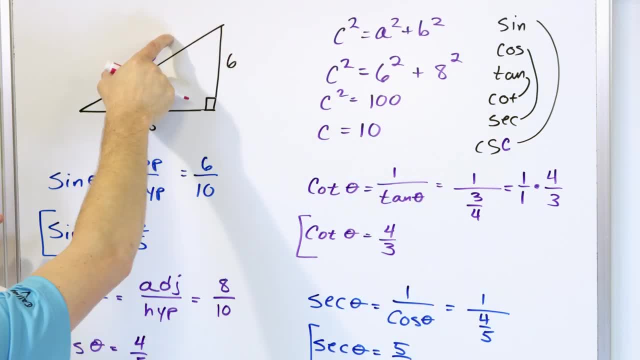 which is the side of the triangle here. So when you take any hypotenuse and multiply by the sine of the angle, it takes the hypotenuse and it chops it and gives you this side of the triangle. When you take the hypotenuse and you multiply by the cosine of the angle, 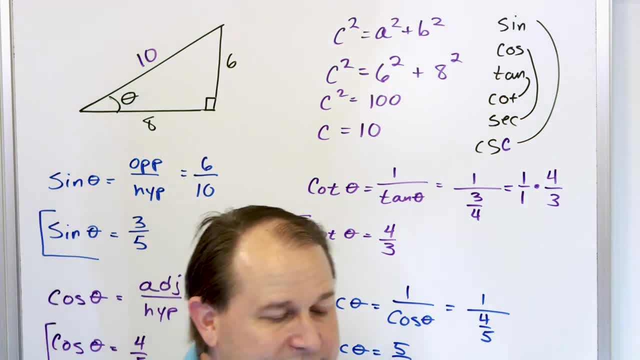 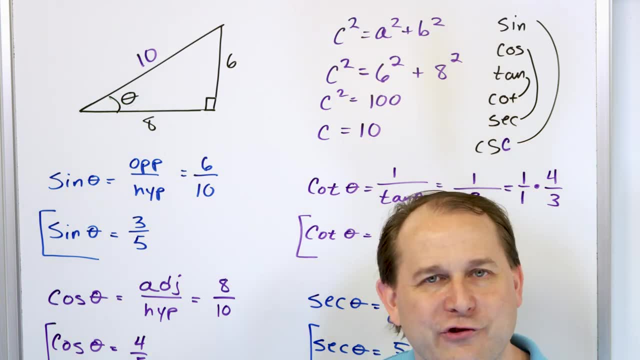 it chops it down and it gives you this side of the triangle And that is why, since the very beginning, I've been telling you about this whole chopping thing, because it comes up over and over again. You can use it to check your triangles. 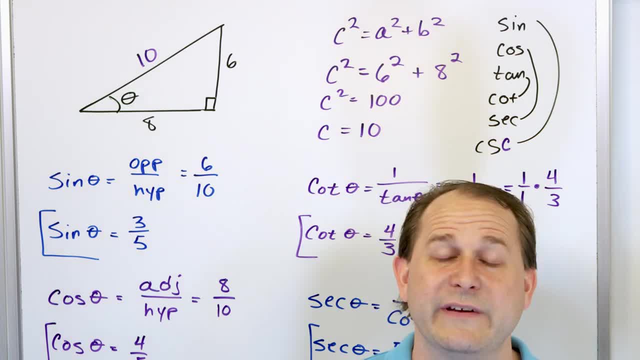 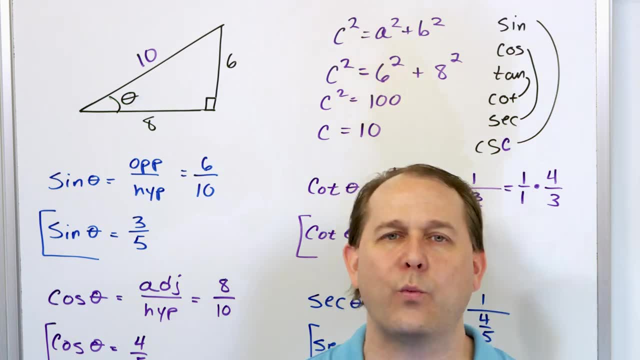 as you go along throughout these basic problems, but we also use it extensively later in something called vectors. We're going to learn about vectors later in this class And then when you go on into math and engineering, you can't get away from vectors. 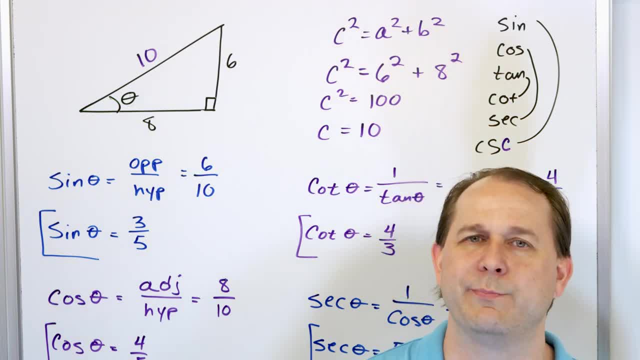 We use them for everything from space probes to building bridges, to building electronics. I mean, everything uses a vector, And so the idea of taking a hypotenuse and chopping it in the x direction, chopping it in the y direction, that is critically important to understanding this thing called a vector later. 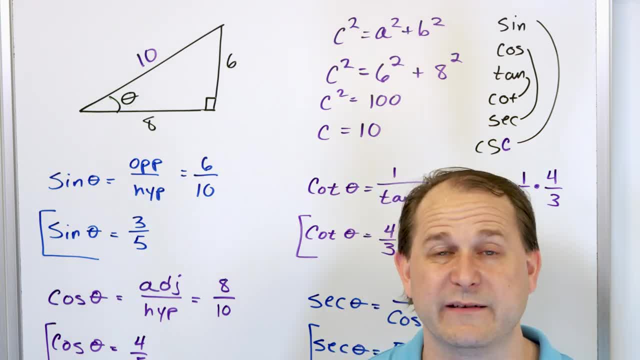 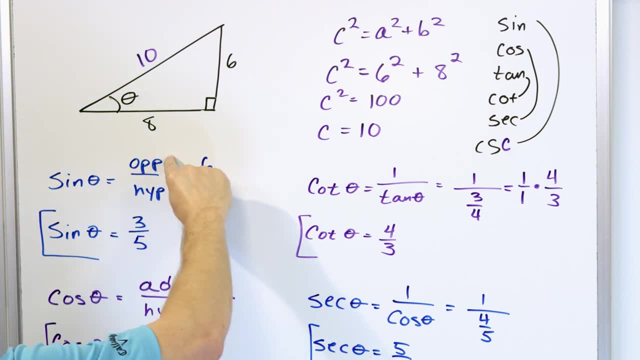 So I'm kind of teaching you some of that as we go in the beginning, because it is very important. All right, Now, why does this chopping thing work? Well, it's because the sine is defined to be the opposite over the hypotenuse. 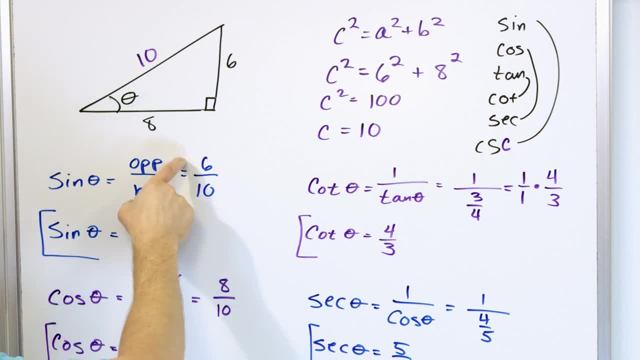 So, of course, if I multiply this by the hypotenuse, the hypotenuse will cancel and I'll be left with the opposite side. That's exactly what I was left with. If I take a cosine, it's defined to be the adjacent over the hypotenuse. 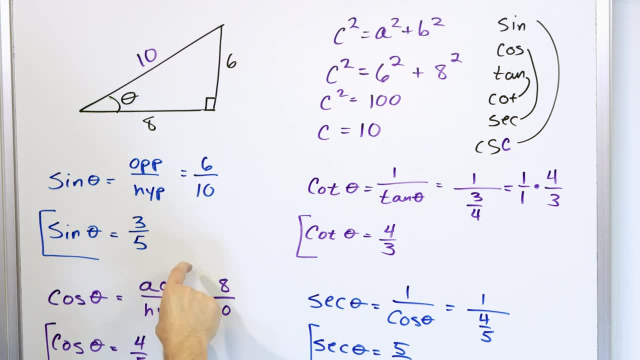 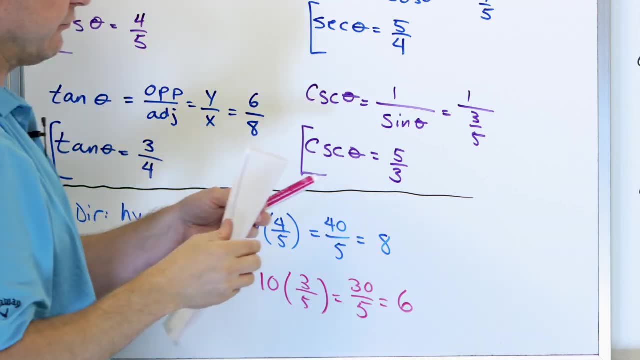 If I multiply this by a hypotenuse, this is a chopping factor multiplied by the hypotenuse. the hypotenuse is canceled and I'm left with the adjacent side, which is exactly what the 8 was: the adjacent side of this triangle. 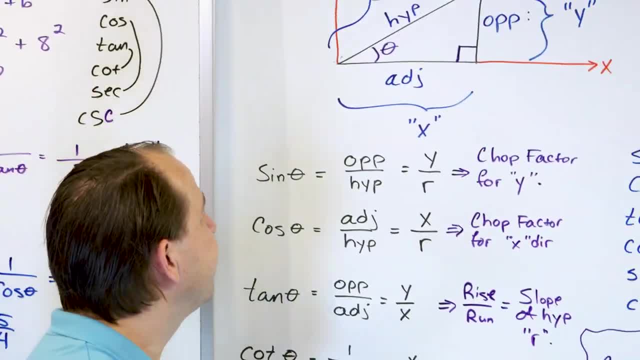 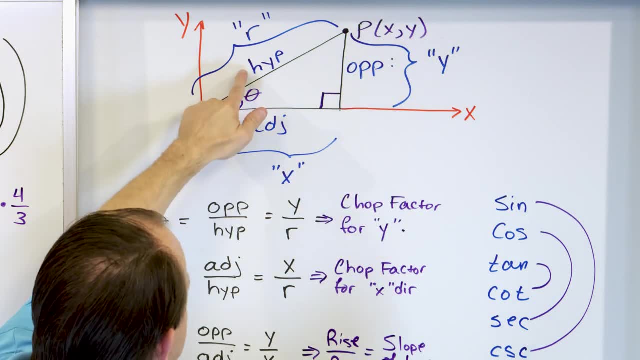 So we've learned a lot in this lesson. We have introduced the concept of a reference triangle like that: We have an adjacent side, an opposite side, which are x and y directions. We have a hypotenuse, we call that r.